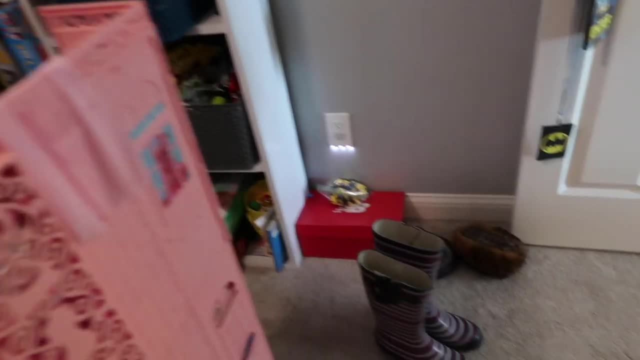 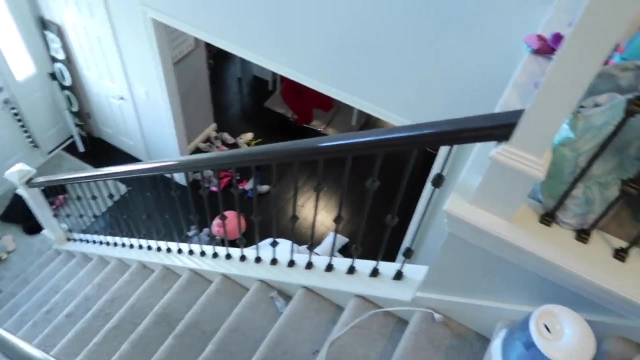 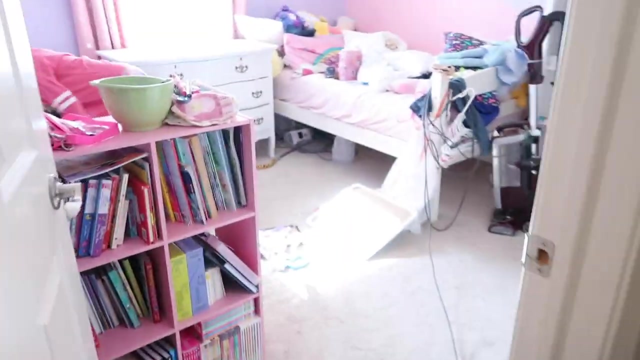 the best. so his room is packed to the brim because pulling everything out, and then the girls are pulling everything off their bed and throwing it down so that we can, so we can get it, so that it can all get wash, and then some of this is really organized like the books stay okay, and so I'm just gonna go through. 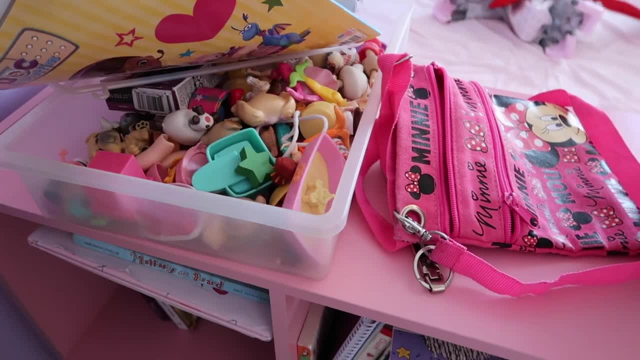 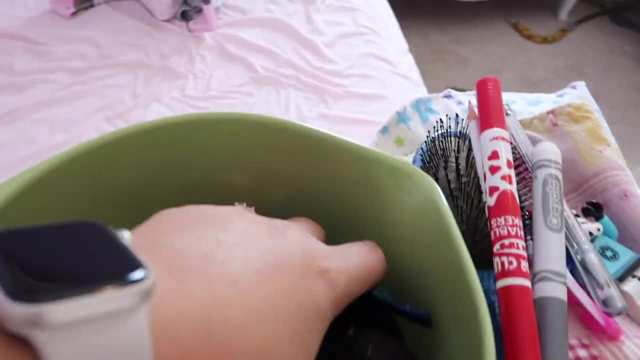 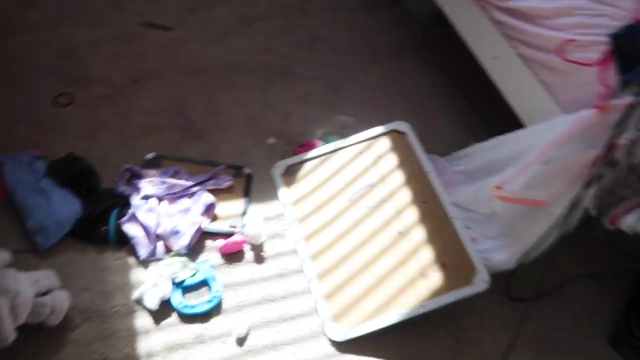 those, see if we can get rid of any. this is like LOL doll, I think, or something. I don't know. I'd have to look what they are. this is all the hair stuff that we have found in beds, under beds, all that kind of stuff, and then we're stripping the bedding to get that all washed. 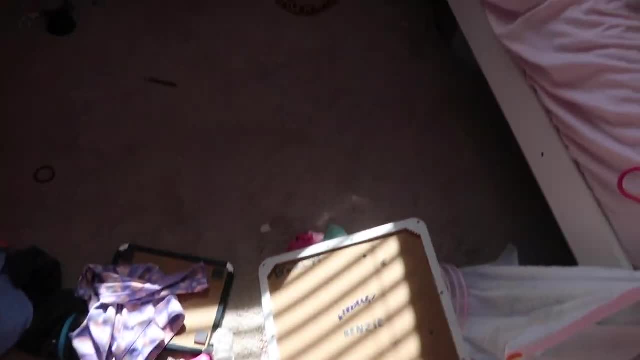 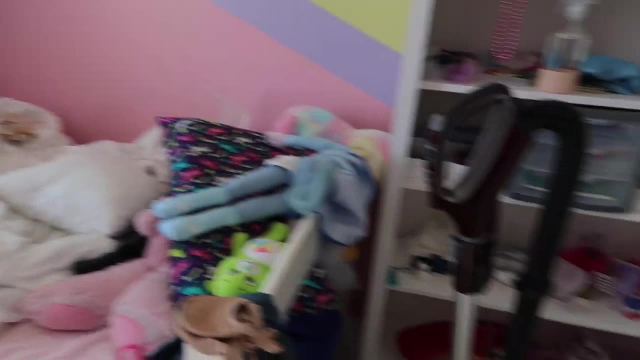 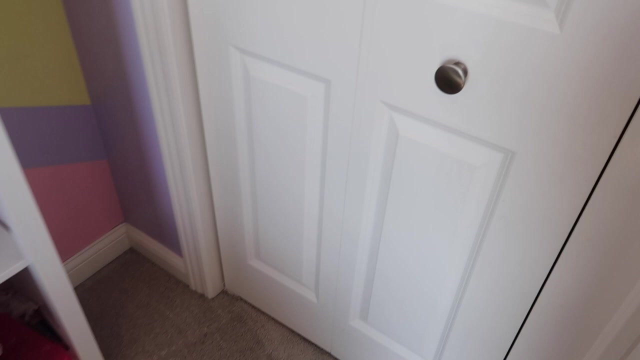 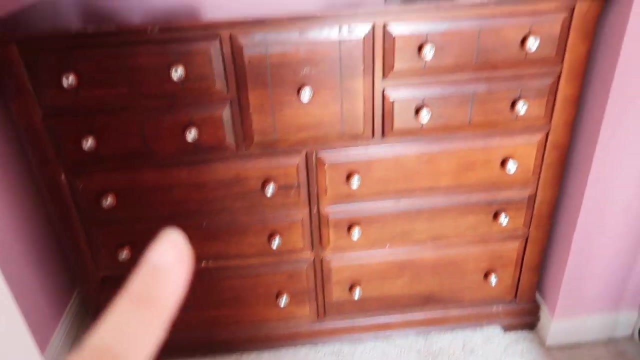 this was stuff that was like underneath the bed and such um. this dresser, I think, is going to go over to Beckett's room, and then we need to do something with this bookcase, because it's just not being utilized to its full extent. and then Lexi is in the closet. um, they have this really. 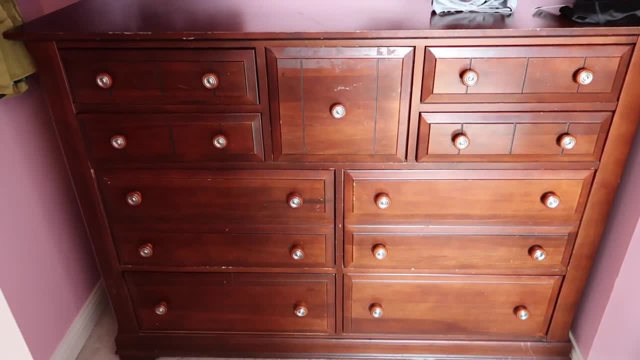 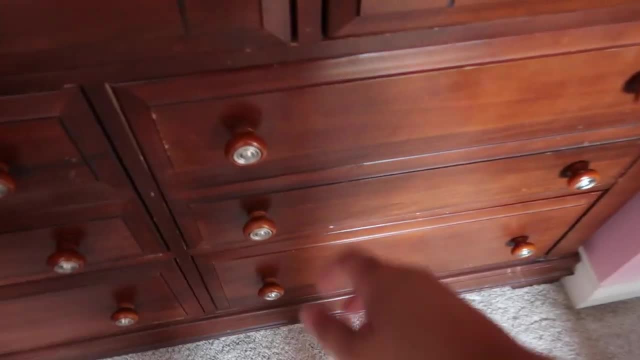 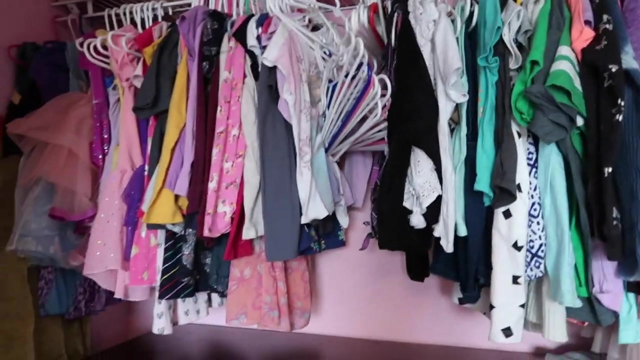 nice dresser that we actually found. our neighborhood pulls a whole bunch of stuff out to trash and it's usually really nice stuff, and so, if you could see, these are double drawers, they're really really deep and so they hold a lot, and then the girls share this closet, so this half 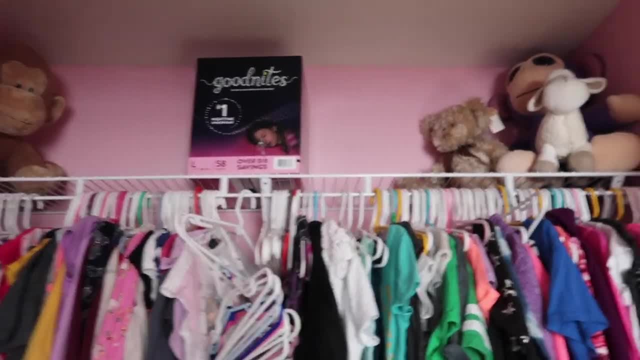 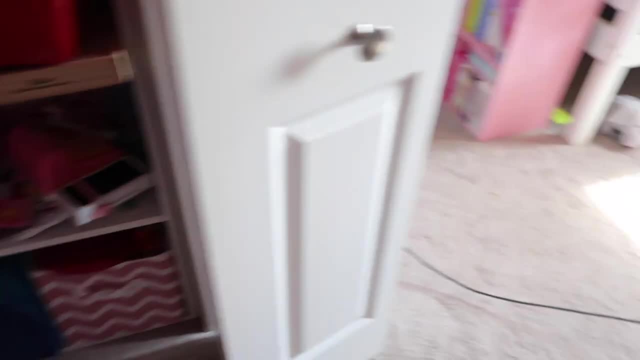 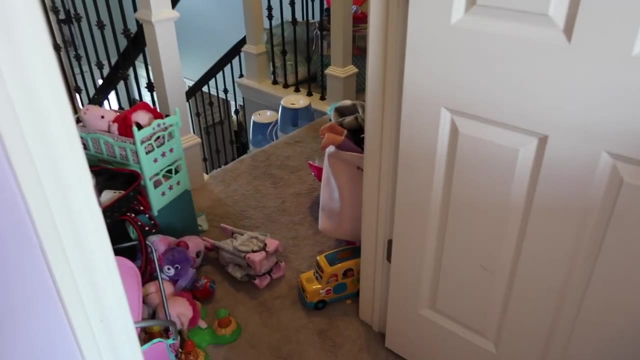 is Kenzie's and that half is Brooklyn's, and then just extra storage up there. these are mostly games or craft items, so I'm gonna leave them up there so we can go through them that way. but other than that, we're trying to pull everything out of this room so that we can just like start completely fresh. 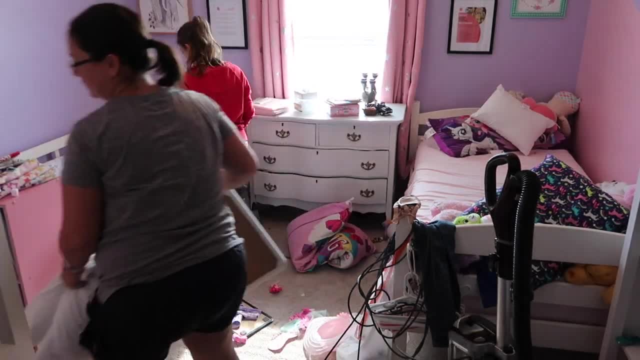 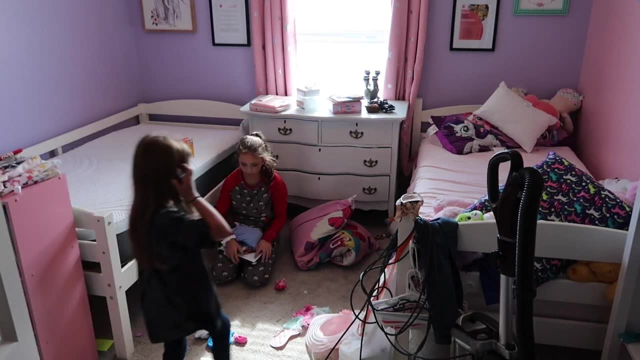 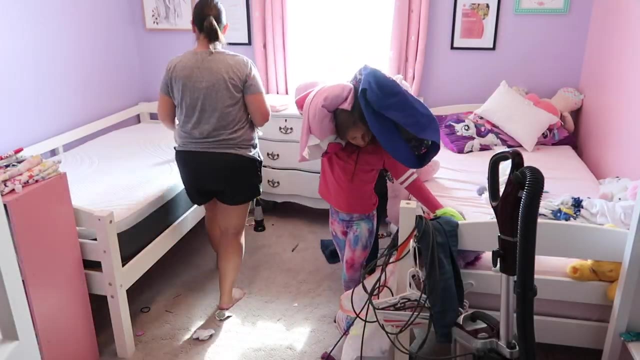 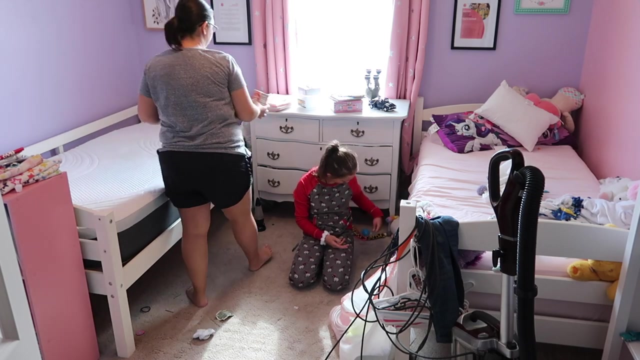 you're my best friend, didn't care about the rules. good, on the weekends I'll be in fools drifting the deep space- so brave and so stupid, just like the movies. how it's gonna stay in the fight with you just thinking we would do this until we couldn't do. 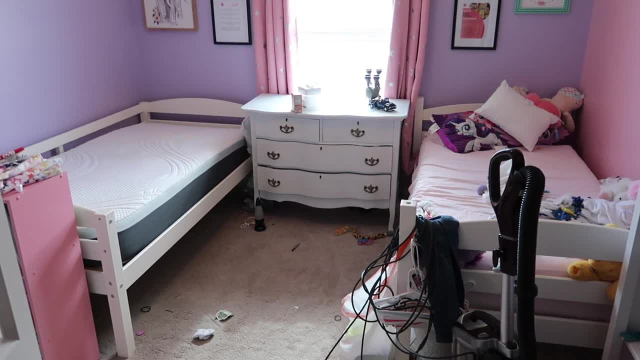 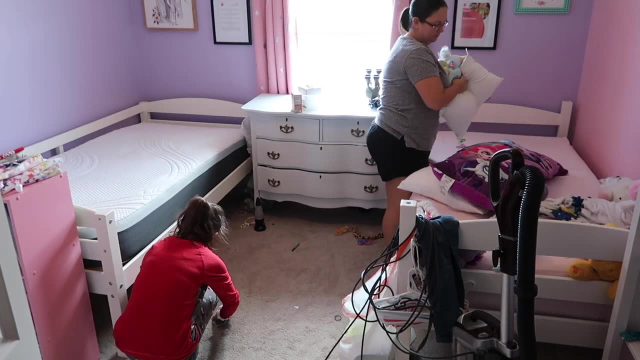 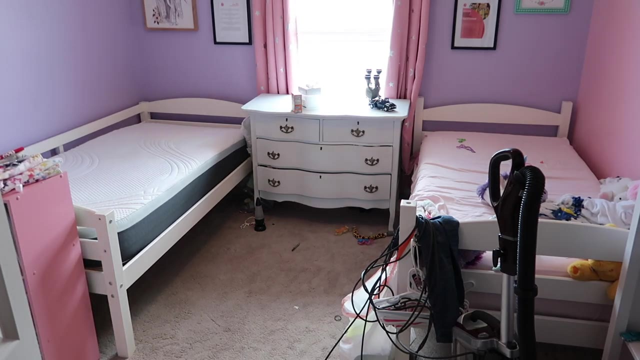 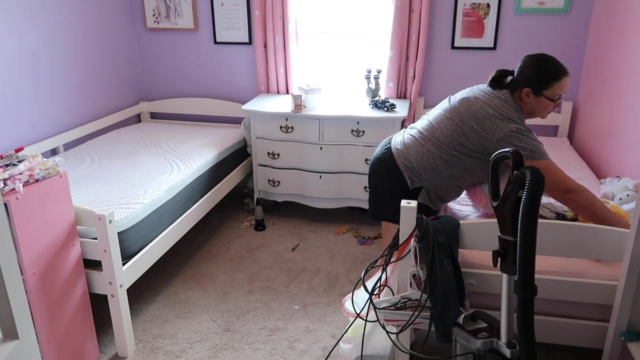 it each and every high, every night with you, you and me. so clueless, we were just broken, shattered, singing along to nothing matters stray around like nighttime rumors. we were in too deep and you worn our sweaters, thinking we'll be young forever, driving in your mom's old hatchback. 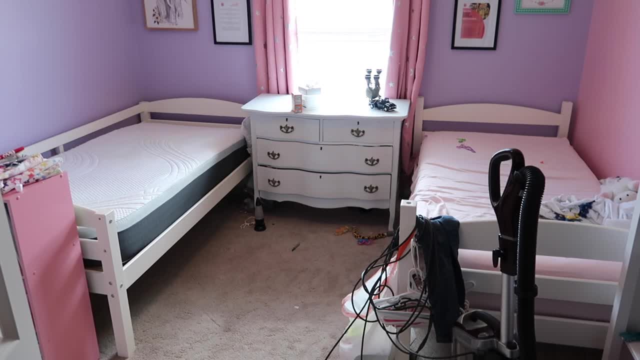 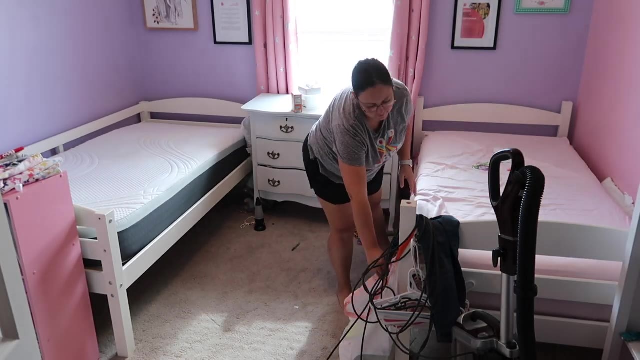 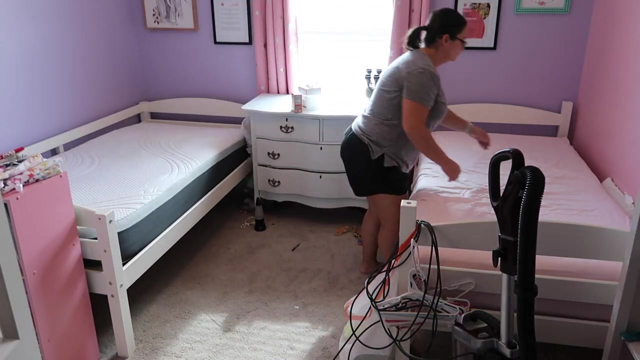 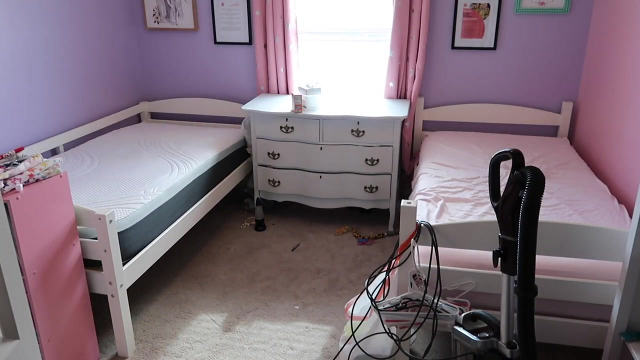 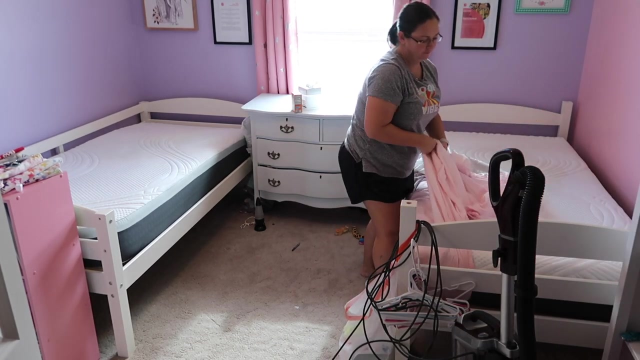 and we were in too deep. cause I'm thinking we'll be young forever, we're young forever. cause I'm thinking we'll be young forever, we're young forever. we're young forever. cause I'm thinking we'll be young forever, we're young forever, we're young forever. 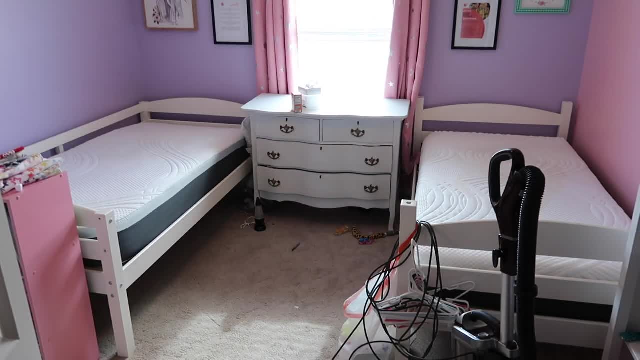 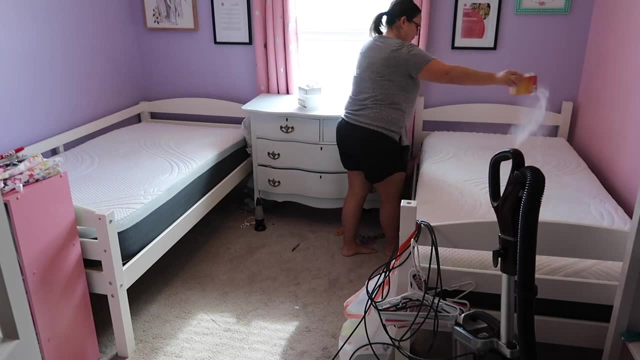 cause I'm thinking we'll be young forever. where did it begin? where did it end? hanging on those strings unable to bend? I never listened. trying to prove it, just like the movies- how it's gonna stay in the fight with you, just thinking we would do this until we couldn't. 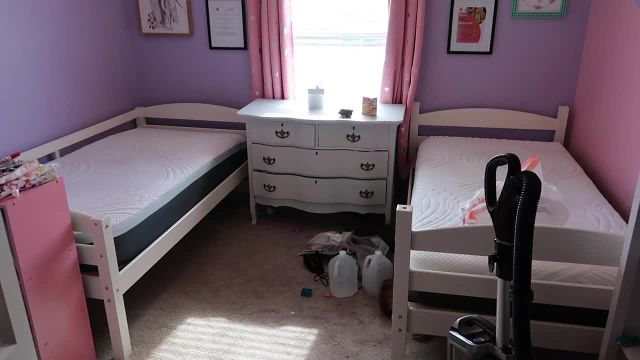 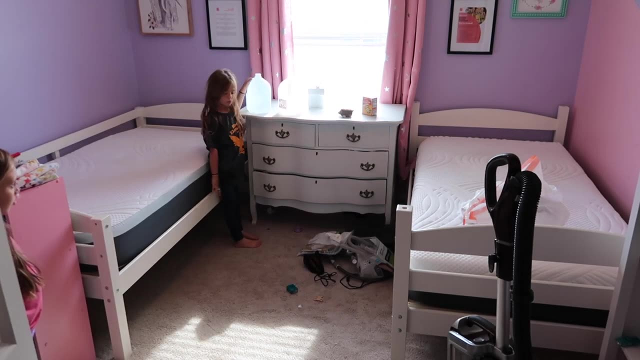 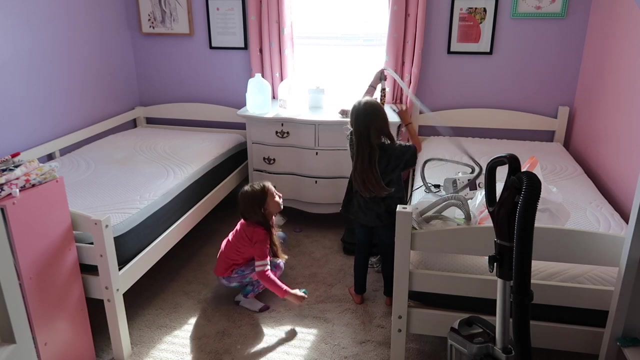 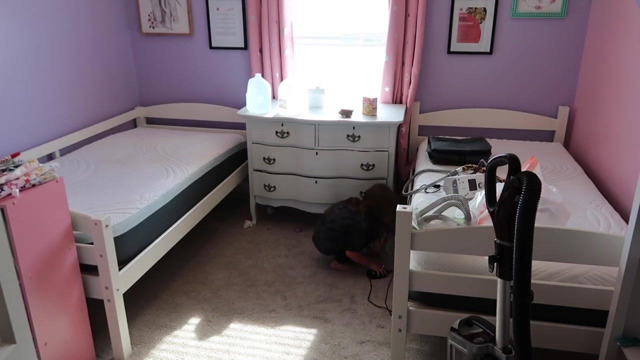 do it each and every day, just like the movies Couldn't do it each and every high every night with you, You and me. so clueless, We were just broken, shattered, Singing along to nothing matters, Stray around like nighttime rumors. We were in too deep. 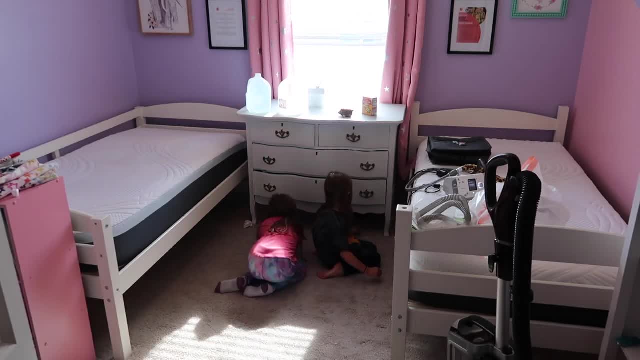 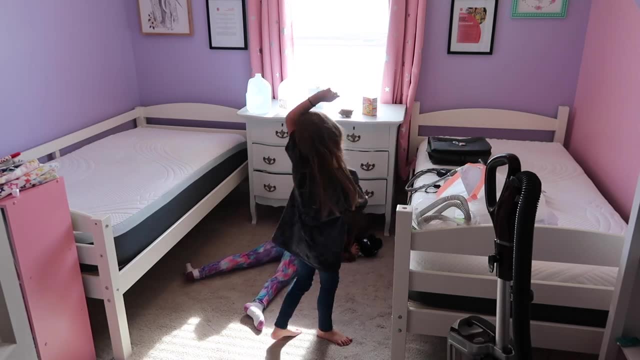 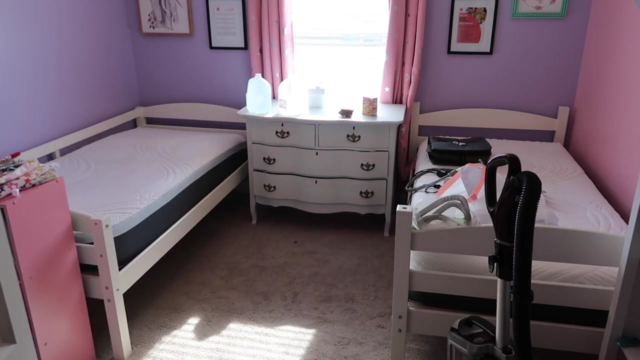 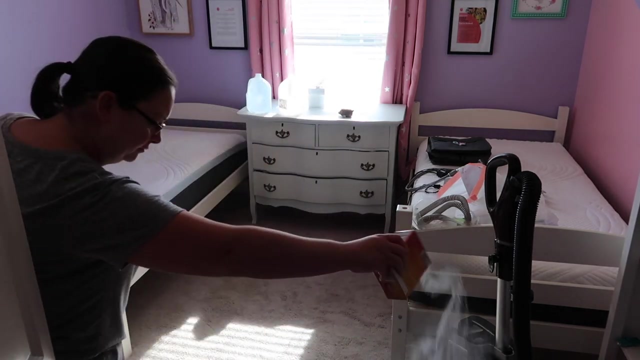 In your worn out sweaters, Thinking we'll be young forever, Driving in your mom's old hatchback And we were in too deep. Cause I'm thinking we'll be young forever. We're young. we're young Cause I'm thinking we'll be young forever. Cause I'm thinking we'll be young forever. We're young. we're young Cause I'm thinking we'll be young forever. You watch me under the light, So keep me in your sight, Cause I can do this all night. You can call me up at night. 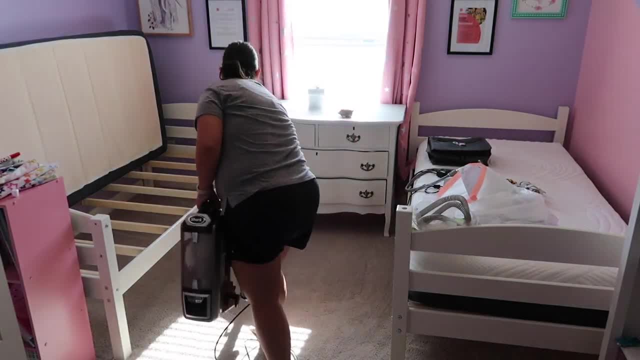 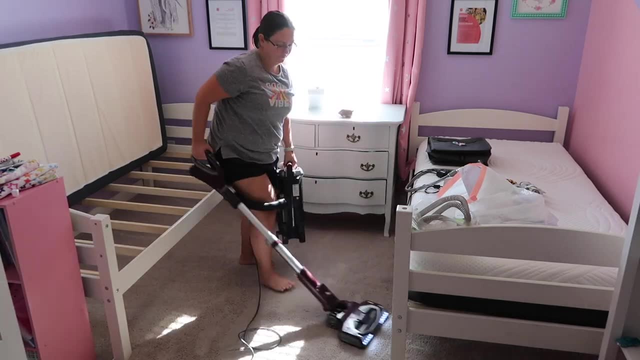 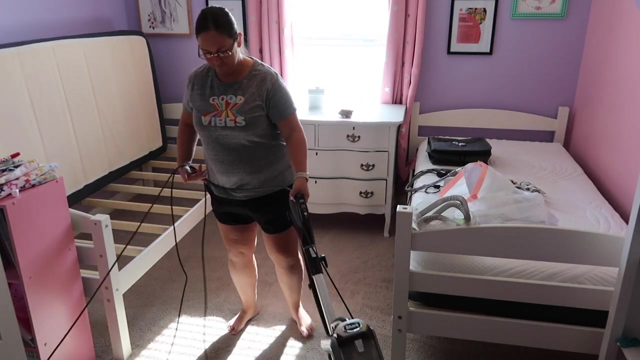 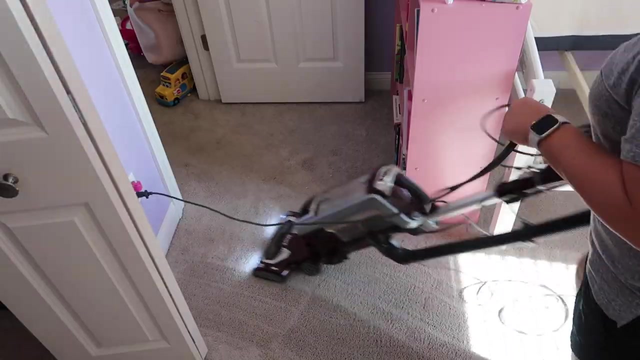 Call me what you want. I got something else in mind. Oh, if it's you I've been waiting for I better make you worth my time. So don't you pay them any mind. Close your eyes, follow the sound, Keep it coming through the night. We don't need to slow down. 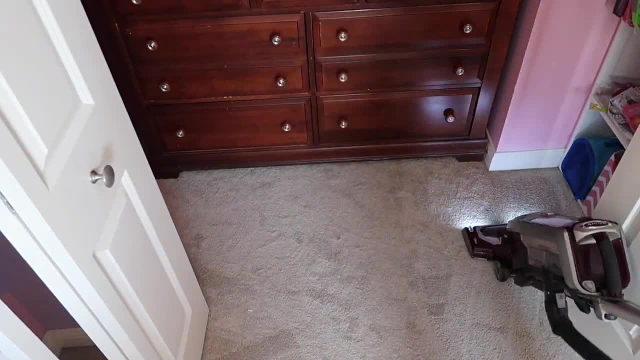 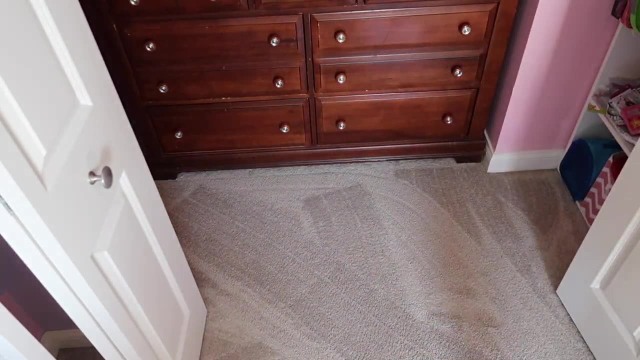 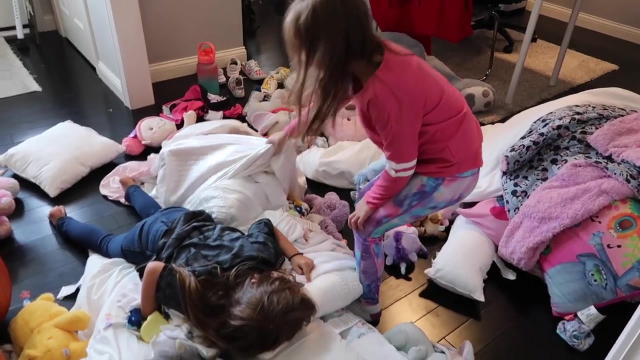 Take it all. I'll give you what you need. If you're sleeping, I love you in the dark, So shine on. I'll lose you. smile on, Show me what you're hiding with What you call me. I'm not holding a pencil, All right, so the pumpkins are in here. 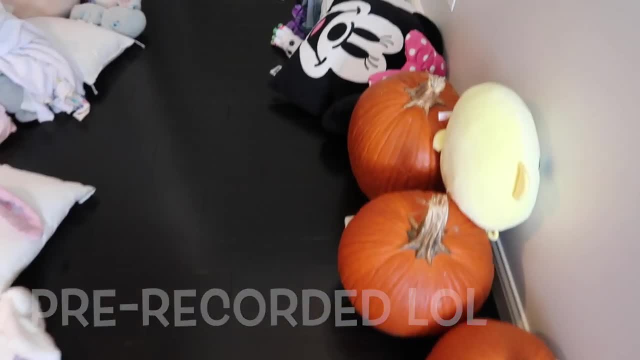 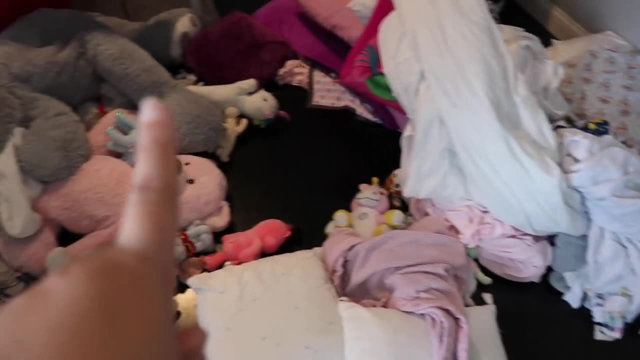 so they can get nice and warm. so when we cut them we're not freezing our fingers off. We have some dirty clothes over here. a couple pillows, more pillows- this is bedding and pillows- and then stuffed animals. So they know they need to be sifting through this. 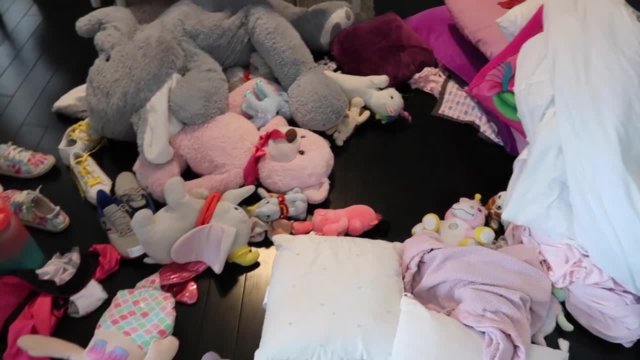 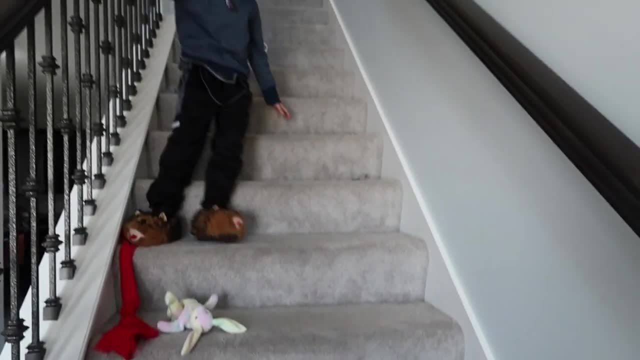 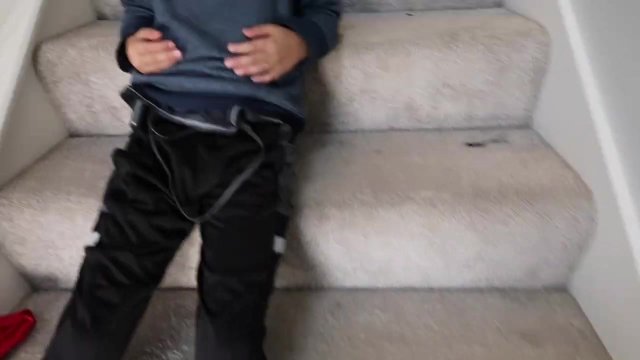 She's already picked out that one that we can get rid of, but we're going to be getting rid of more. And then da, da, da, Oh my gosh, so dirty up there. They're all running out of so, am I? 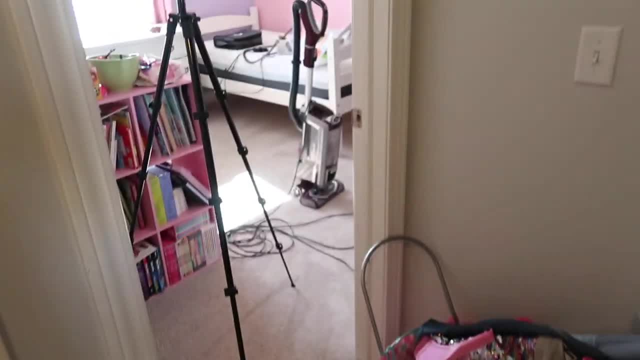 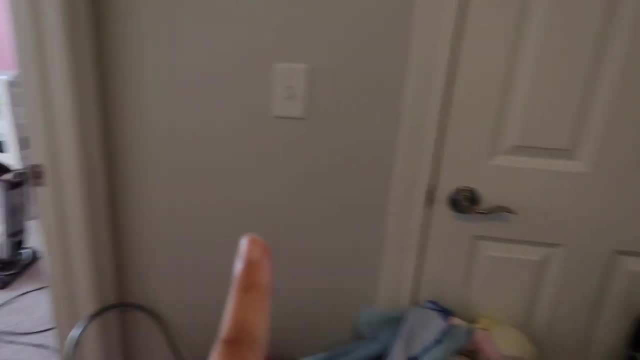 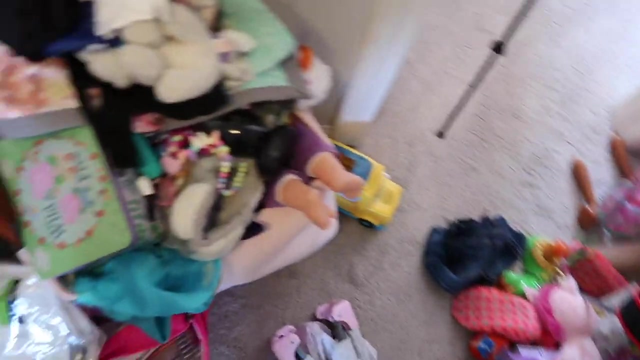 All right, so what we do need to do, so all that's cleared and vacuumed in there, All this stuff, because this white dresser that's over here is going to be going into his room. So all this stuff right here, we need to somehow or another. 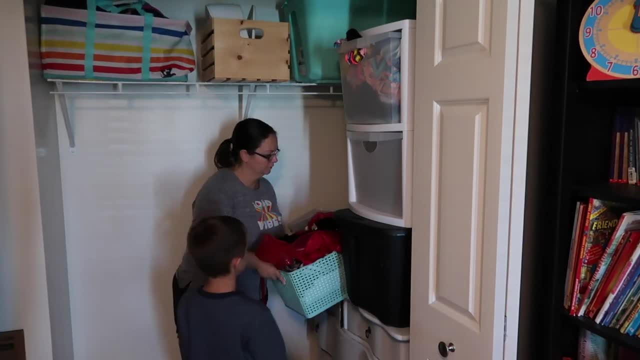 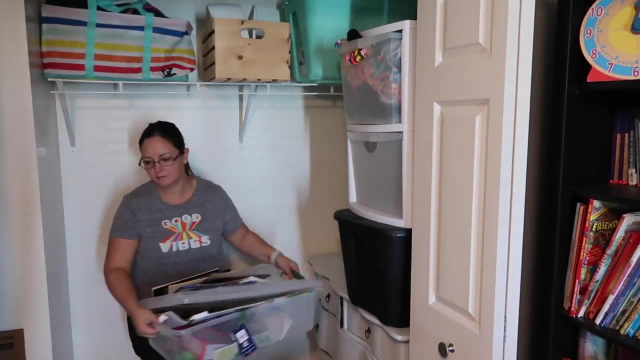 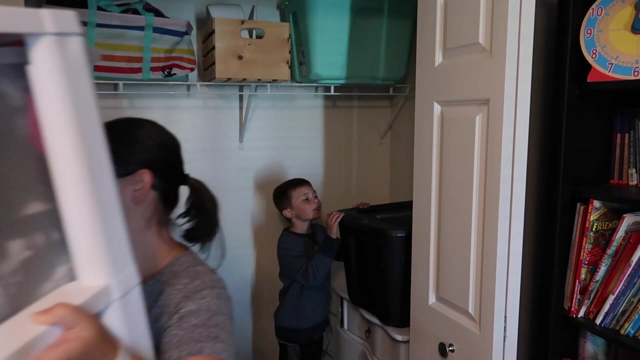 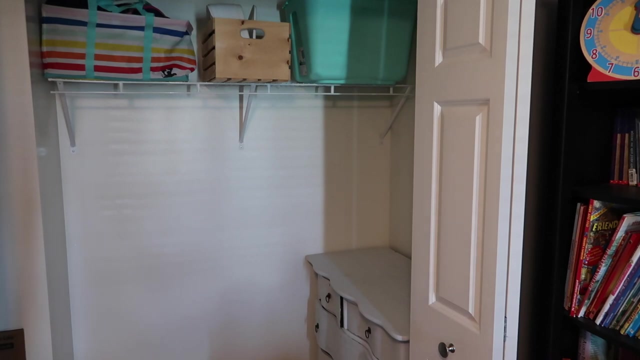 find room over here for it. You look at me like I'm crazy when I shut my feelings out. You look at me like I'm different. Still, you stay because you feel something real. Get so lost in my moments Doesn't mean I don't need you. 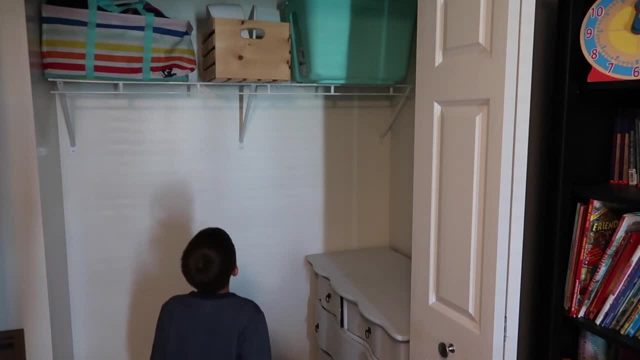 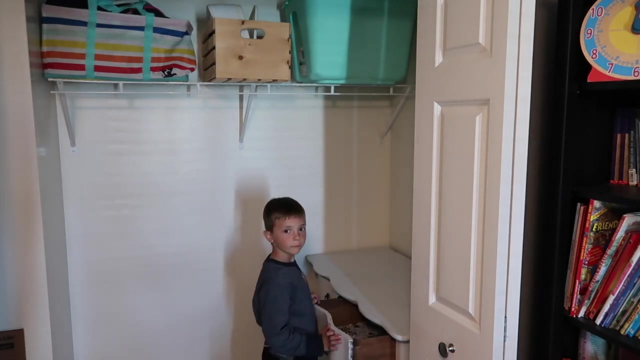 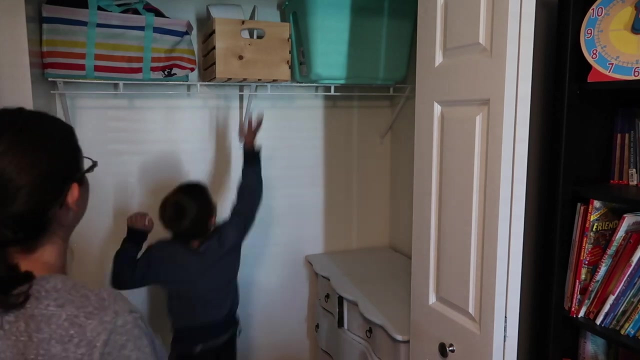 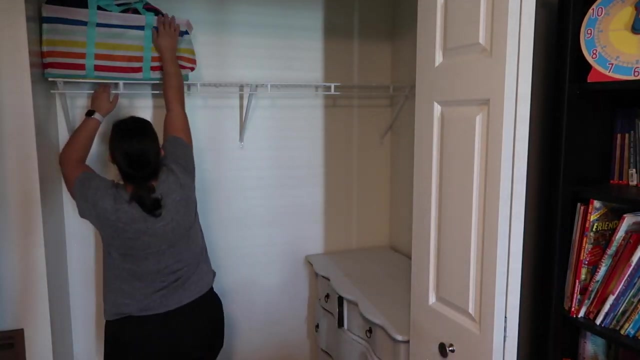 I, I, I fell in love with your colors. They kind of tell me what I'm thinking. I fell in love with the way we are and the way we lose it. there's something different about us and the reason why we stay. we fly around like paper planes. they never know where we will fall. nobody can see us. 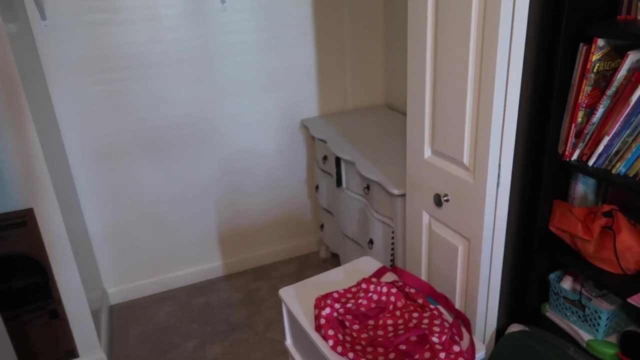 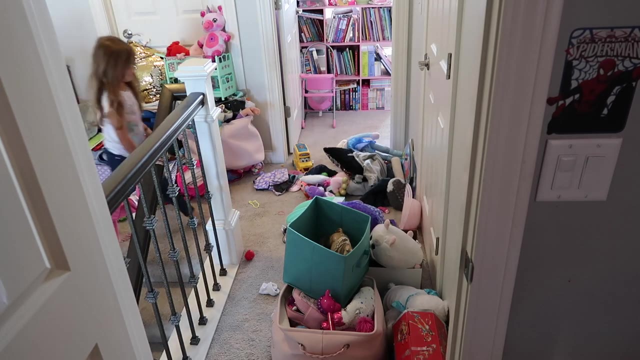 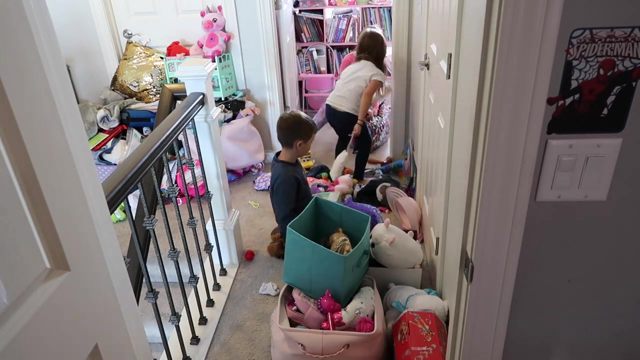 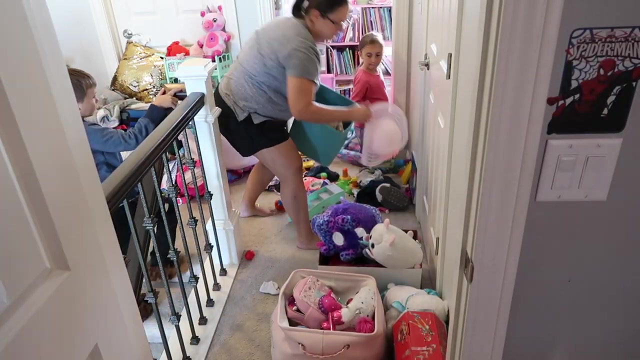 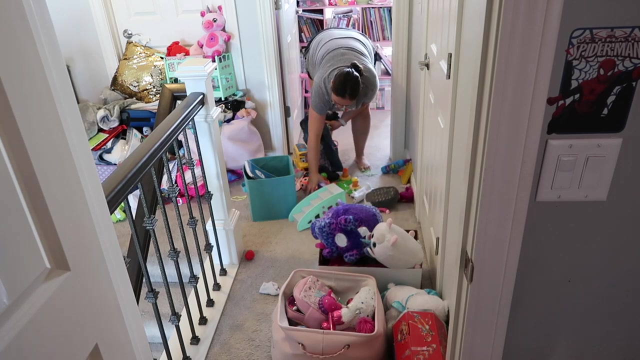 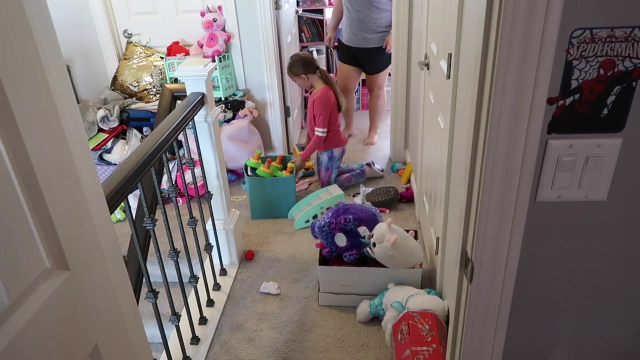 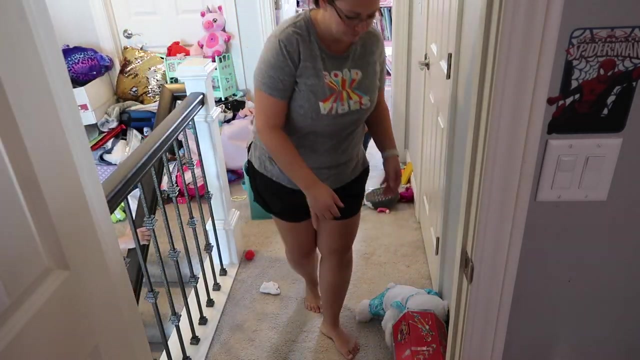 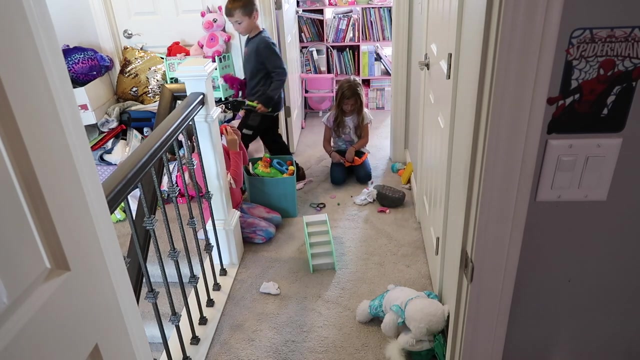 still, they wanna tear us apart. there's something different about the way we are. there's something different about us. there's something different about us. we're pouring cup after cup after cup. yeah, it's just the way we do it. anything just to block out the real life? real life: yeah, we're loving the way they. 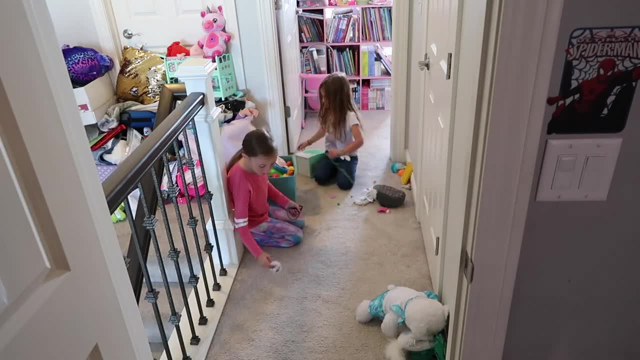 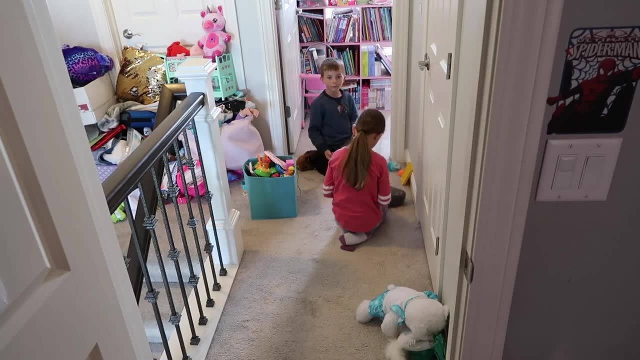 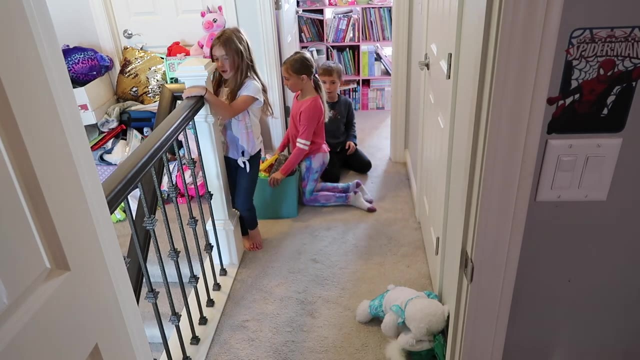 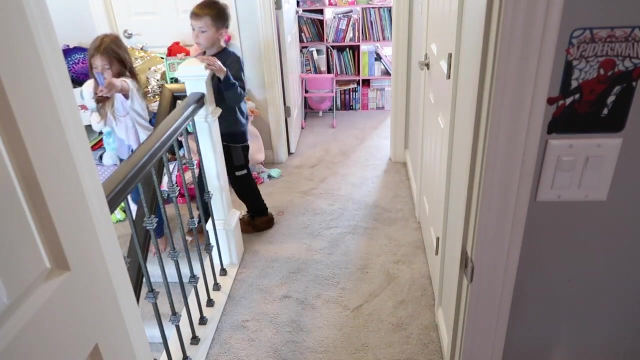 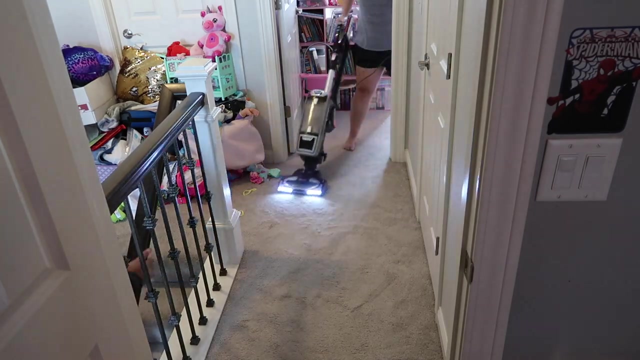 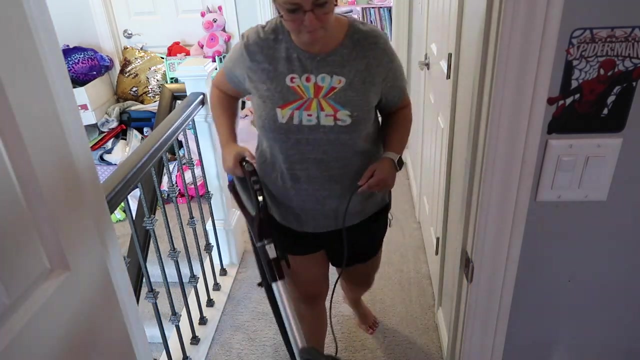 think we're so messed up, even if what we're doing is bad. there's so many emotions sharing so much is that we never had the end of israel. i think we're searching for reasons not to be like them. we fly around like paper planes. they never know where we will fall. nobody can see us. still they. 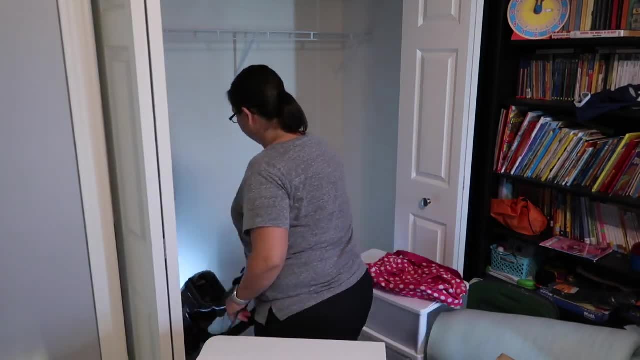 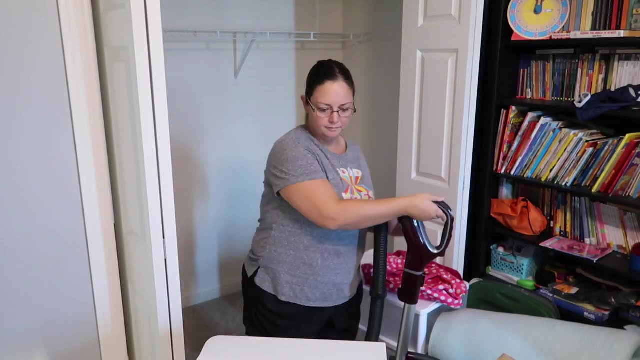 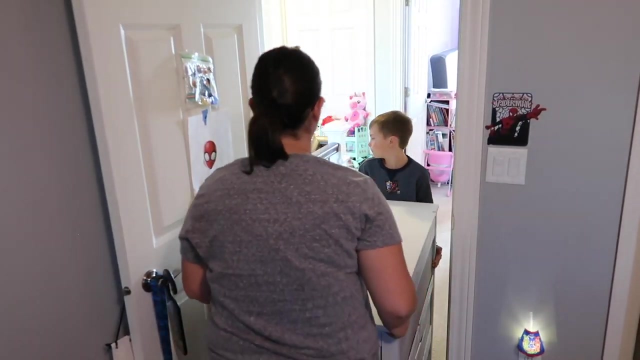 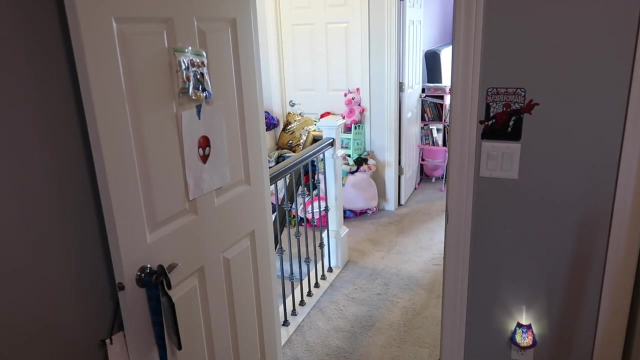 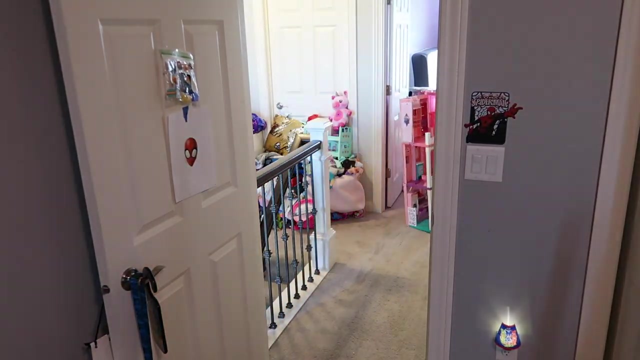 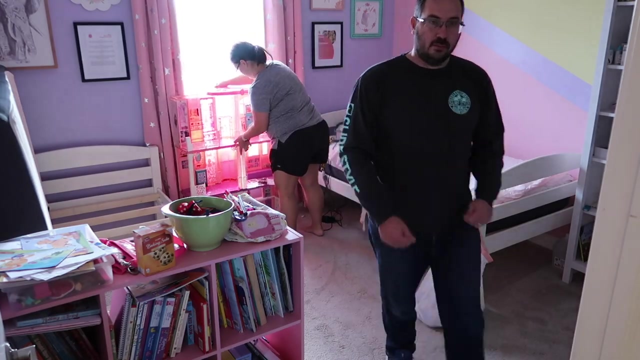 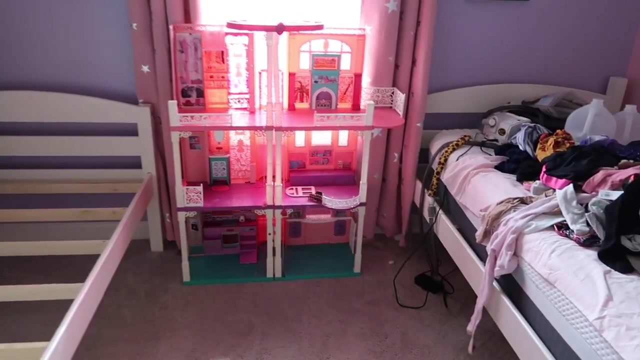 wanna tear us apart. there's something different about the way we are- just the way we are. there's something different about us, All right. so this is the part that it starts getting harder, because I need to go through these little monotonous things. This Barbie dream house was over in my son's room because. 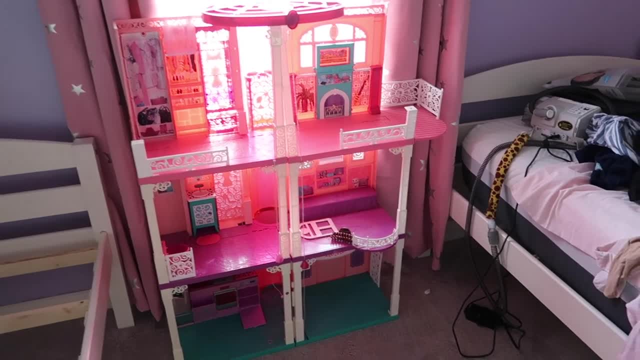 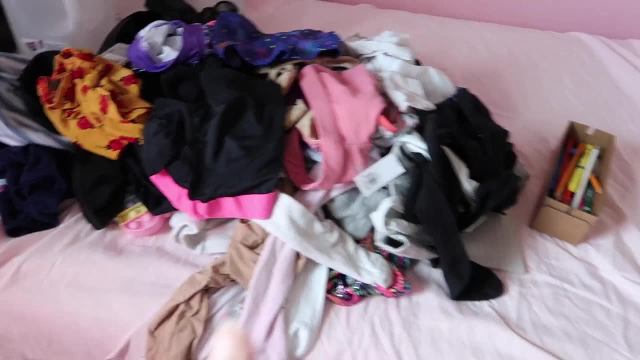 there just wasn't room in here with that white dresser, and so we swapped spaces, which is what we originally planned. All this stuff was their dance stuff. that was in that dresser, so I just need to go through it and get it in their dresser over here. All these up here, my daughter has to. 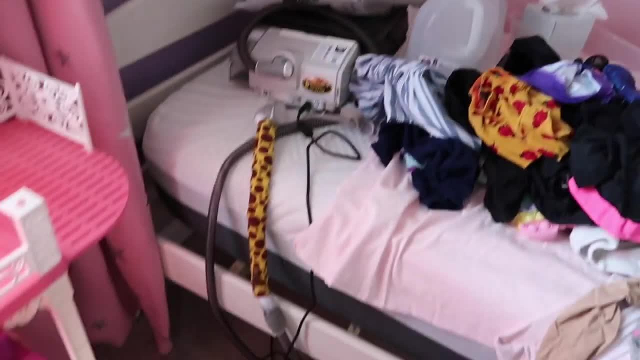 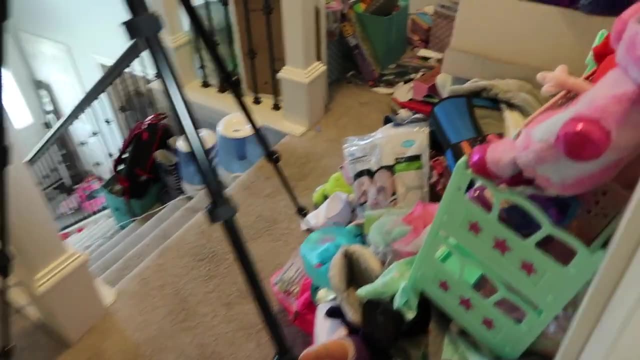 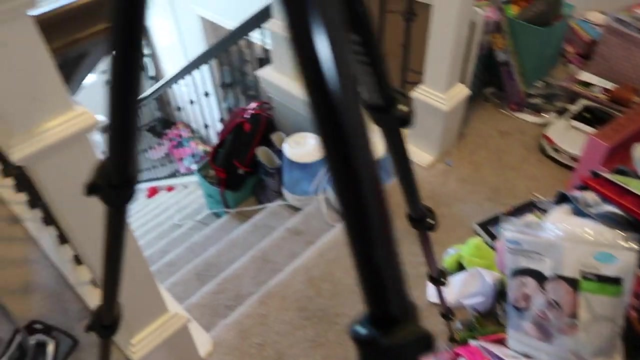 wear CPAP at night for her sleep apnea and so that's just kind of her stuff because it's going to remain right here. That's a trash bag and then out here I mean it looks bad but it's actually better than I thought it was gonna be, which is kind of crazy to end up saying Down here we have. 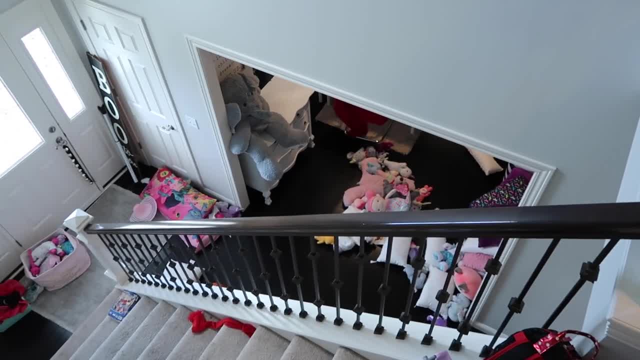 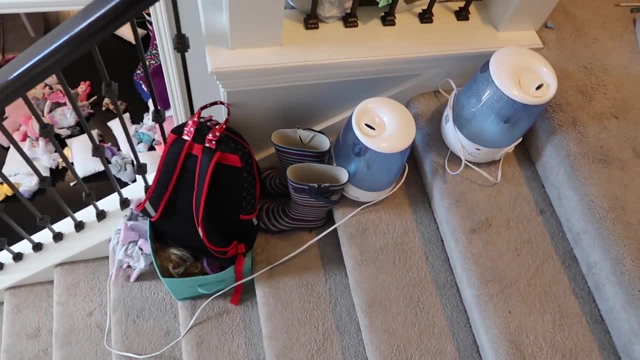 all the bedding and some stuffed animals sorted out. So over here I already have like a get rid of pile going on, and then these are like humidifiers and stuff that's going to go into their rooms and then my son's room. This is where I'm overwhelmed. 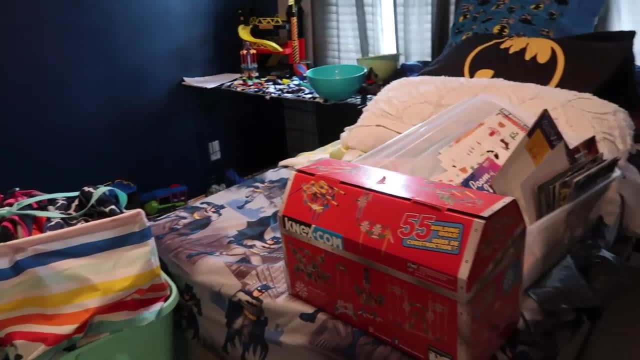 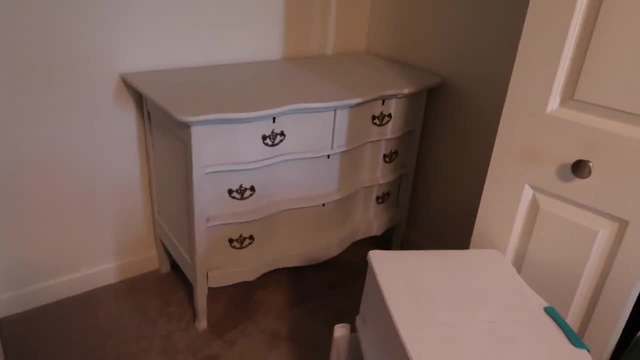 because it's like doing both rooms is making it more crazy, but at the same time, I feel like I have to do both rooms to get this to work correctly. We did put the dresser in here, so I just need to get all his hang-up clothes and his other clothes out of, like our. 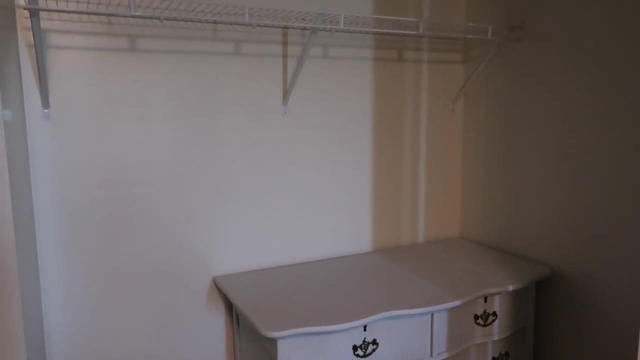 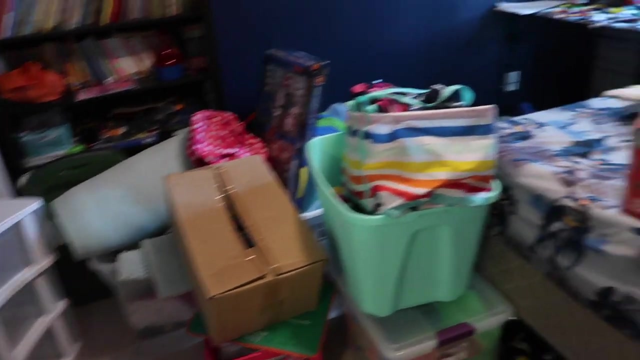 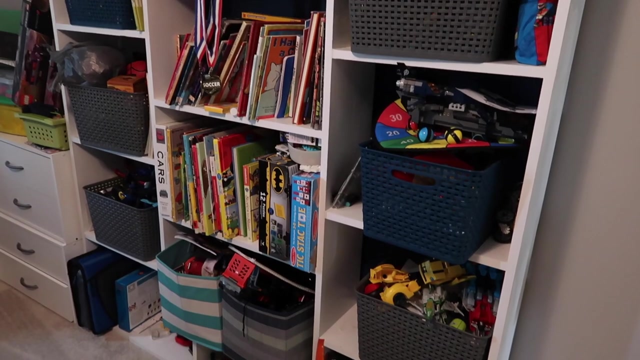 master bedroom one and get it over here- and luckily he's kind of my tidier kid. I know this doesn't look like it. all this was in his closet, though, so this is my fault, not his. Same with these two items, where most of the time this is pretty tidy, He actually does a really good job. 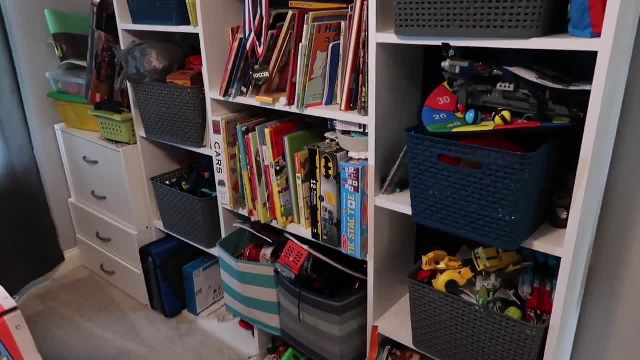 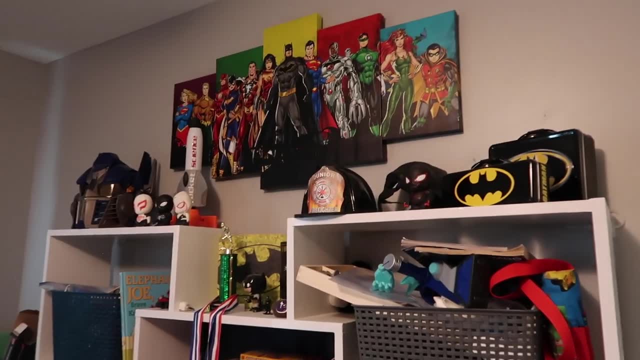 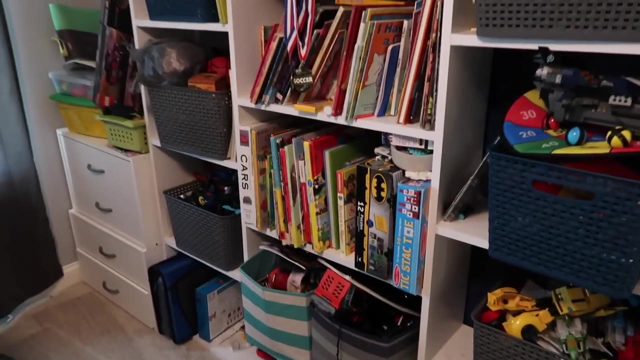 keeping stuff. but I see so many things I feel like I can get rid of and he's gonna tell me no, but I also remind him, like Christmas and everything is coming up, so if they want nice and all this nice stuff, we got to get rid of things too. So I'm going to. I kind of want to. 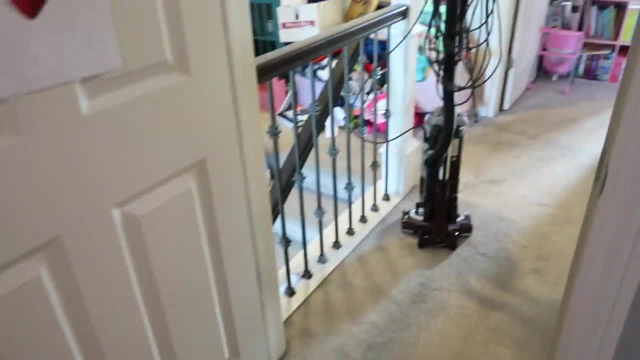 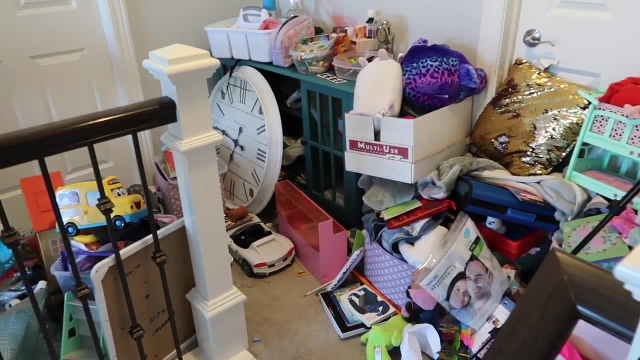 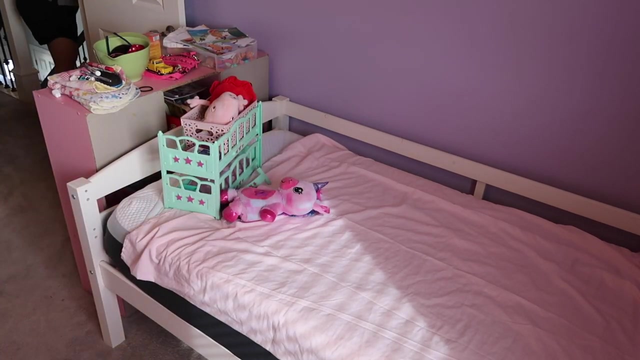 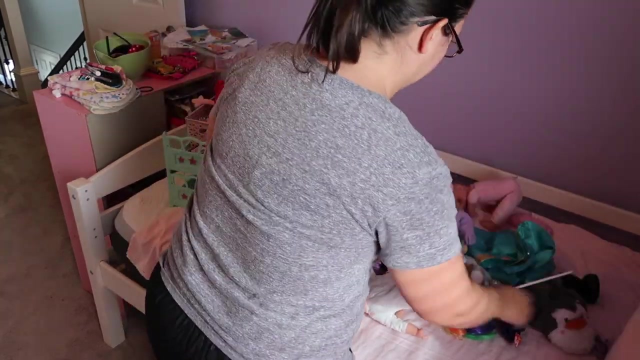 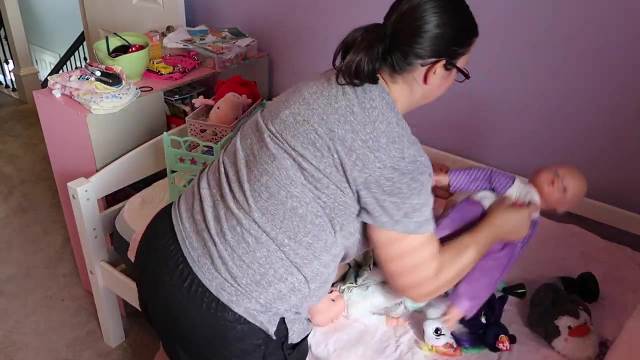 start with books. but logically that doesn't make sense. Oh, and I have laundry going. I think what makes sense is to kind of start working out here a little bit. You already know what I'm going to say. I've been feeling this way for far too long. 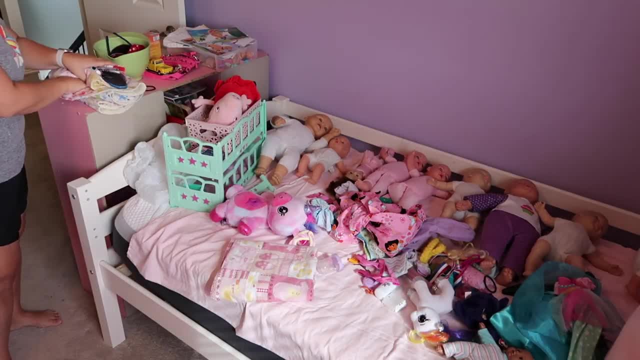 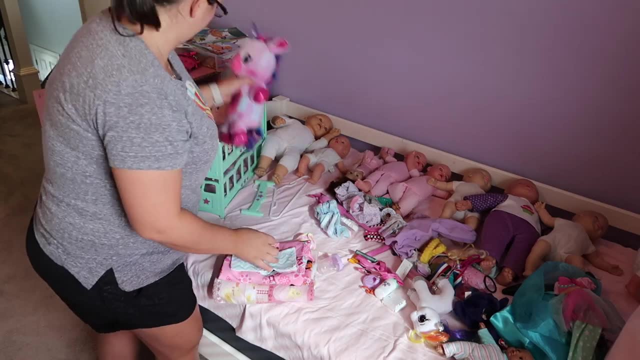 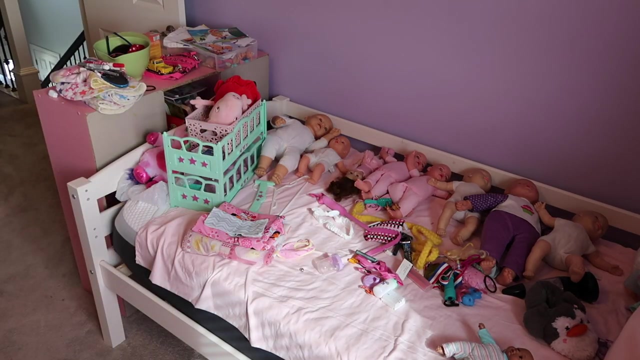 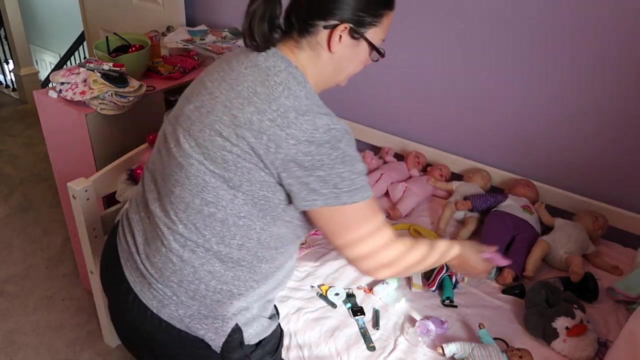 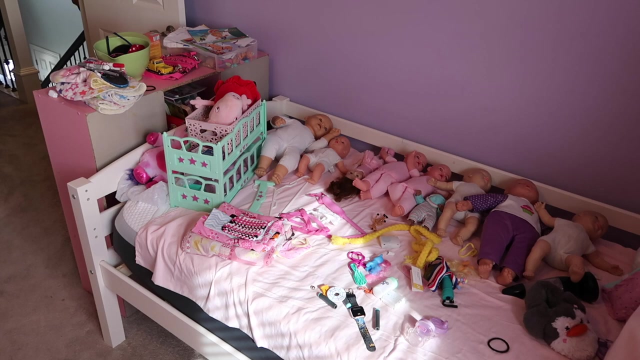 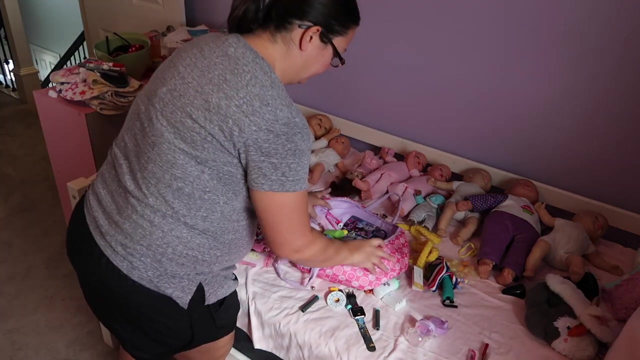 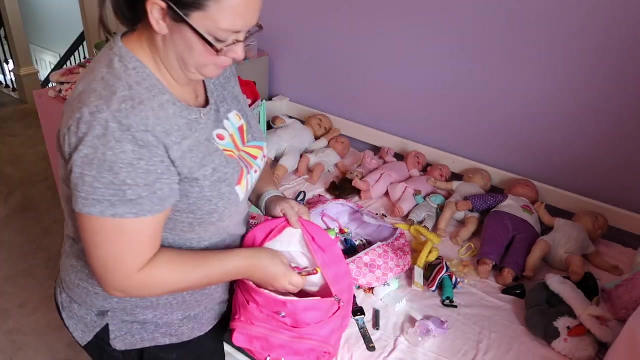 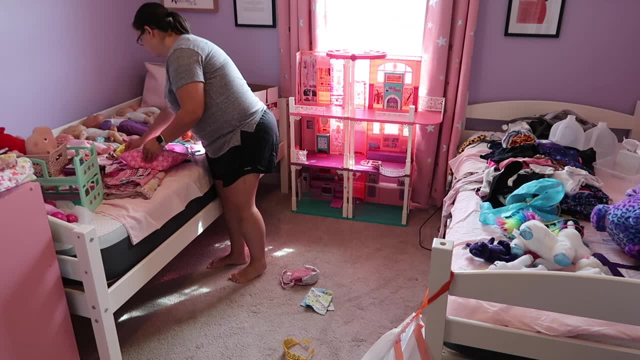 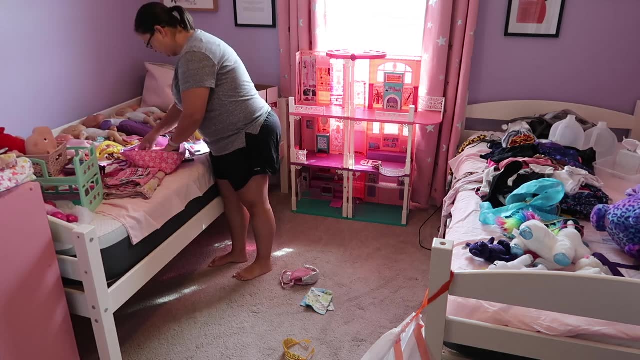 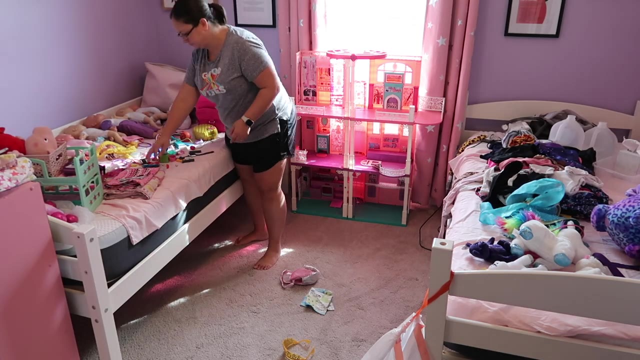 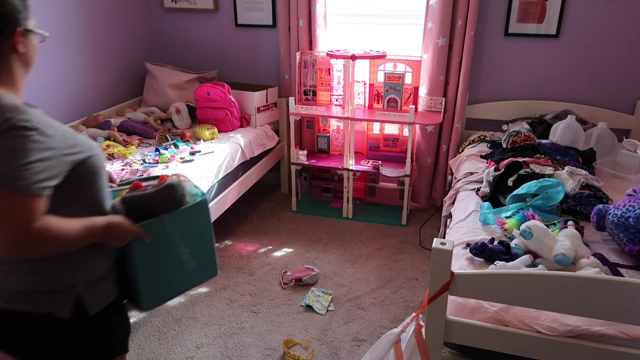 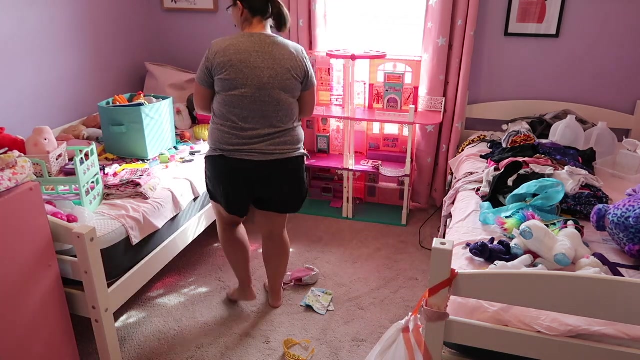 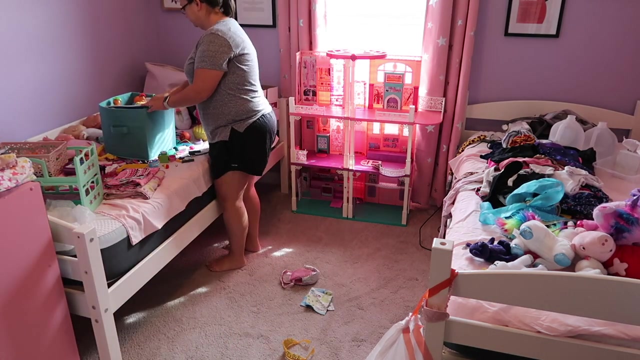 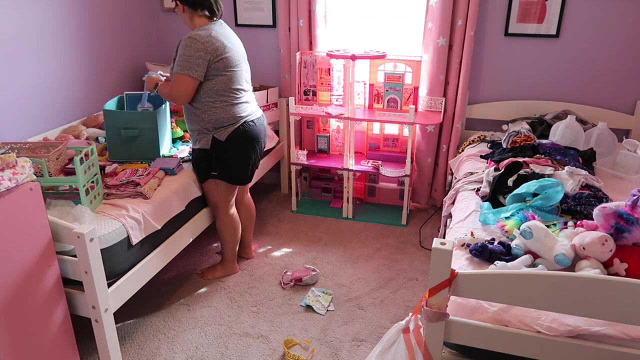 I'm in love. I'm in love. I know it's nothing new, But it's so good to see you. We do this every day And I'm still so amazed By you, So hold me tight Through the night. It's just us two. So currently I'm just pulling each bin, one by one, from the hallway into their room. 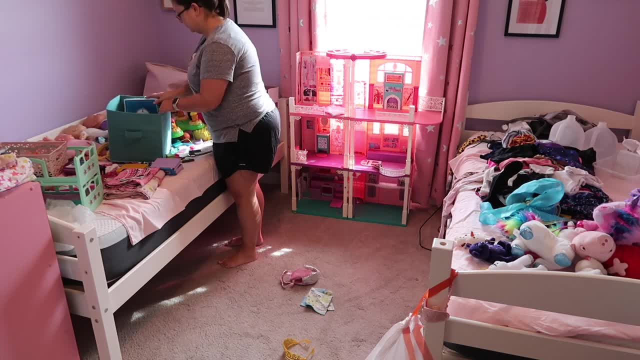 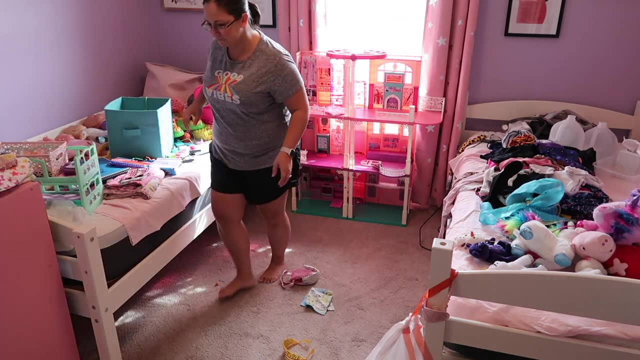 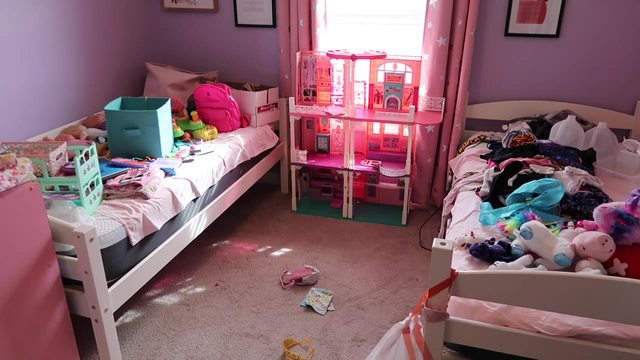 And I'm sorting them into different categories. So we have Barbies, board games, craft items, Dolls, stuffed animals, stuff like that, And so once I get them into different categories, Then it'll allow me to see how much space I need To allot a certain area for that item. 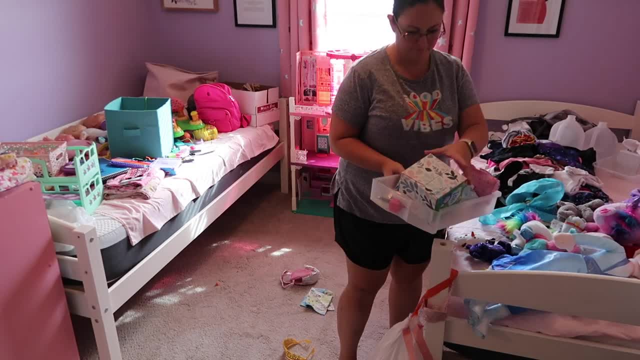 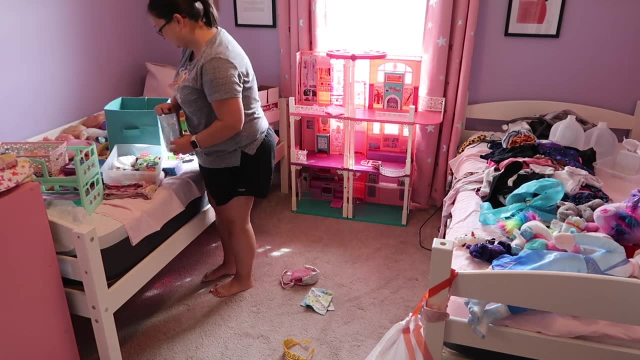 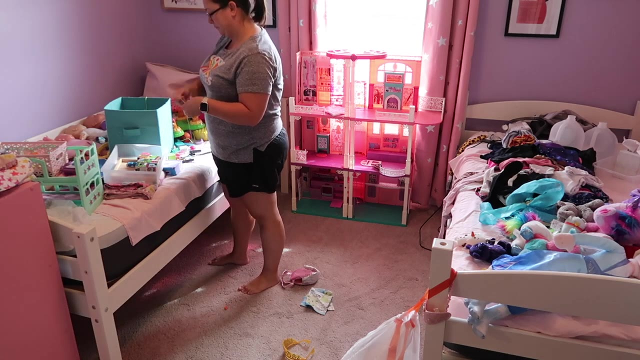 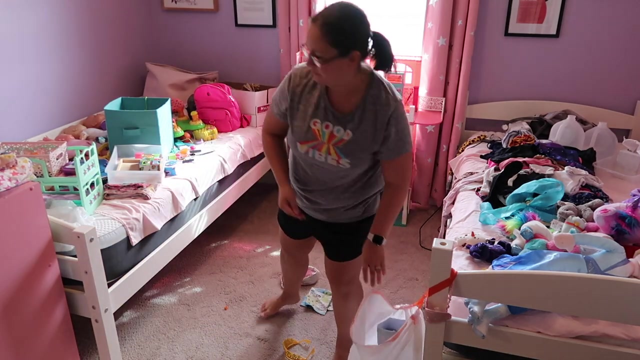 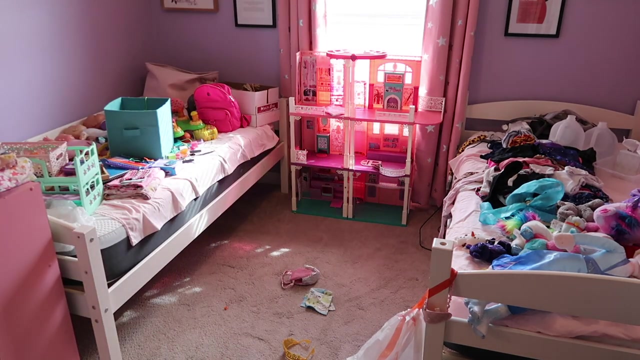 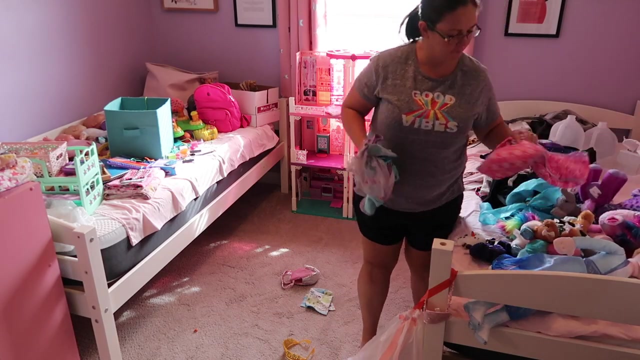 If you love me, I hope it never ends As being more than friends. Yeah, I hope it never ends As being more than friends. Yeah, You know I'm here to stay Every single day. Yeah, So hold me tight Through the night. It's just us two, Me and you. 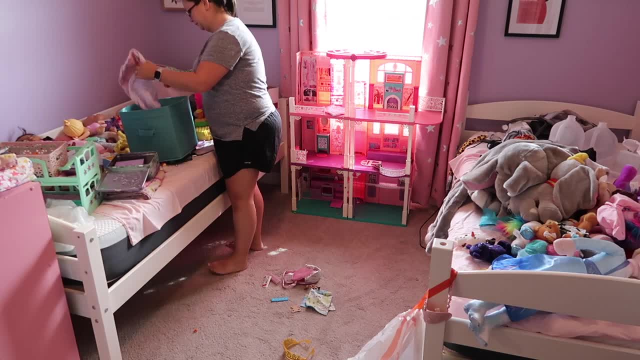 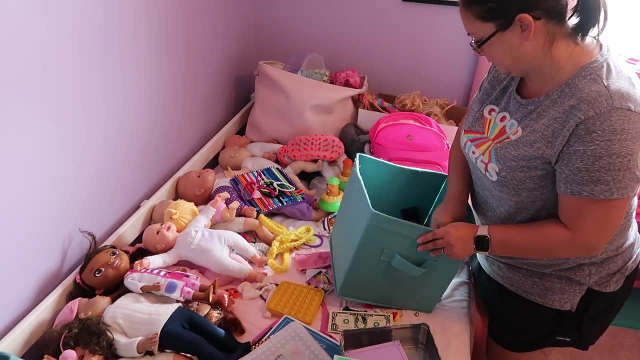 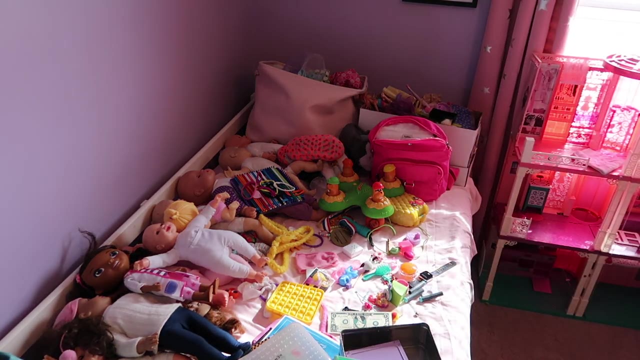 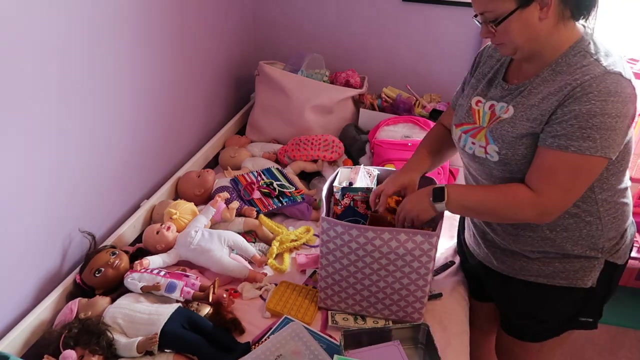 I'm here to stay Dancing up in the stars. You know where I'd rather be Than with you. Oh no, oh no. I can't believe you love me. Oh no, oh no. I just feel so lucky. Oh no, oh no, I can't believe you love me. 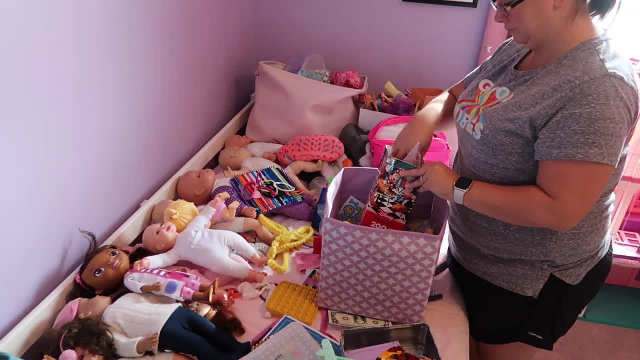 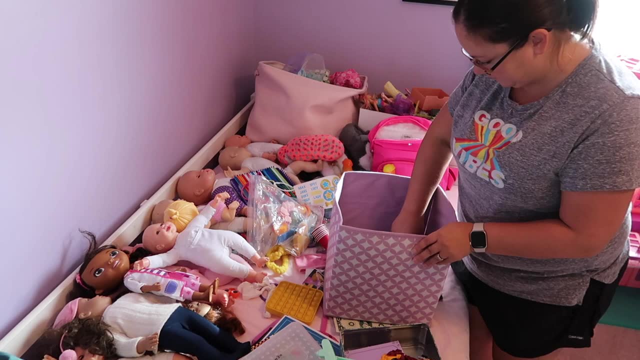 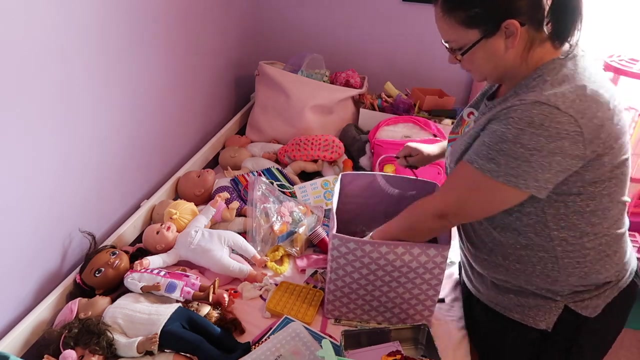 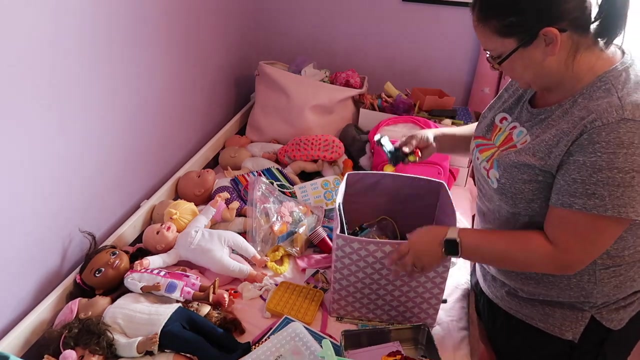 You're all, I feel so lucky. Oh, oh, still can't believe you love me. Oh, oh, oh, oh, I can't believe you love me. Oh, oh, oh, oh, I just feel so lucky. Oh, oh, oh, oh, still can't believe you love me. 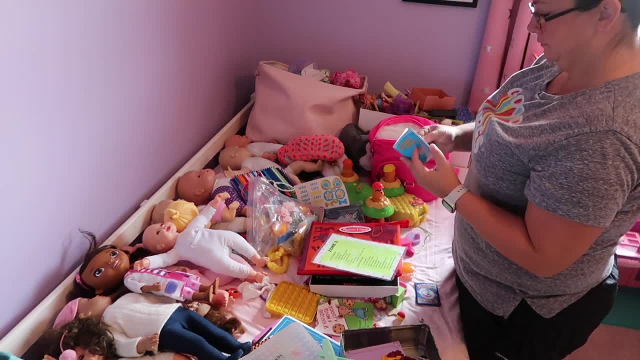 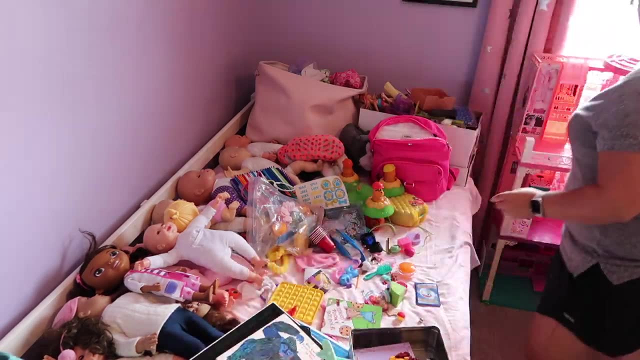 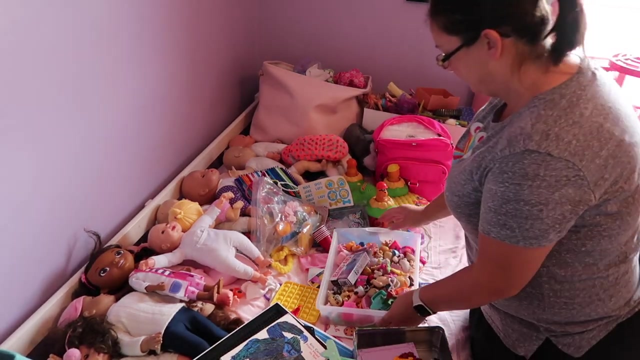 Oh, oh, oh, oh, yeah, Oh, oh, oh, oh, yeah. So cause I'll give her like a party. Listen up, yeah, it's time to start it, And I- and I know you- got it- Get with me, let's rock this party. 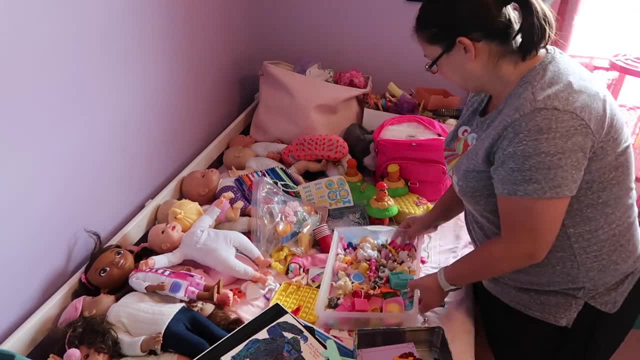 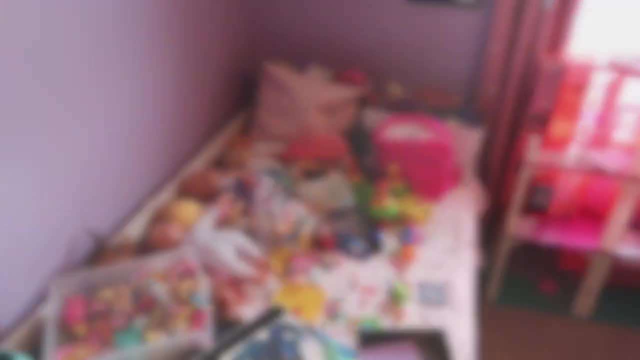 All the girls on the side say, And all my fellas on the side say: It's never gonna fly high to the sky, Cause we're gonna have a taste of the good life. Here we go, here we go, here we go up. We're gonna rock this road to the close up. 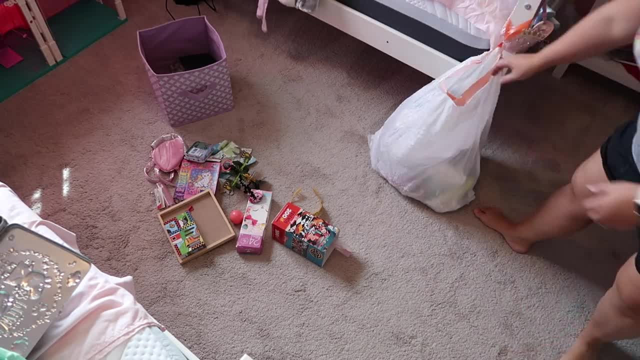 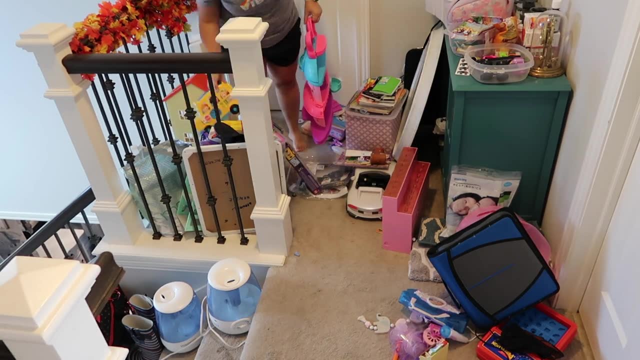 Yeah, we're gonna live the good life. Yeah, we're gonna do it all night. So I was at this for quite some time And I know it doesn't look like in this hallway Like I'm making any progress, But I really was, And there was not a single thing in this room. 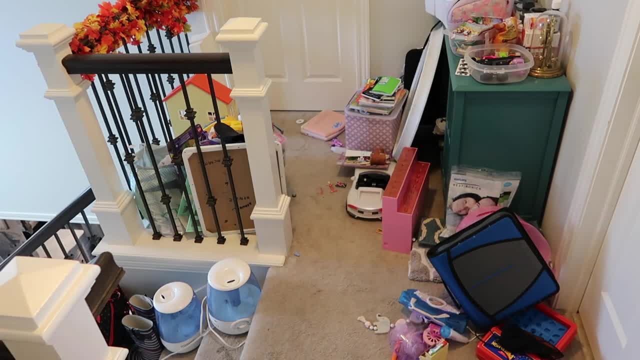 That I wasn't touching, and organizing, Making sure we actually wanted it, We were getting ready to go And we were getting rid of a lot in the end And it felt really, really good. But all this takes, you know, time And it's a process. 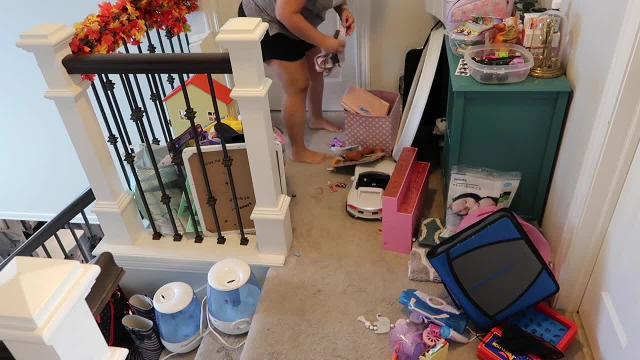 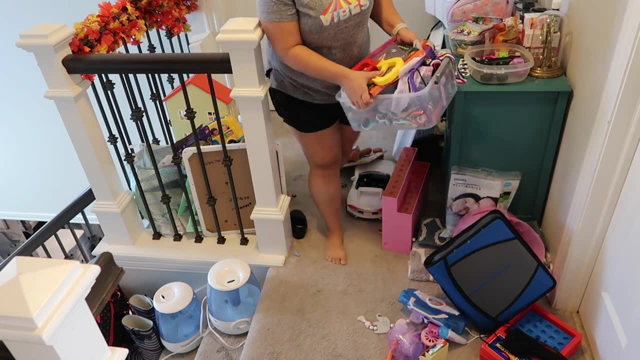 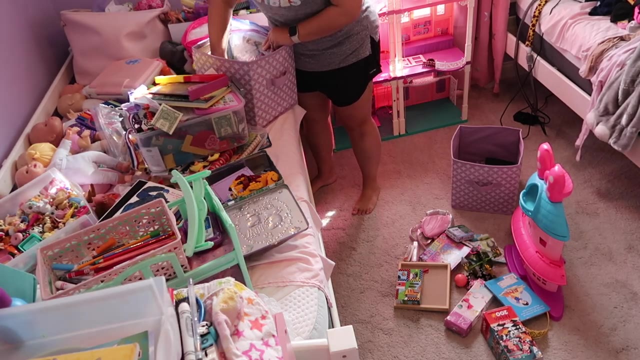 And it always gets worse before it gets better. So we're gonna live the good life, The good life. We're gonna live the good life. All right, Let's go and live the good life, The good life I'll show you when you pass me by, girl. 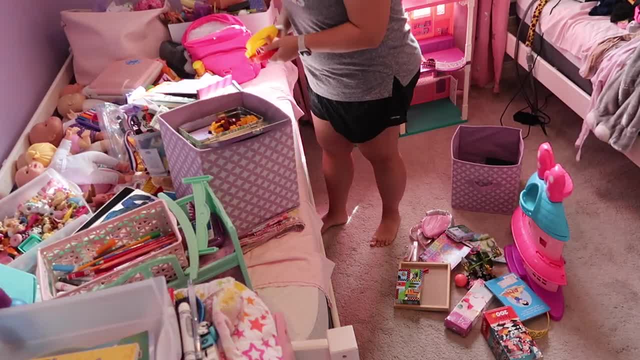 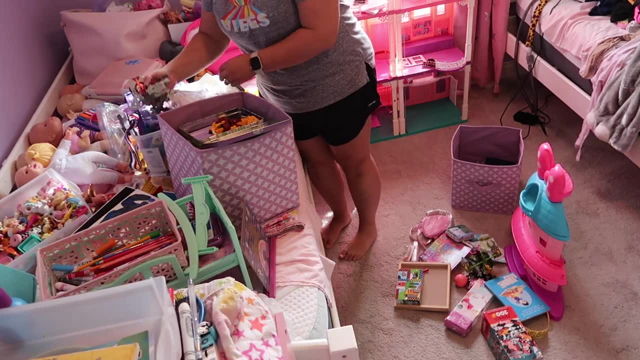 Listen, baby. yeah, yeah, It ain't a lie, girl, And I- and I can't deny That your sexy little booty caught my eye, girl, Listen, you don't have to be this shy girl, No matter where. you know, I'm not the guy girl. 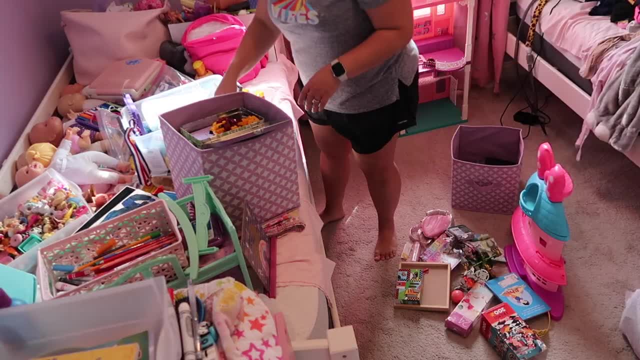 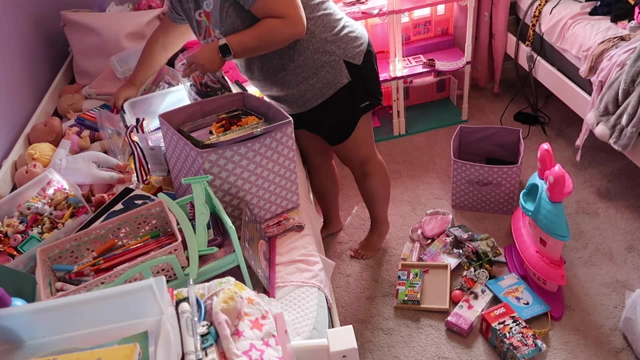 Listen. yeah, I know that we could fly Up in the sky. At least we could try girl. Yeah, you know that I've been around this town. Nothing else for some to play with. Yeah, I know I finally found you girl. I know I've found you girl. 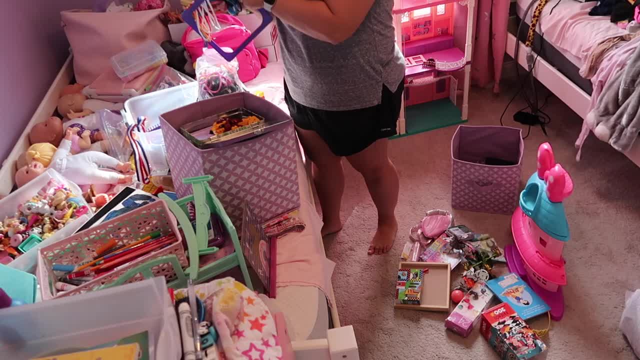 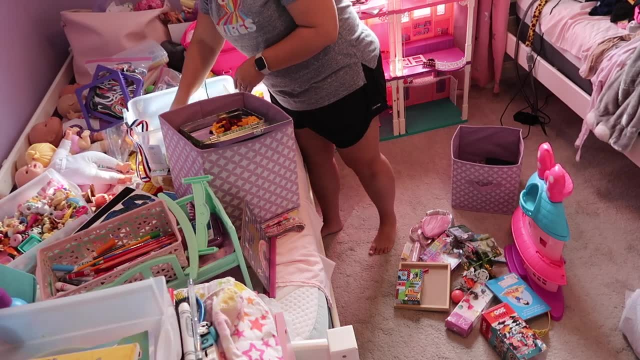 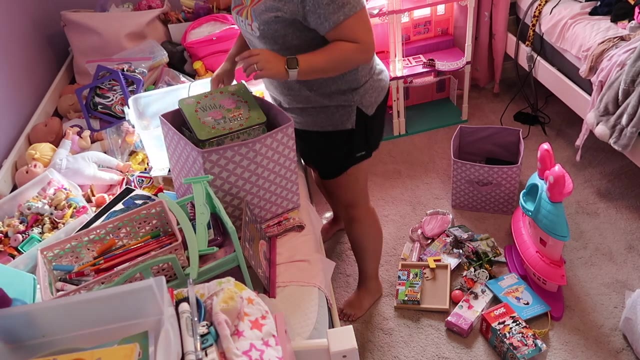 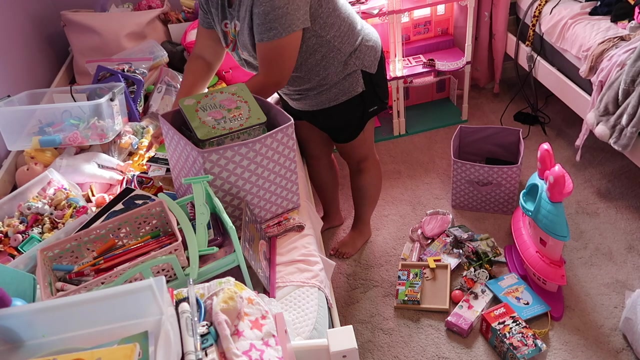 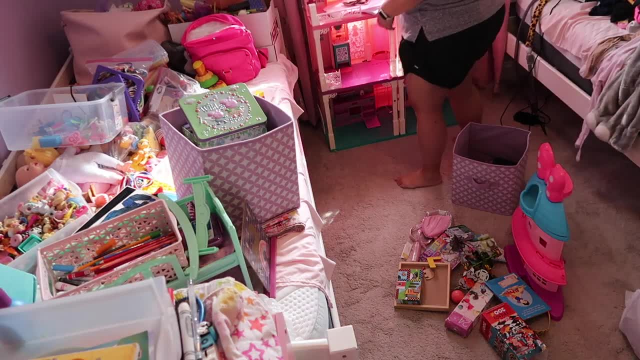 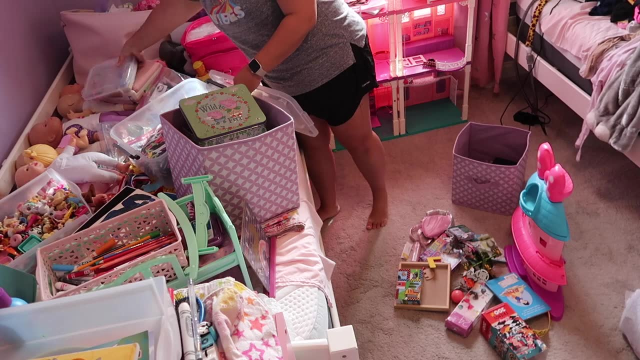 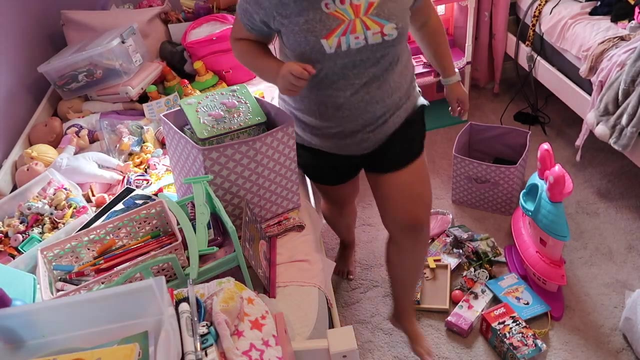 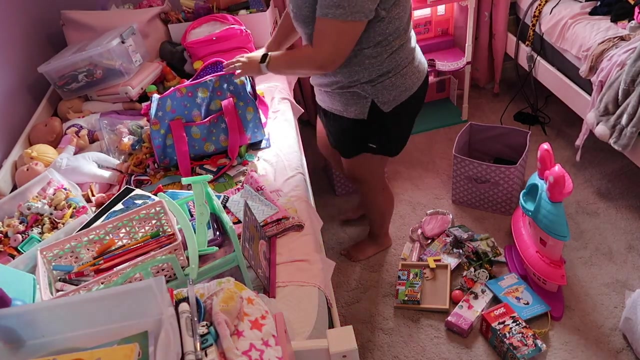 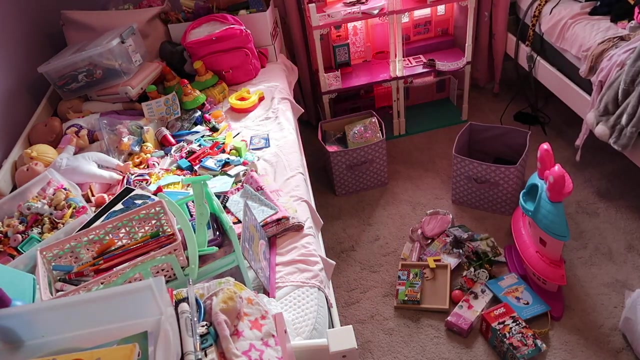 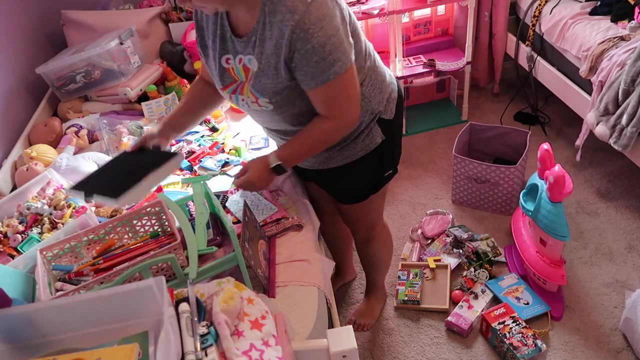 The good life. Let's go and live the good life, The good life, The good life. Come, you, come with me, Come, you come, come with me, And I'm gonna live the good life. All right, Live the good life, The good life, The good life. 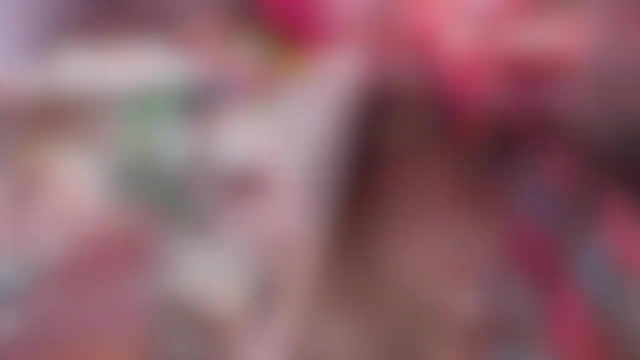 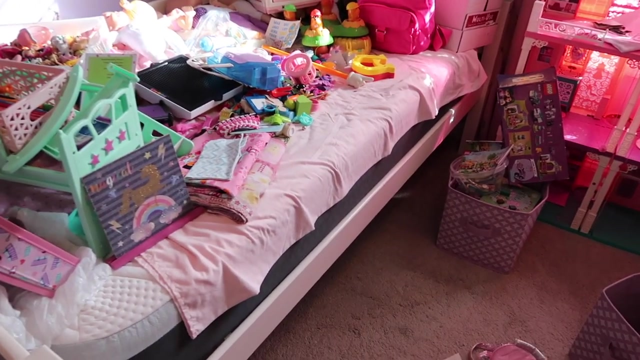 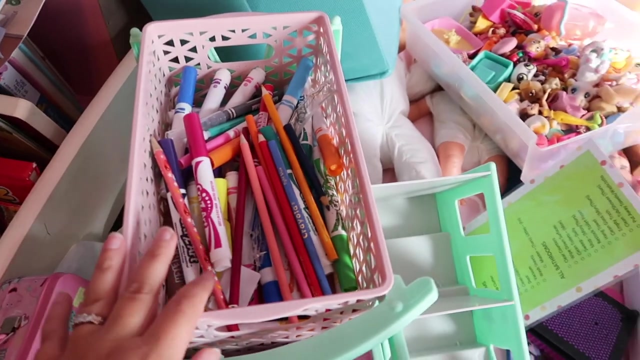 We're gonna live the good life, The good life. All right, guys, We have a hot mess express going on, But this actually makes a lot of sense in my head. So over here I have different, Like this green bowl. here is all the hair stuff. This is all markers and writing utensils. 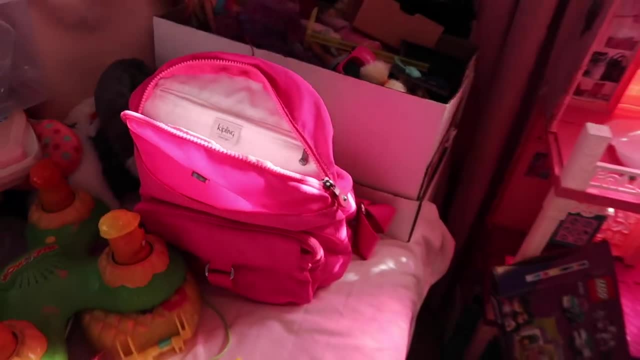 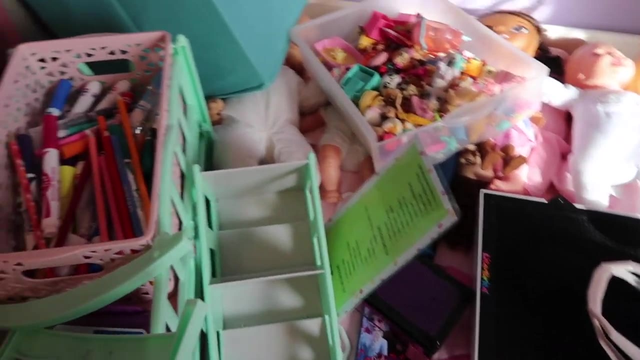 Along with this pink bag here Has a whole bunch of them. My kids love taking that stuff away with them, Like on car rides and stuff, And so I'm just gonna make it portable, Because the more I just put it in these baskets It doesn't work. This has some random stuff I need to get through. 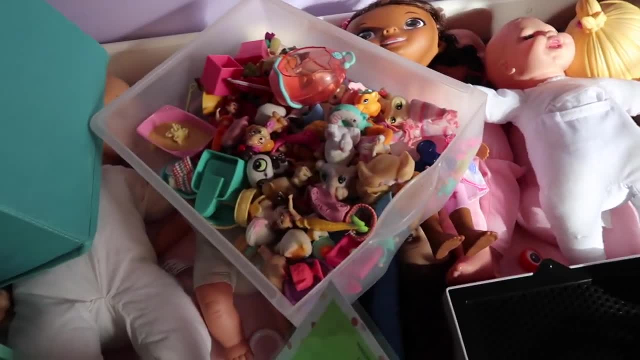 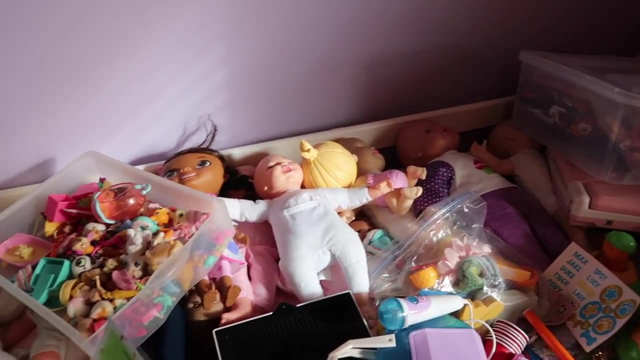 These are all. Are they little pet shop, I think is what they're called? Underneath them is all the baby dolls that we have, So I'm gonna go through those. It's hard because all four of my kids Play baby dolls together at the same time. 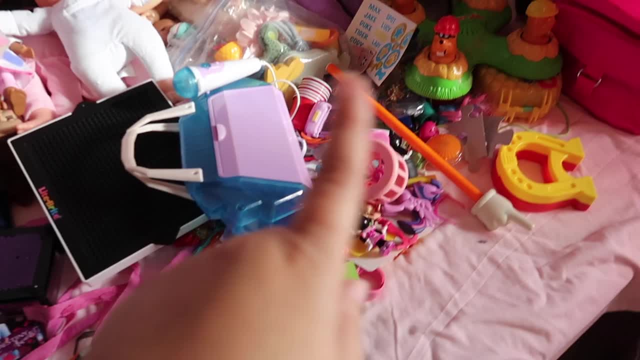 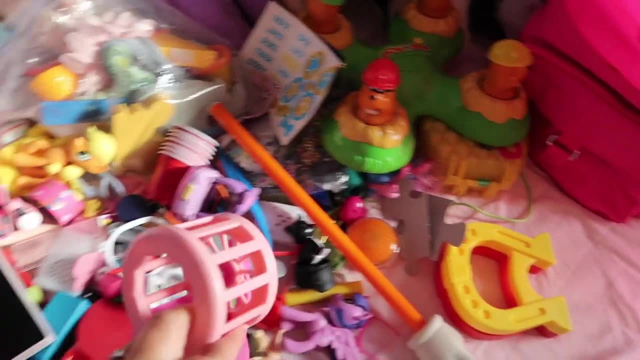 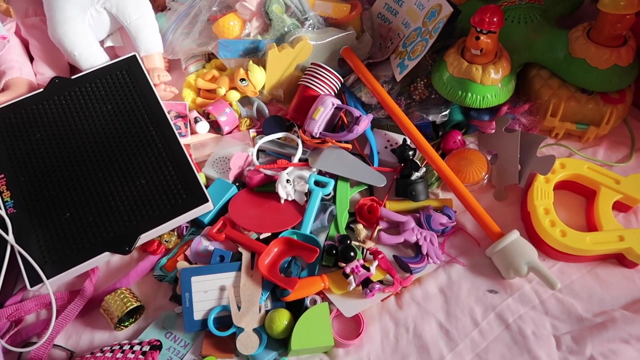 So they do use a lot of them. But I'm gonna peek through. This is the crap that gets me, Not these bigger ones. All these tiny things Drive me nuts. This is a little pet shop, So we're good on that one, But this, This Like I end up putting it back into a bin. 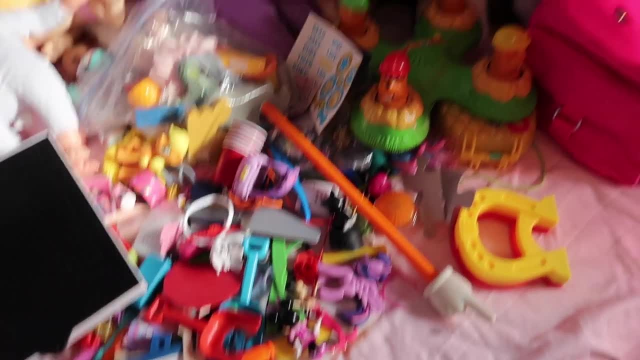 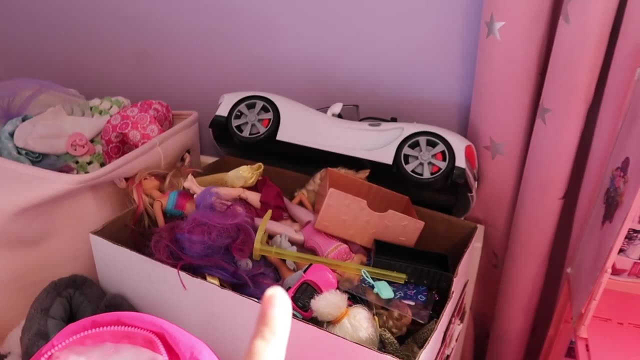 In hopes that you know, Something just happens with it And it never does. These are little craft Like: make bracelets and stuff like that. This is all the baby doll accessories And then Barbie doll accessories, So I'll be going through those. Look, found some money. That's tooth money. 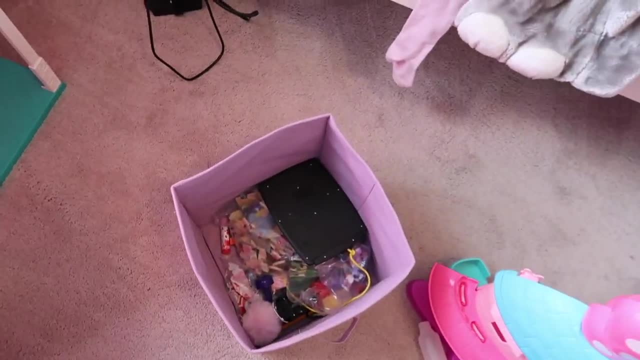 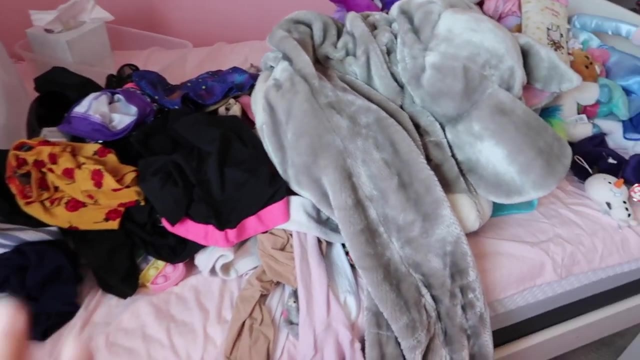 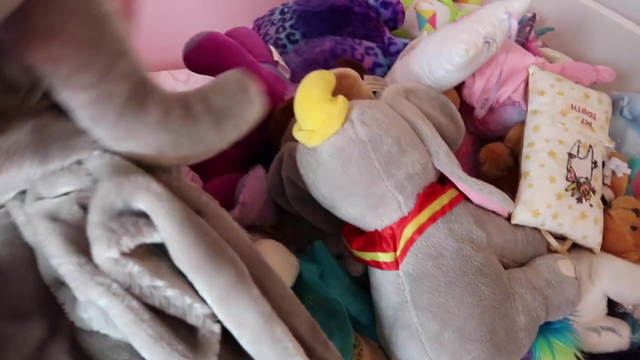 This is all Legos, And then these are like some puzzles and such. This saw my daughter's notebooks and planners That she really, really enjoys. Like I said, this was dance clothes I need to go through, But otherwise We have a couple of Halloween costumes. Yes, that is a huge elephant. 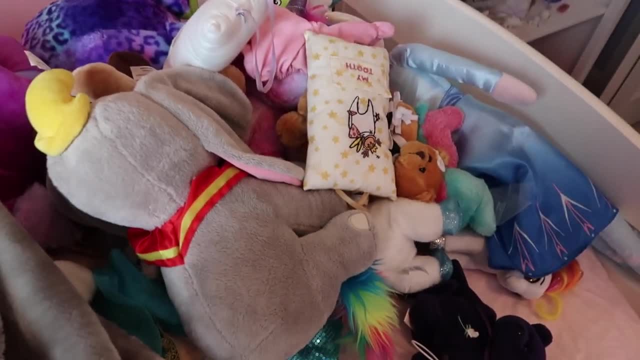 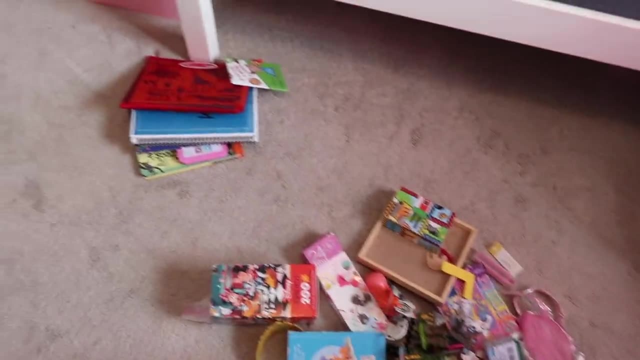 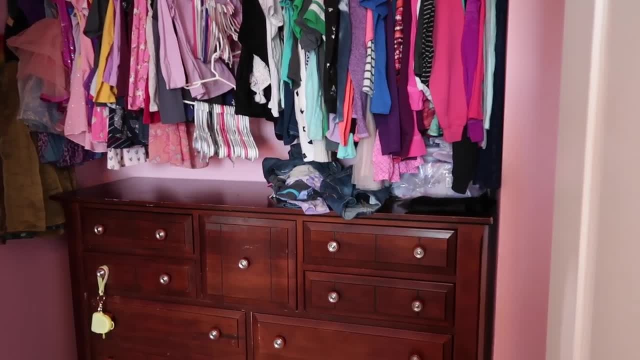 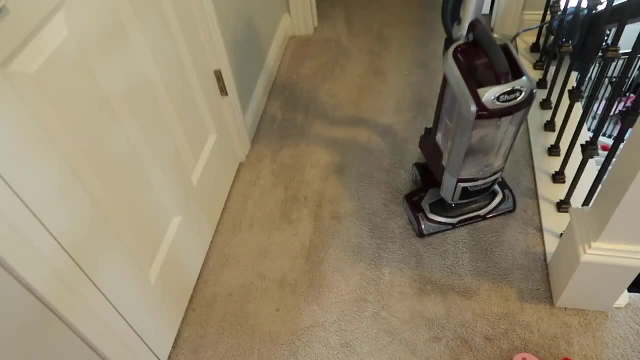 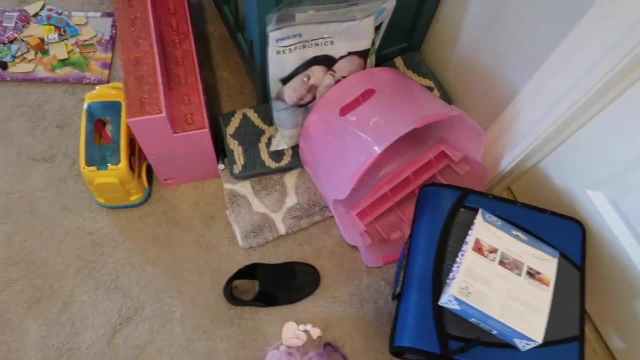 I do want to go through all these clothes and stuff, But I want, like beds, to get functional tonight first, Alright, then out here We, So all this area is still clear, And then over here. It's just tiny things that make sense to me To leave out here for now. 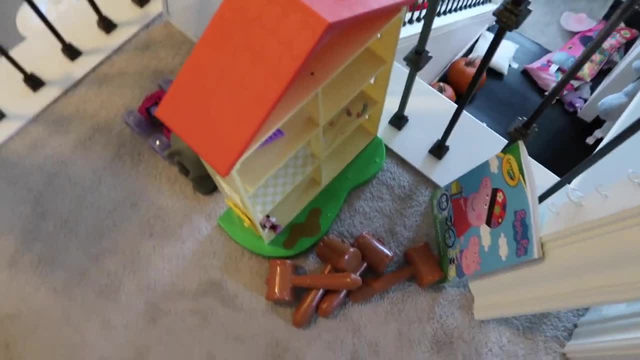 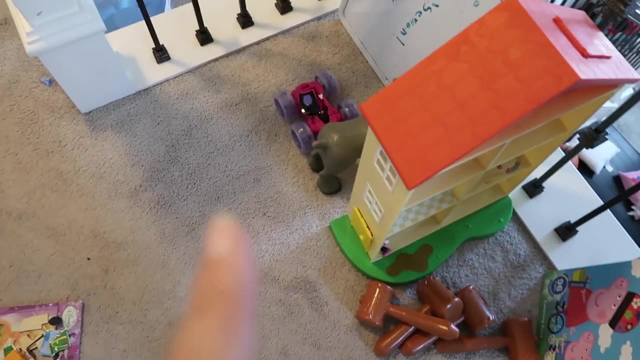 So stuff like Over here- This is for the whack-a-mole game, This will for sure be keeping. And then over here I got rid of a bigger one. This is a remote control car That I need to find the charger for, And stuff like this is for LOL dolls. 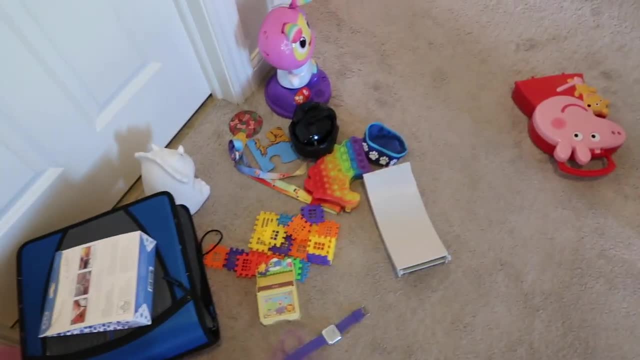 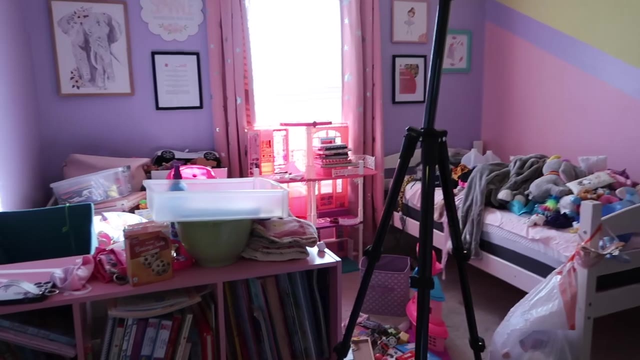 That's going to be staying, So I'm not in a huge rush of getting these Tiny things back into the room, But I think we need to start getting in here. I'm fed up with changes. Come pick me up, Cause I just want to see the light. 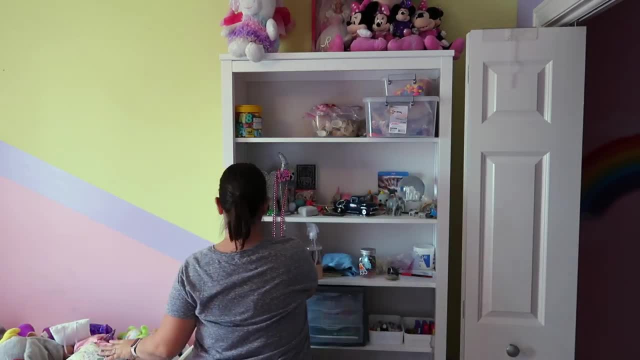 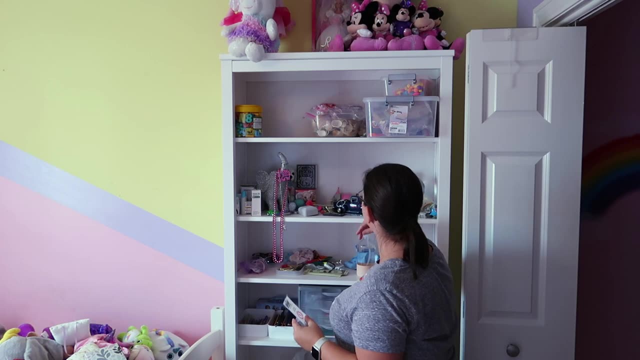 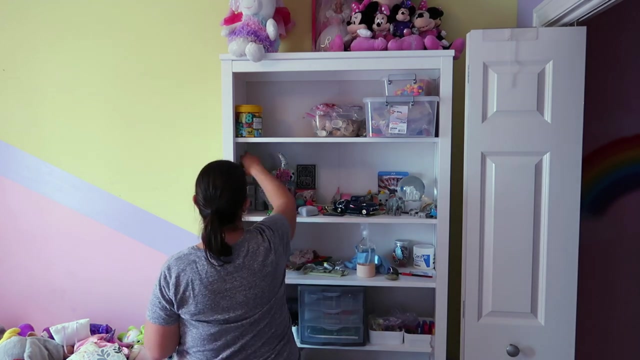 I want to be weightless Deep in my heart. Teach me to fly. I won't be coming down. Could somebody wake me up? I don't want to be here and let the world pass me by. I just see her face. wherever I look, She's standing in the crowd. 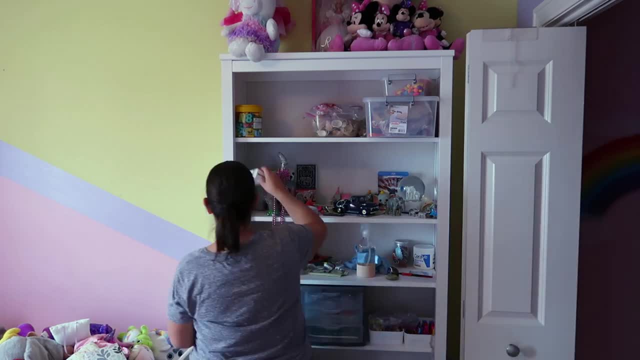 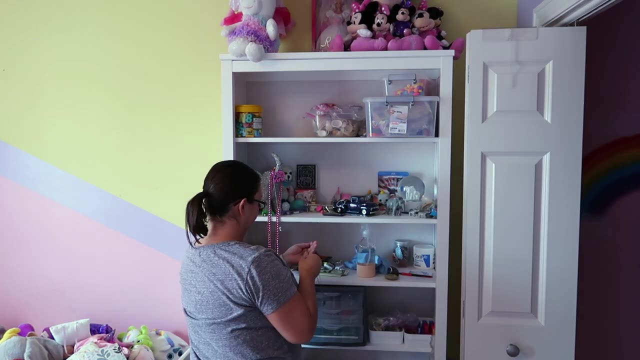 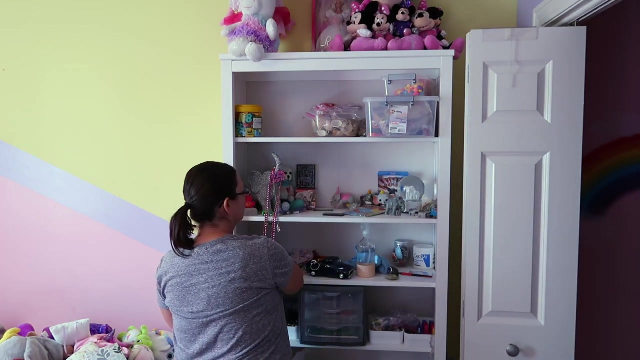 So let go, let go. I don't want to, but I'm gonna try. When she left me. Yeah, let a little bit inside you know. Let a little bit inside you know, Maybe things are gonna be alright, Cause I just want to see the light. 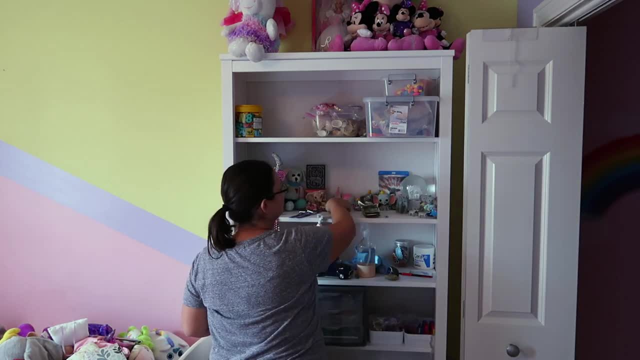 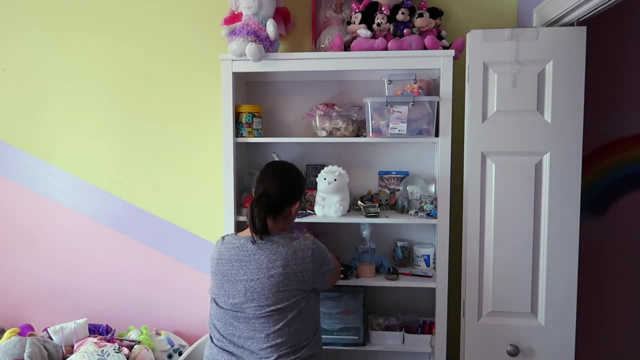 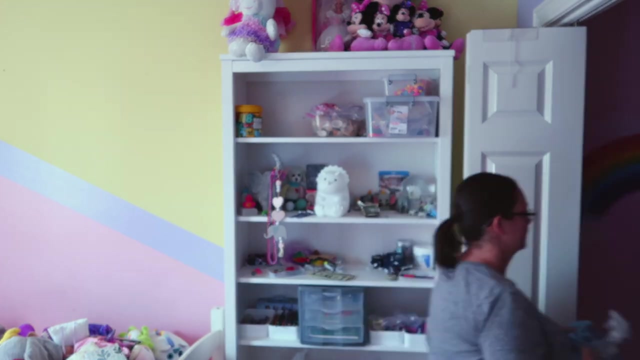 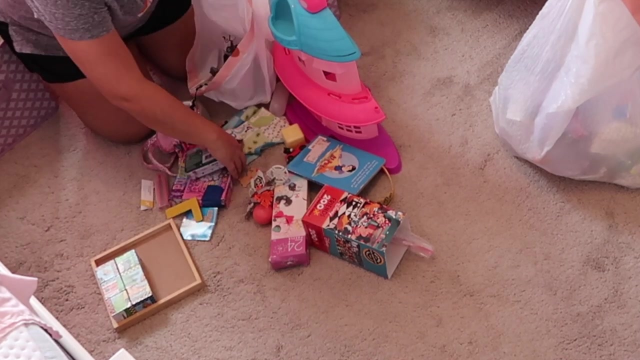 I'm so sick of waiting And getting too restless to be in this dusty town. I've heard of this place where People forget and you get another try. So come open up my door. I don't want to be here and let the world pass me by. I won't see your face wherever I look. 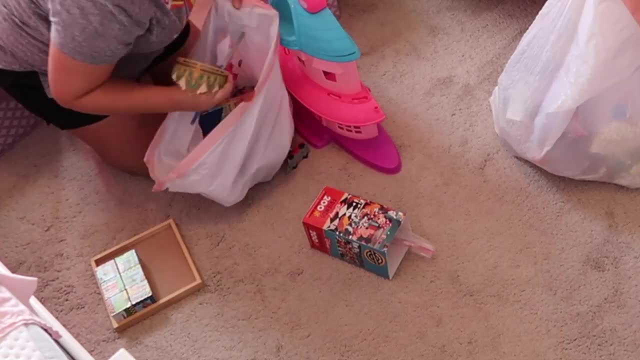 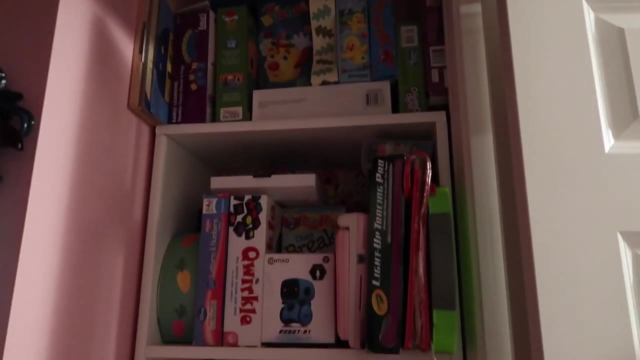 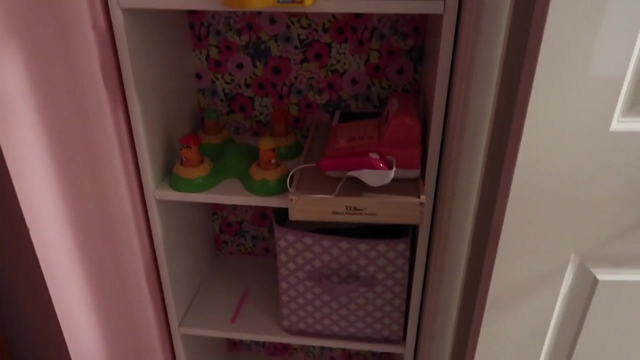 I'm blinded by the light, So let go, let go. I don't want to, but I'm gonna try. Alright. so I snuck in And I did inside the closet. This was just kind of rearranging these games a little bit And making, like, all the extra stuff come out. 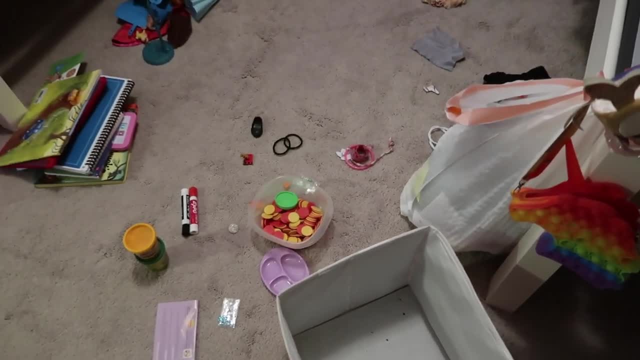 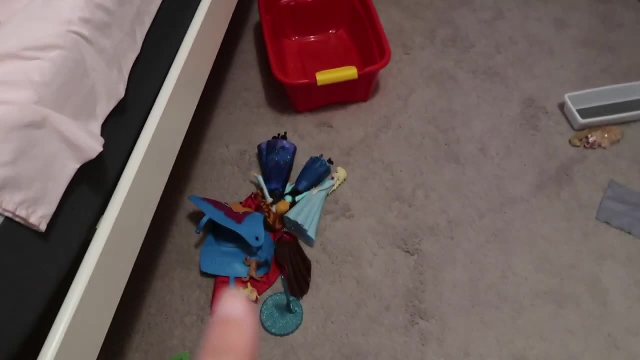 So this bin was completely full. I gave a lot of it away And then a lot of it was trash. What's laying here? I just need to get into their rightful bins. This will be for Barbie doll. I know they're frozen stuff, but it goes with Barbie doll type items. 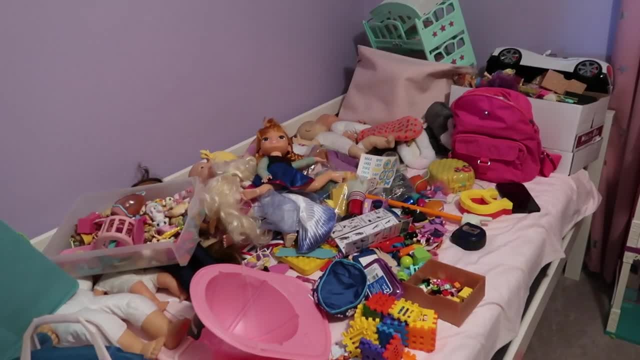 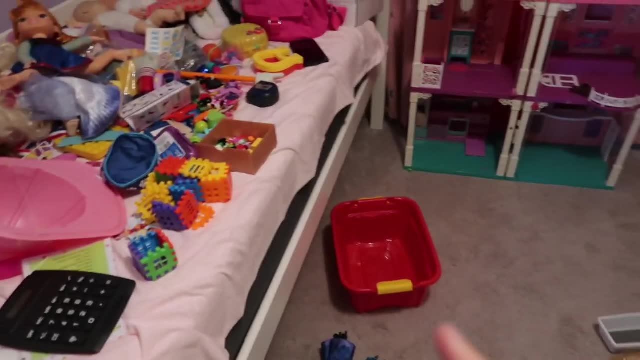 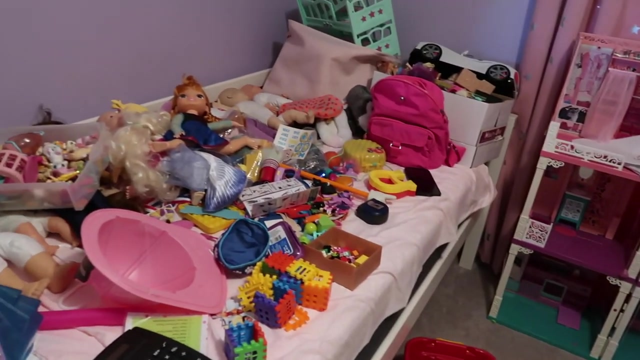 We still have a hot mess, but What I am doing is My husband's actually at Walmart And I'm gonna have him get some. I think they're three foot by six inches high And like Sterilite containers And they can go underneath their beds here, So I can stack them two high. 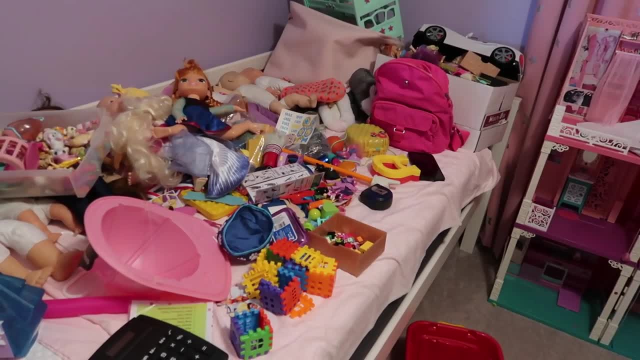 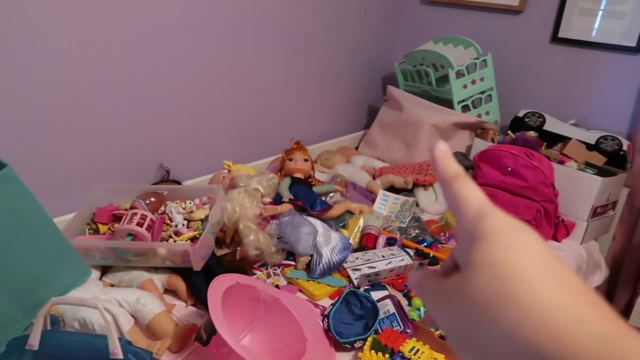 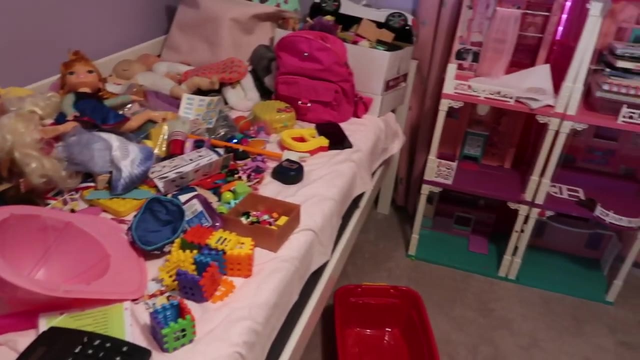 Because their beds are one foot tall. So stack them two high And I think like having two each. Like Barbie doll- Whoops, sorry, Barbie doll should go in one, All the doll stuff should go in one, And then we'll kind of find you know Extra little toys and stuff that can go into another one. 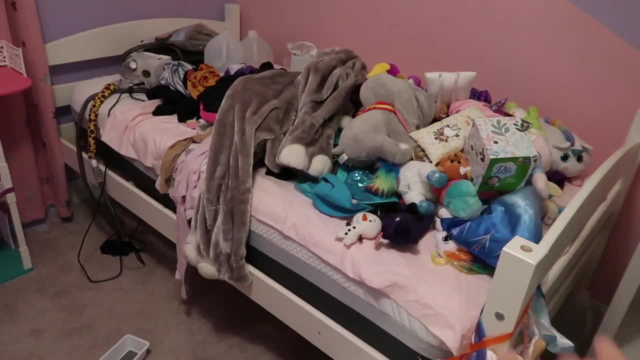 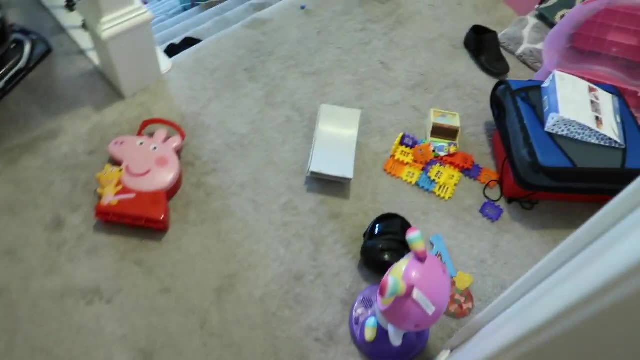 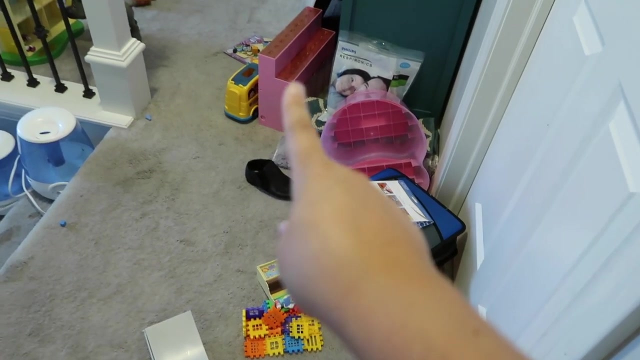 So that should suffice. These stuffed animals are kind of The bane of my existence, But I think in the meantime We're almost done out here. We're doing really, really good. These last things- Like that is a step stool that will go in their closet But then, like this, will go underneath their bed. 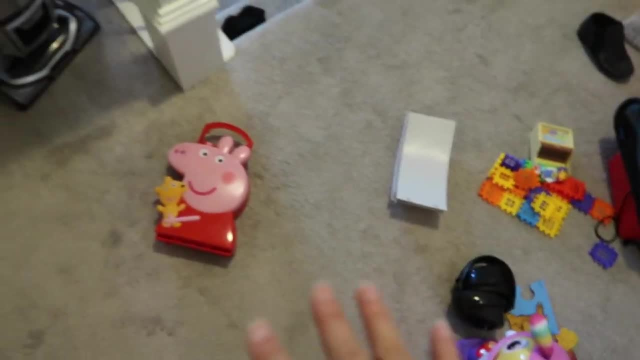 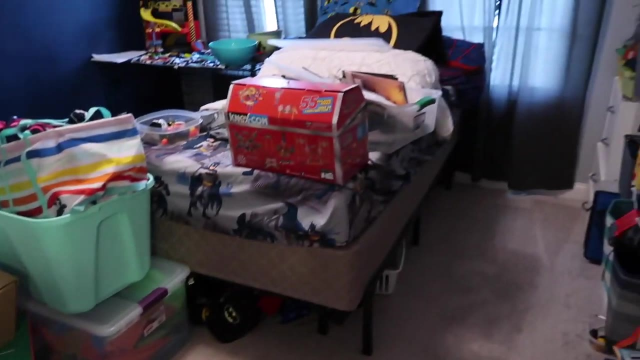 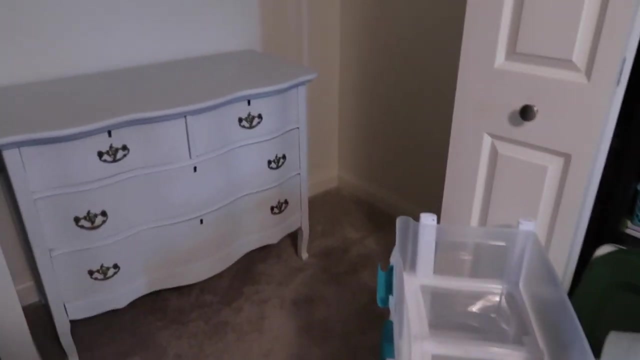 For the LOL dolls. This is like craft items And so not too much sitting out here. We might Go into my son's room. So, Again, Really big mess. But it's Like all this is me. Um, We're gonna come in here. I ended up coming in and moving this dresser over. 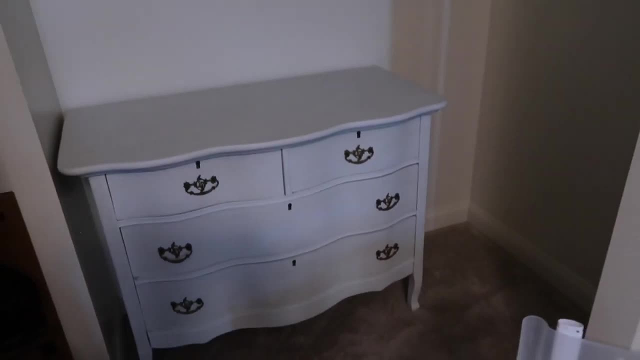 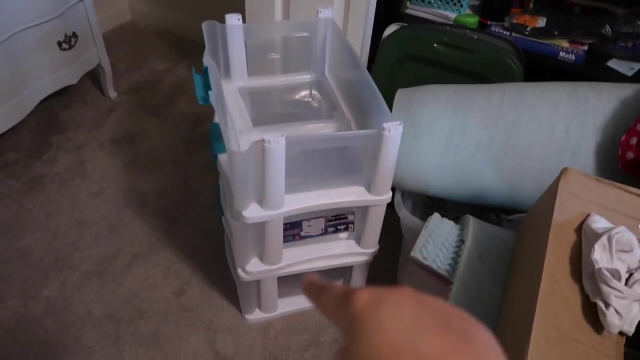 So that when he has to access it, He can walk directly in it. Um, But I'm looking at this And I'm wondering if it'll fit right there So that he can put, like some of his toys And stuff like that in here. So I think I'm gonna mess around with that. 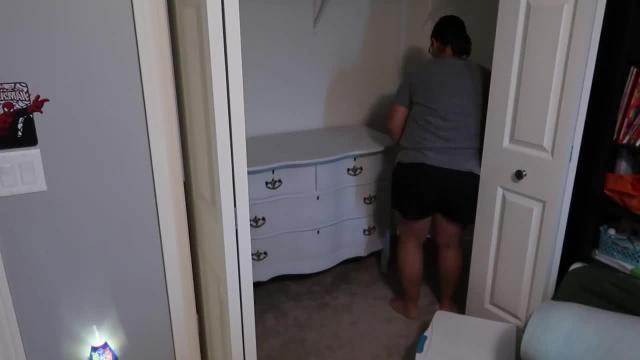 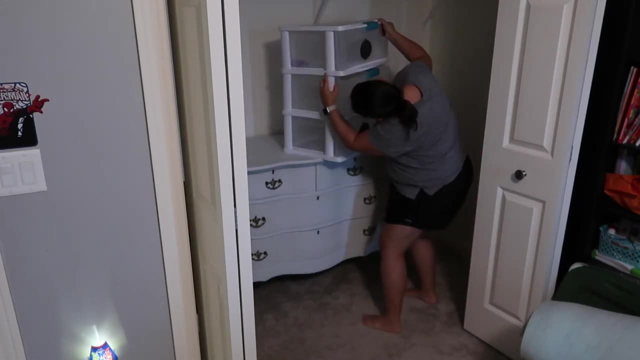 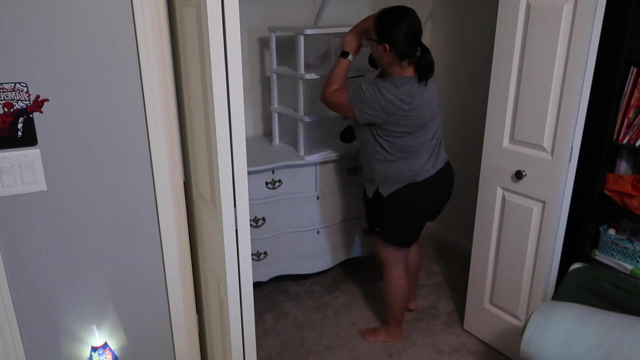 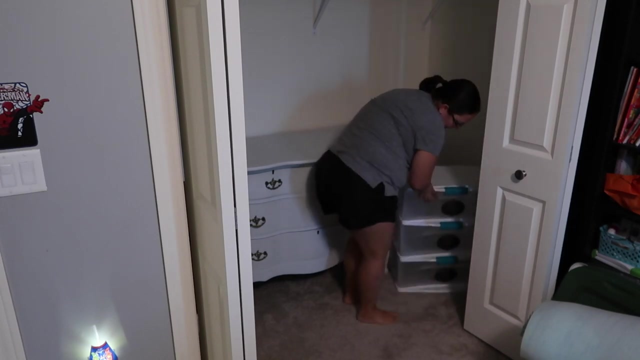 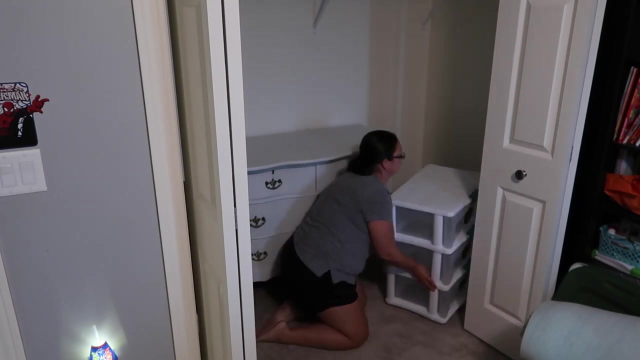 And see if that works. When she left me- Yeah, I died a little bit inside, You know. you know, Maybe things aren't gonna be alright Cause I just wanna see the light. Yeah, I just wanna see the light. I won't look back. This three drawer storage container. 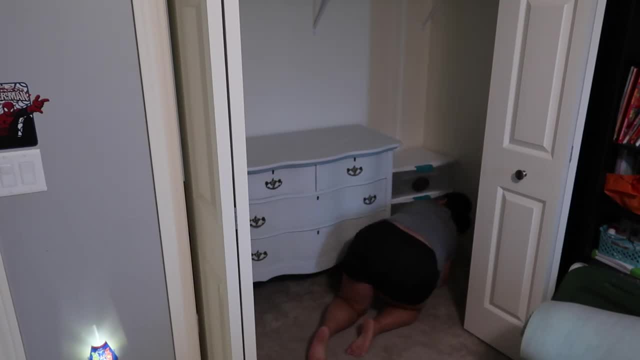 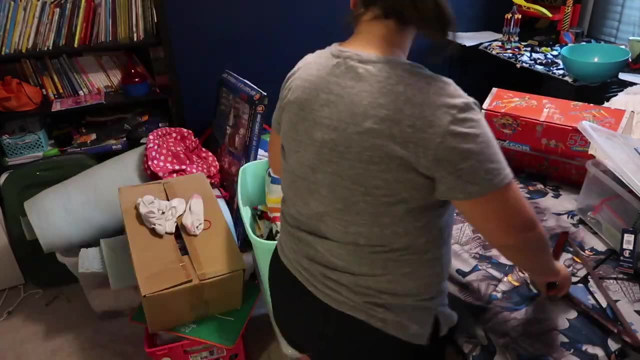 Ended up giving me a run for my money, Like I would get it all put together And then, um, It would basically get caught up on the carpet And end up coming apart again, And so I had to shimmy it in there. Exactly right. I am going to start tackling some of the stuff. 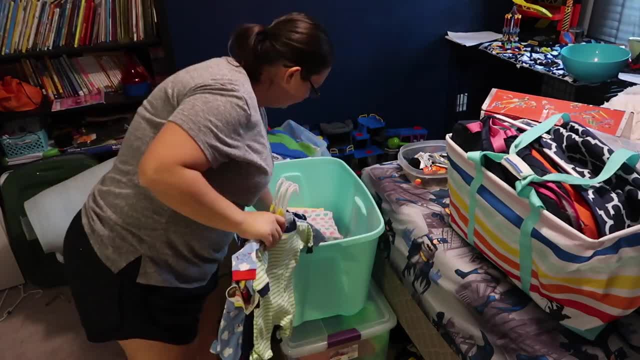 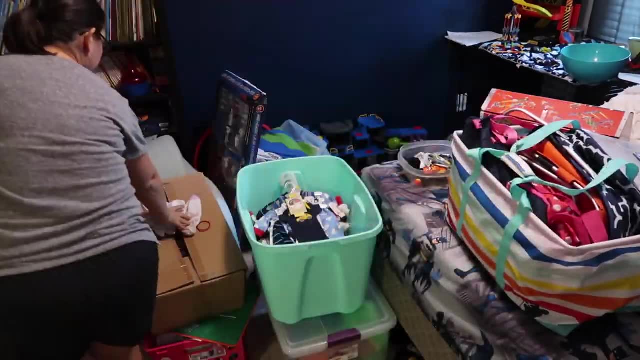 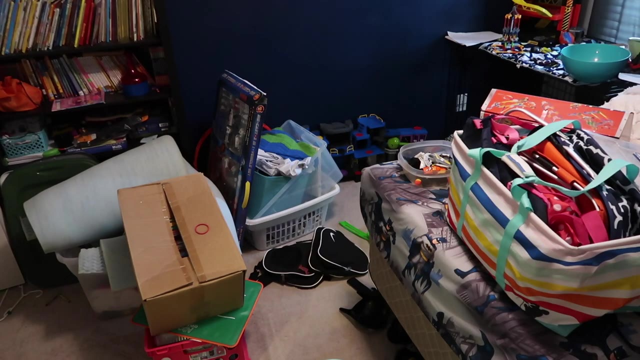 That came out of this closet, Cause most of them are pretty like Easy to tackle. So whenever I find preemie clothes Or newborn clothes Like stuff on clearance, I end up buying it, Cause I work at a NICU, So then I can donate those there, And so I need to be able to do that. 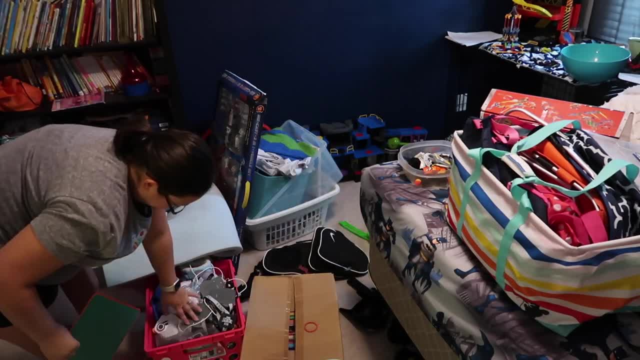 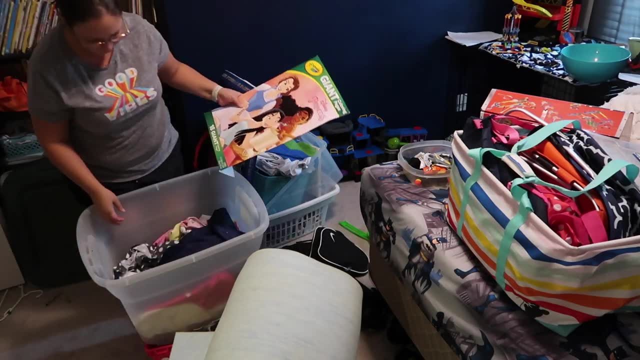 Also. um, They fit baby dolls really, really well, Like preemie clothes do, And so my kids like getting some of those Preemie clothes just for that. Um, the bag that is The colorful bag, Like the rainbow bag that's on his bed, That's just full of other bags. 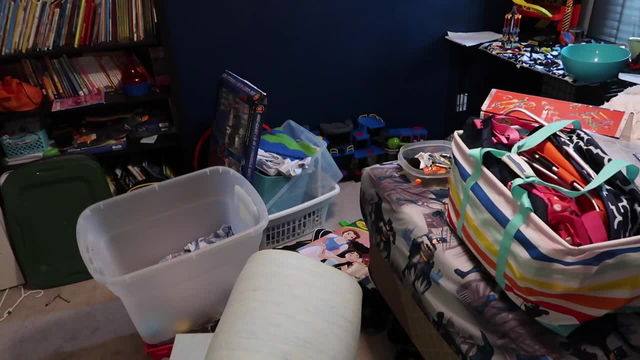 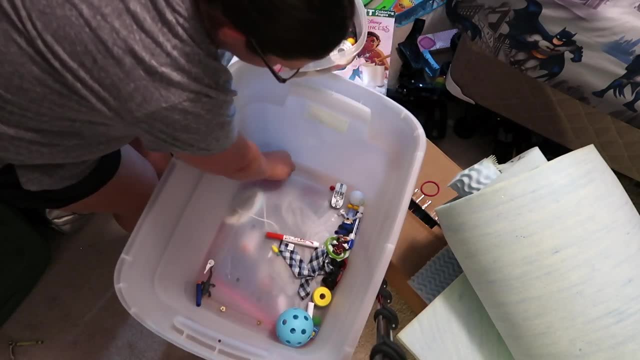 Also, so I just need to go through it And get rid of anything that I want. So all these bins, As much as they look like there's a lot of clutter And it is clutter, But as much as it looks like it's a lot, Really they were big items. 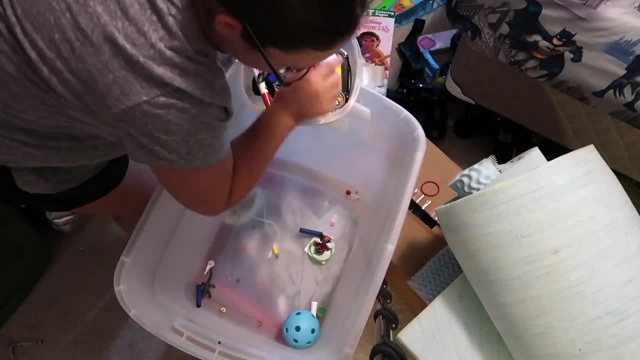 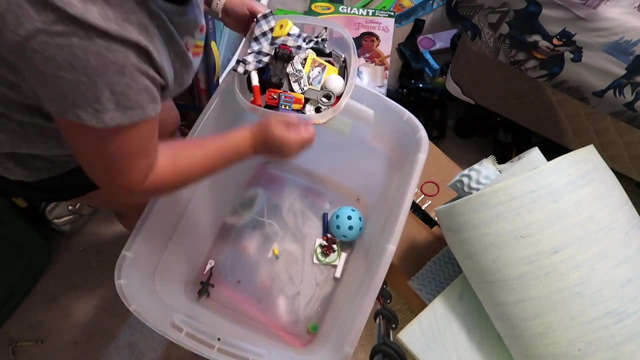 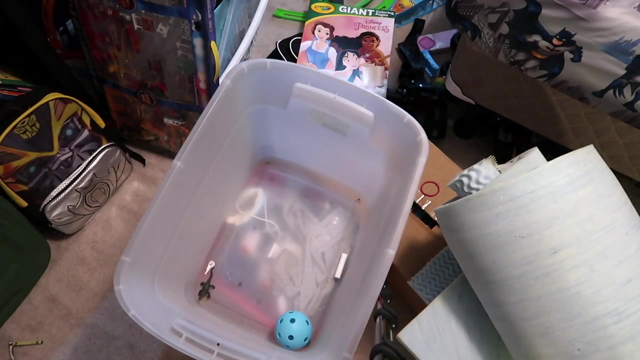 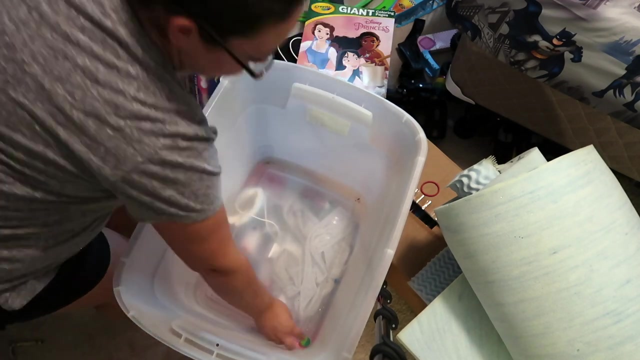 So it was really quick and easy To end up going through And if they啊 landscape Or a large store I would like to share, Do you know what I like to buy? I do not. Do you know what I like to buy? I love to buy, Of course. 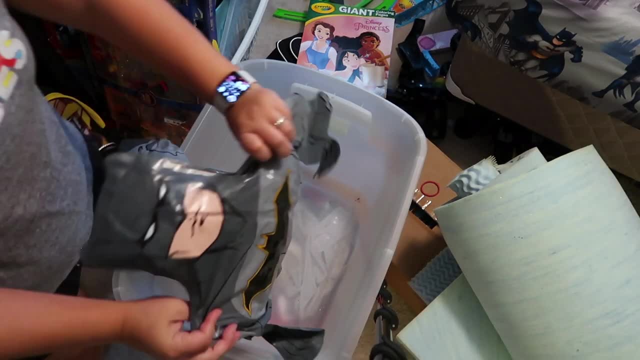 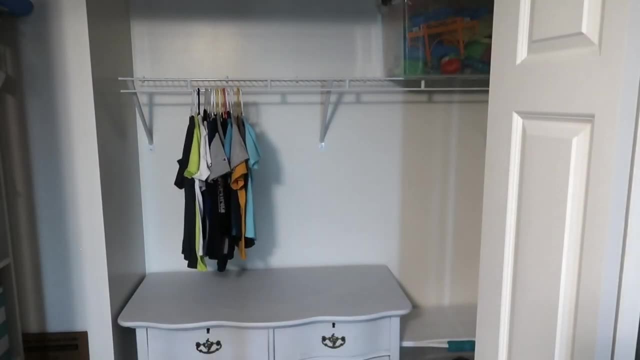 Cause I know I love to buy. I love to buy Because I love to buy, So use Some items To keep Some items. It's not a lot, So some of them, I think a little more Makes sense. If it's not something That I really like, Then you know. 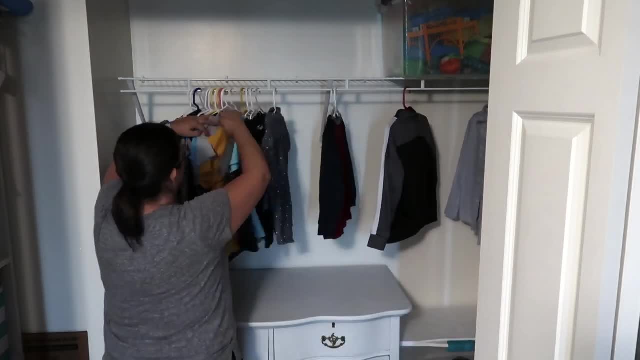 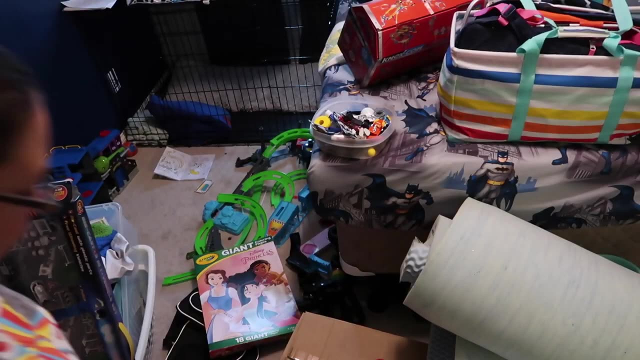 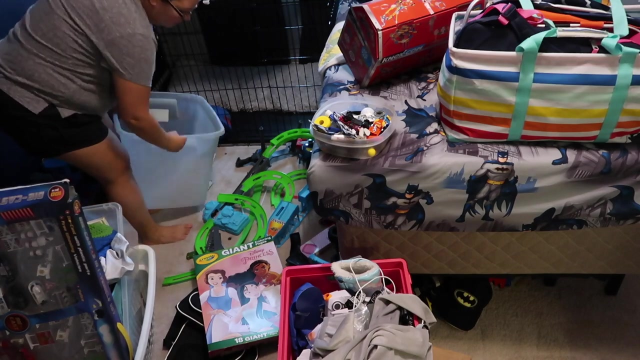 Why not? Why not? Cause I would like To have Some items. Never get it right without you. no, I don't wanna step into the light If I don't get you shawty. You bring out the sweetness of my life. oh yeah, Come on and give me that. give me that, give me that. 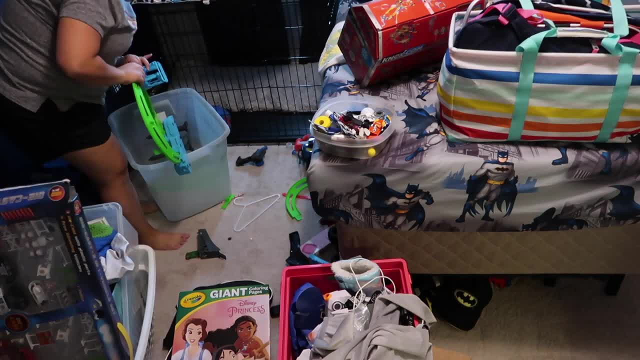 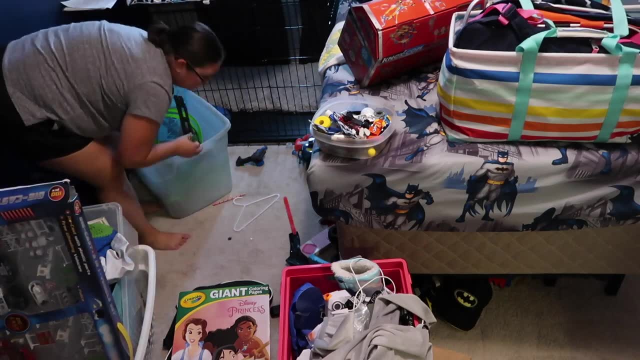 Good, good lovin'. Come on and show me that, show me that, show me that You're the one I move to the left while you move to the right, While you tryna fight. just Come on and give me that, give me that, give me that. 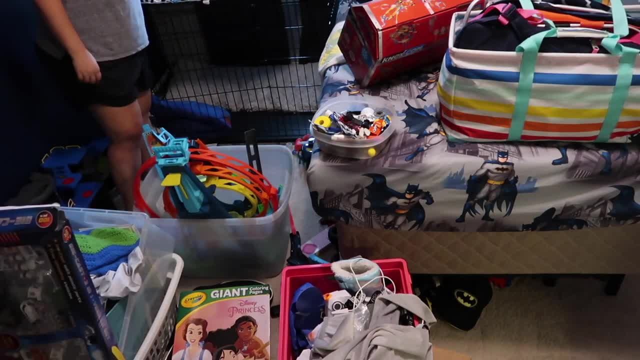 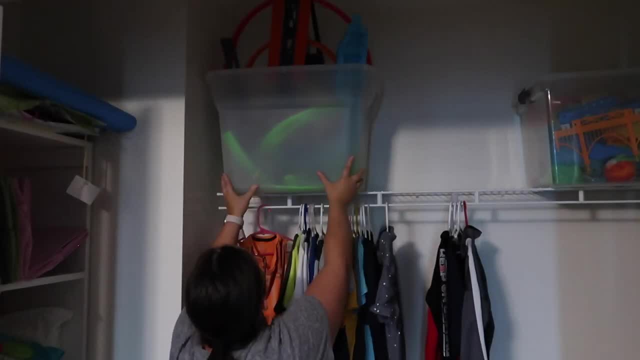 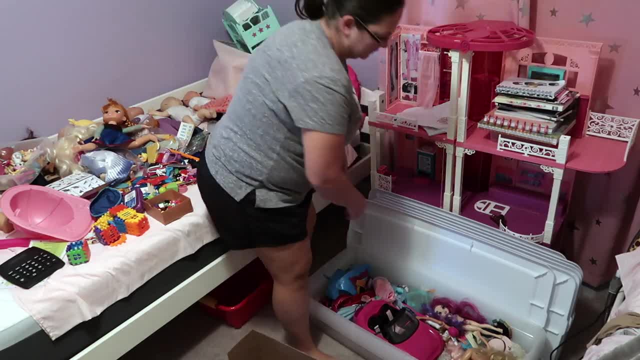 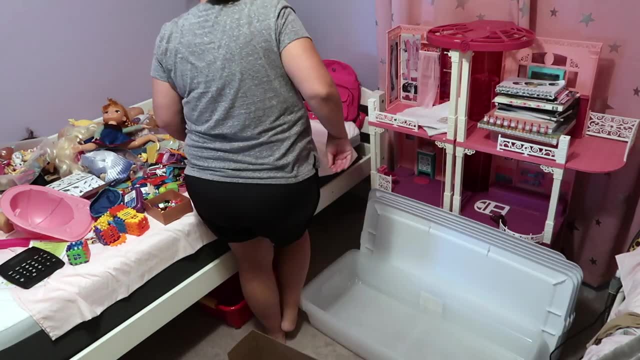 Wherever you go, I'll be there, you know. Don't be a stranger, don't be a ghost. Cause, baby, I love you. yeah, Guess, I'm gonna dance alone tonight. I'm gonna miss your body. You know I can never get it right. 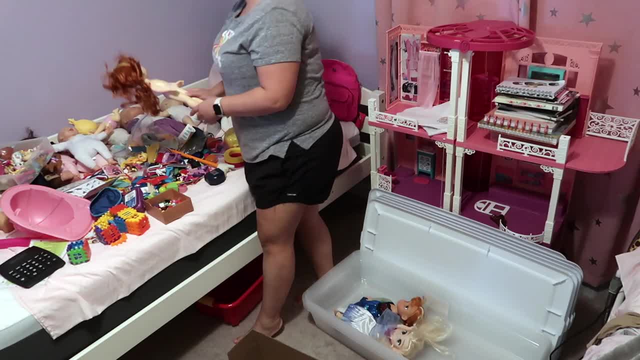 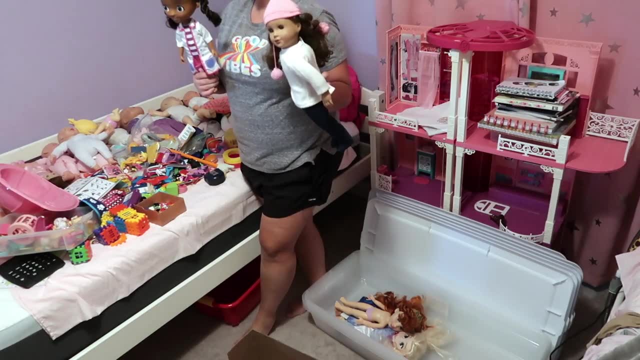 Without you. no, I don't wanna step into the light If I don't get you shawty. You bring out the sweetness of my life. oh yeah, Good, good, lovin', Come on and give me that, give me that, give me that. 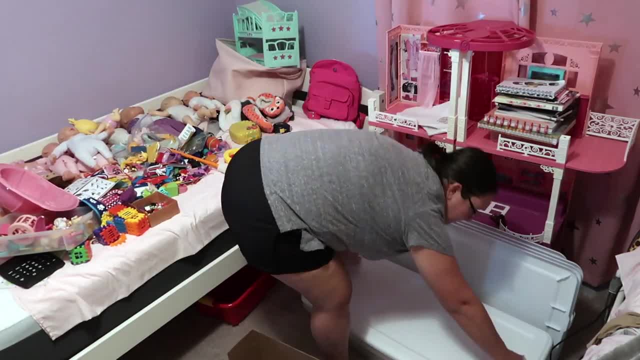 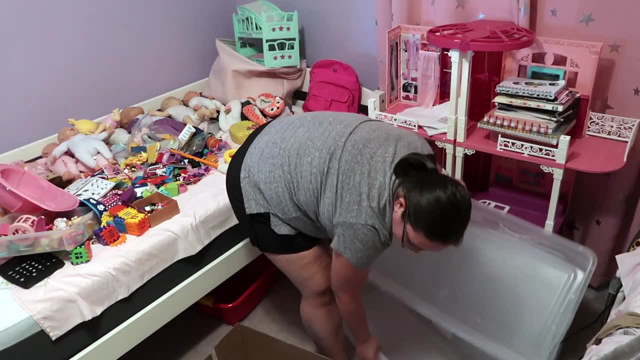 Good, good lovin'. Come on and show me that, show me that, show me that You're the one I Move it all up, while you move it right, While you tryna fight. just Come on and give me that, give me that. give me that. 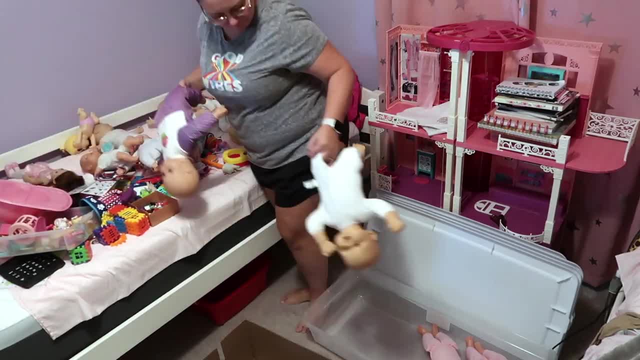 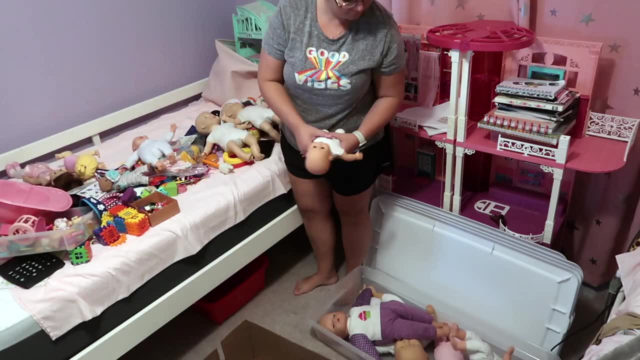 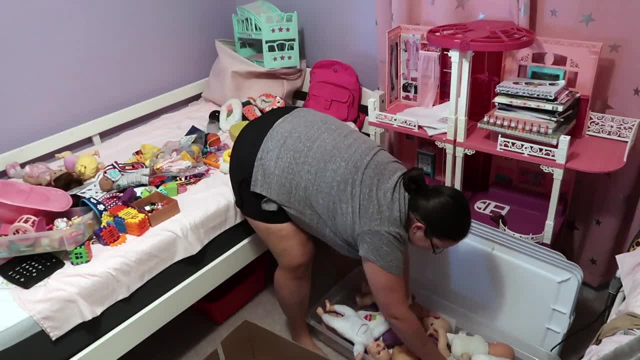 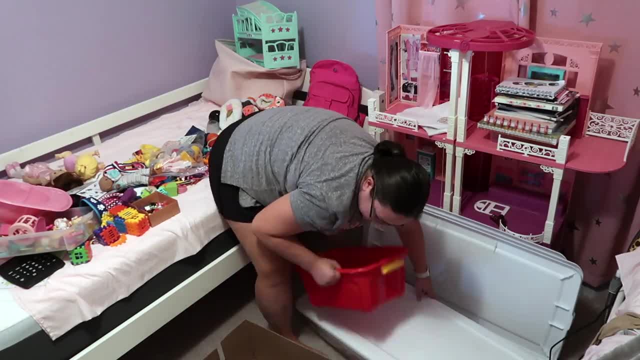 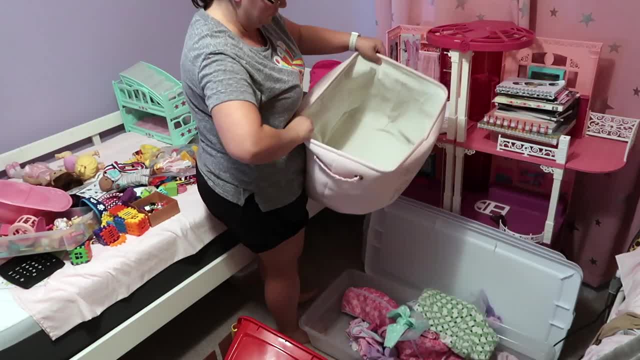 I don't feel right when you don't come home. I miss your body and I love you. so, Baby, I do, baby I do. oh yeah, Come on and give me that, give me that, give me that Good, good lovin'. Where you gonna leave when I need you the most. Wherever you go, I'll be there. you know, Don't be a stranger, don't be a ghost. Oh-oh-oh-oh-oh, I don't feel right when I dance alone. 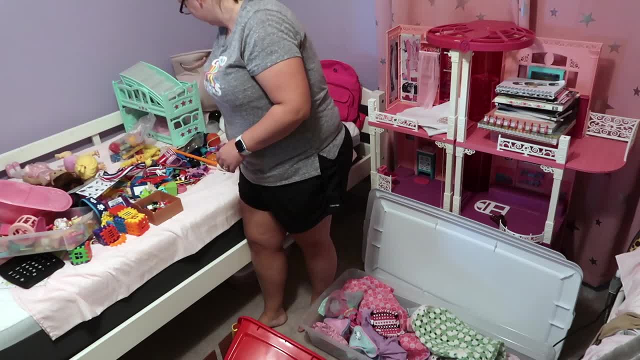 I don't feel right when you don't come home. I miss your body and I love you. so, Baby, I do, baby I do. oh yeah, Come on and give me that, give me that, give me that Good, good lovin'. 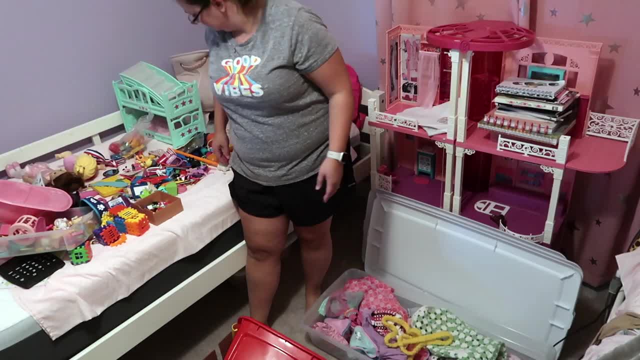 Where you gonna leave when I need you the most. Wherever you go, I'll be there. you know, Don't be a stranger, don't be a ghost. Oh-oh-oh-oh-oh-oh, I don't feel right when I dance alone. 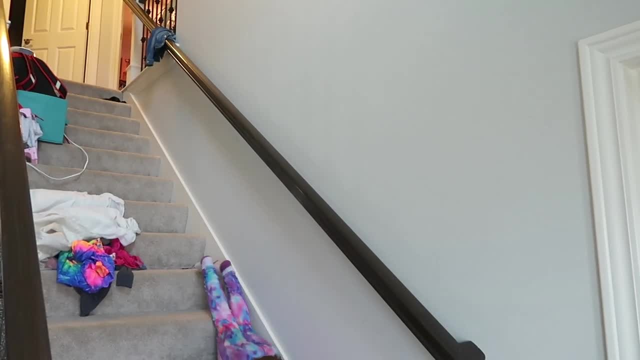 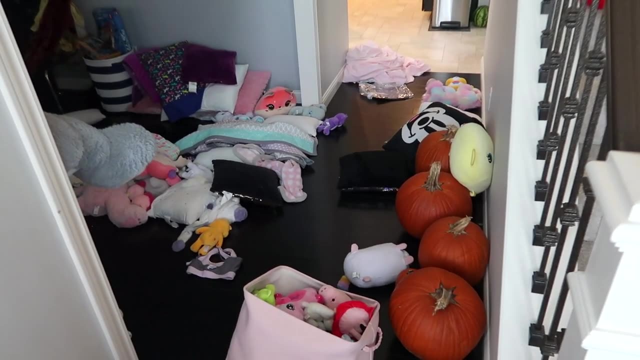 Baby I do, baby I do. oh yeah, Come on and give me that, give me that, give me that. This is what their feelings are about sorting through these stuffed animals over here. So then I brought down their bin of it and I looked over here and I realized there's. 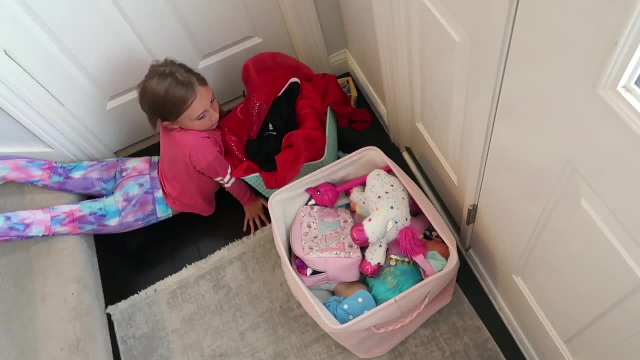 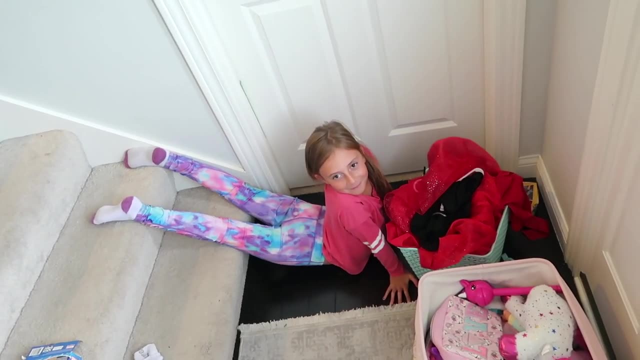 a couple more bins I haven't gone through. So we're gonna collect all the stuffed animals and then we are going to make some decisions. right, Brooklyn? Yep, Are you getting rid of stuff? Yep, You see that willingness behind those things. 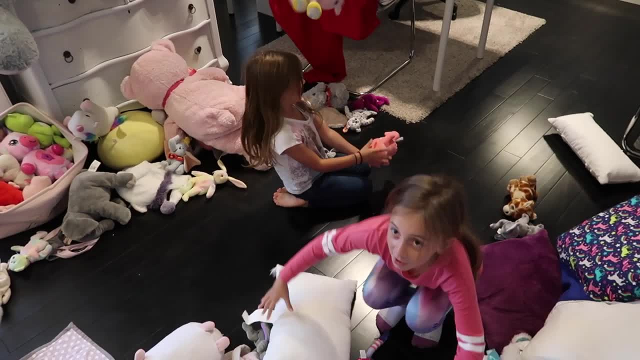 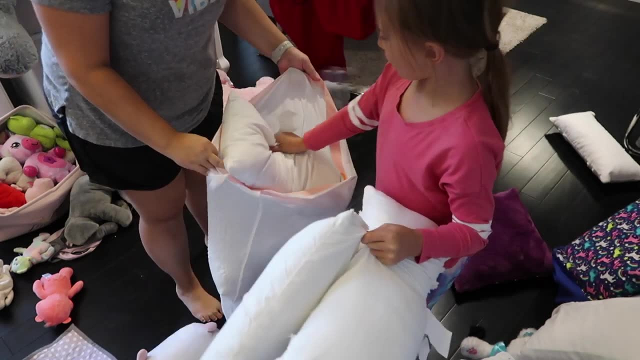 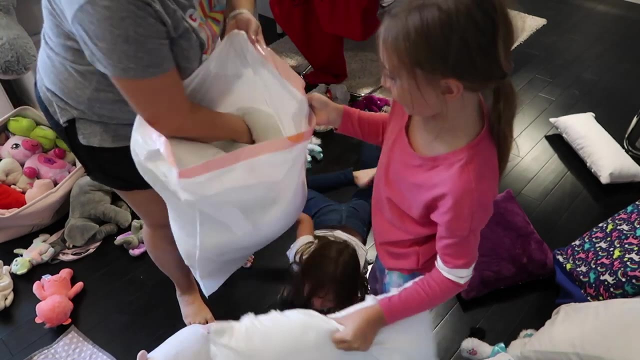 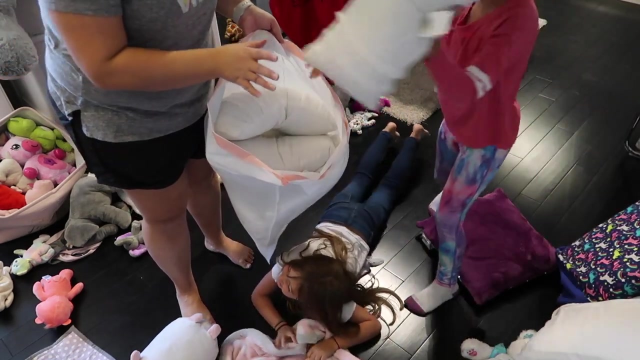 Those sweet eyes. Yeah, All right, these white pillows that came with their bedding are kind of just being extra monotonous right now. so there's one over there, Brooklyn. So these are just going to go in storage down in the basement until they're a little bit. 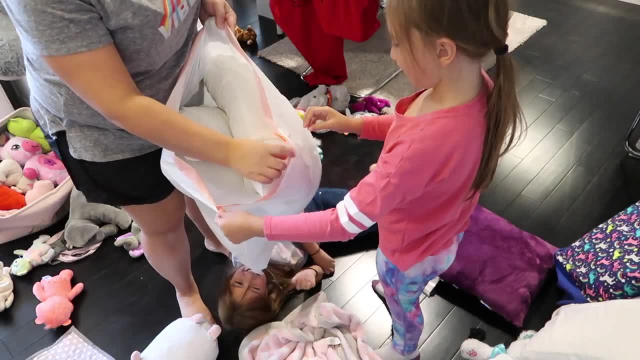 older and they like these pillows. Right now they'd rather have Squishmallows, Squishmallows, Squishmallows, Squishmallows, Squishmallows, Squishmallows and such All right sort me guys. 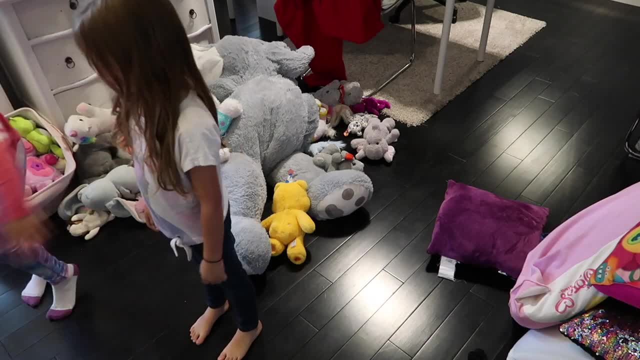 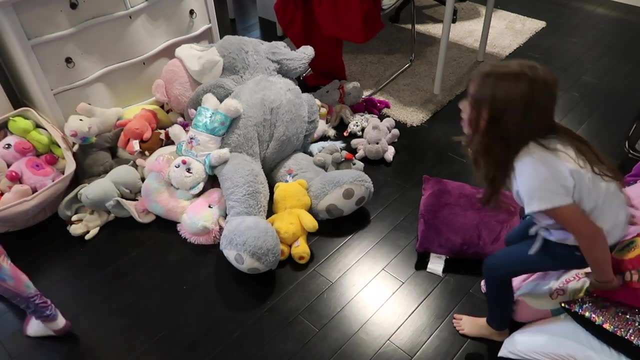 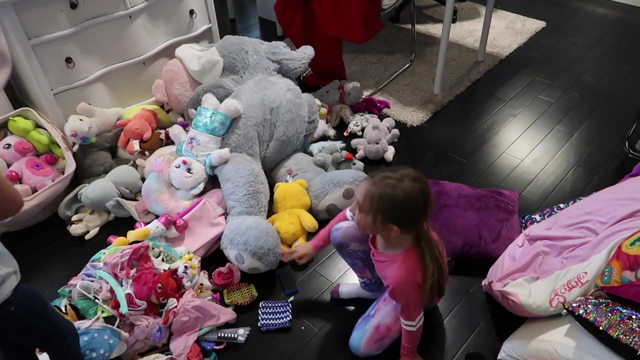 Might be that another day she would have wished he stayed, but the time's up. Well, we got more over here. y'all, Jump it up, Jump it up. I'm distracting right now. He's fine, But Lucy on the line, let's get this started. Where's the party tonight? 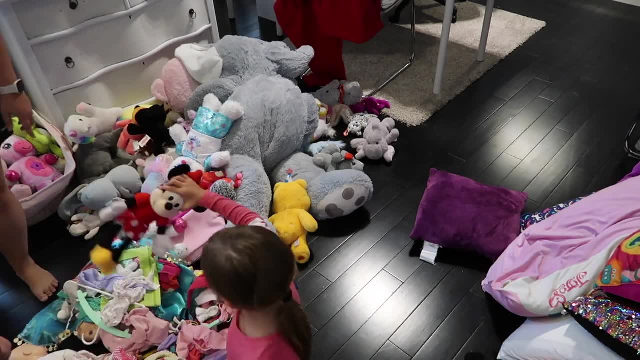 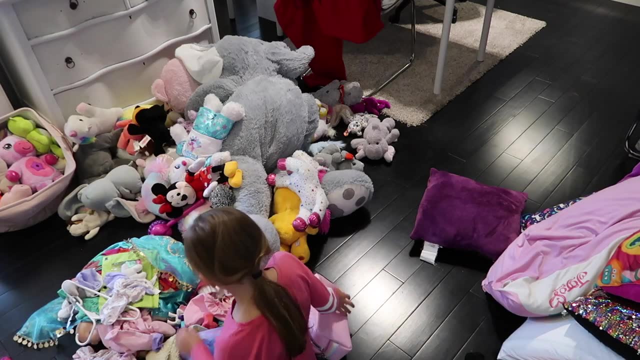 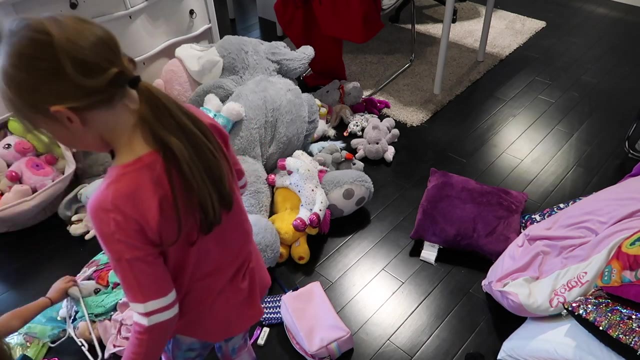 I feel good. Nothing weighs me down. I can't believe my love right now. Red eyes, while he said: don't you want to have fun? Fool around with someone? Don't you want to have fun? Never mind my dumb heart, It needs a little kickstart. 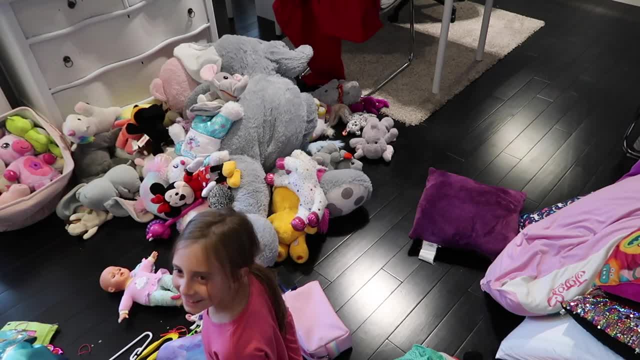 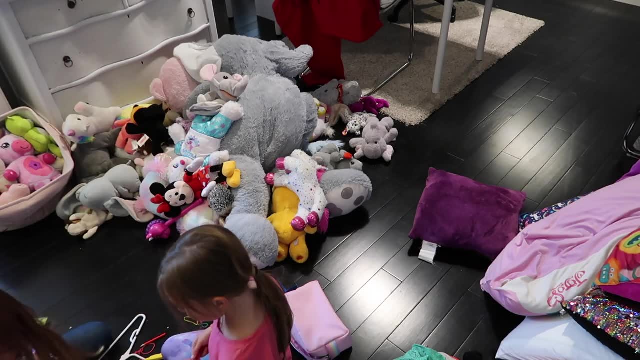 Don't you want to have fun? Don't you want to have some fun? Don't you want to have some fun? Don't you want to have some fun? Ooh, who needs a job to pay the rent? He's busy. Gotta feel free sometimes. 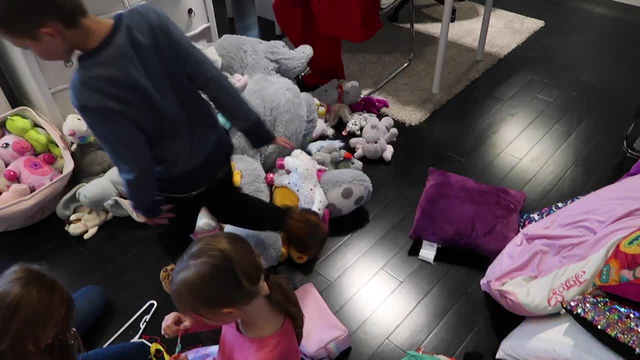 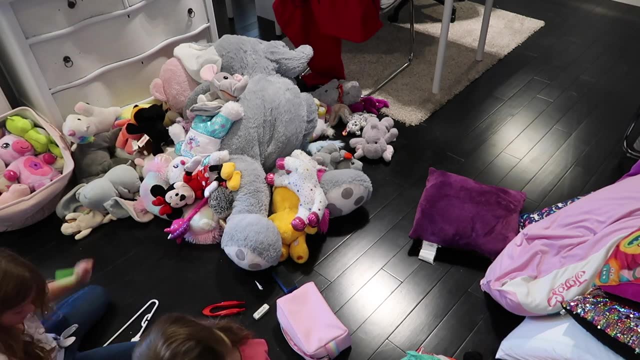 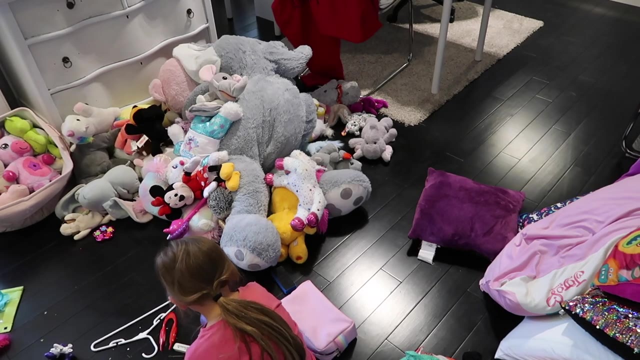 But what does it make you? It'll only make you stronger if you believe what they say. Maybe that another day she would have wished he stayed, but they're done. Red eyes, while he said: don't you want to have fun? Fool around with someone. 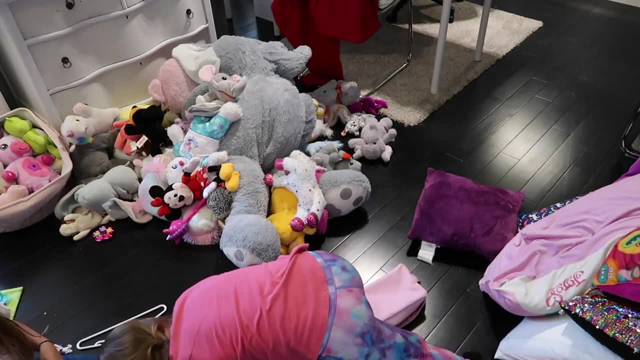 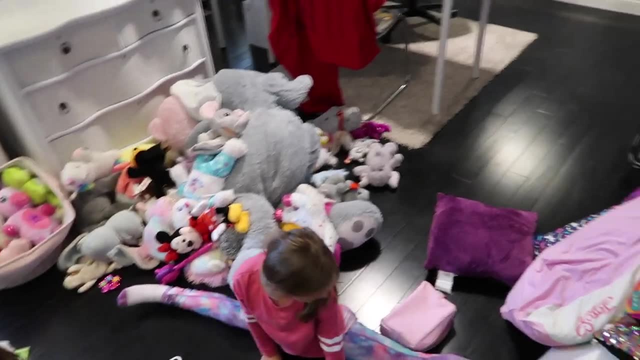 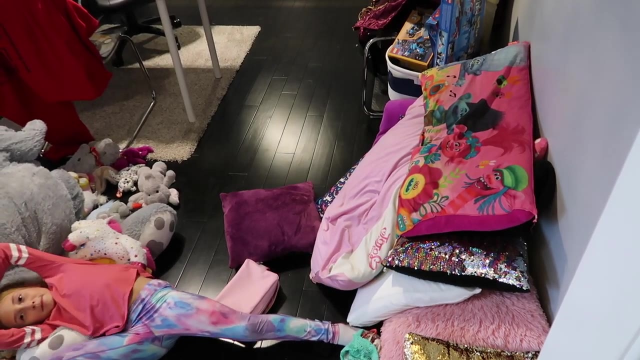 Red eyes while he said: don't you want to have fun? Red eyes while he said: don't you want to have some fun? Red eyes while he said: don't you want to have some fun? Alright, so get your kids involved. We have over here is a pile of pillows that we're gonna go through, because those pillows are for two girls. 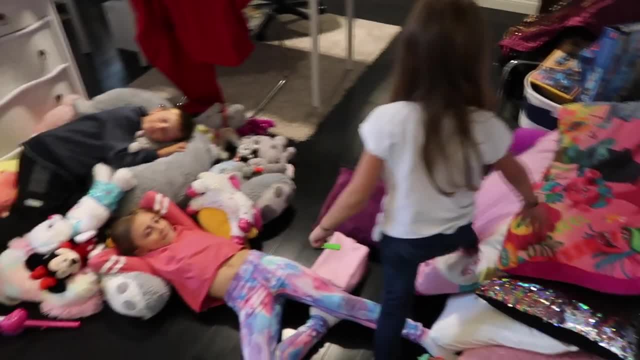 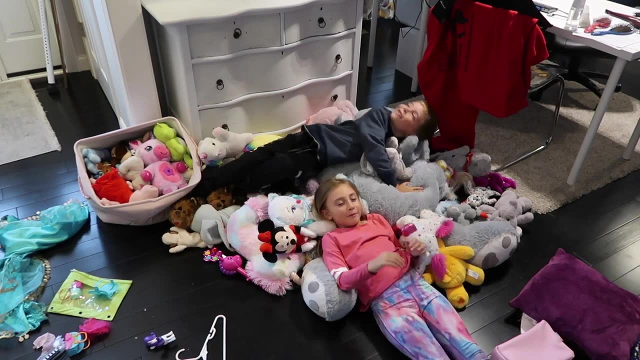 And I'm pretty sure there's more pillows that aren't right here. Then underneath the twins over here and this basket right here is all their stuffed animals, Red eyes. while he said, don't you want to have fun, lies the issue in their room is stuffed animals. none of my kids were big stuffed animal kids. 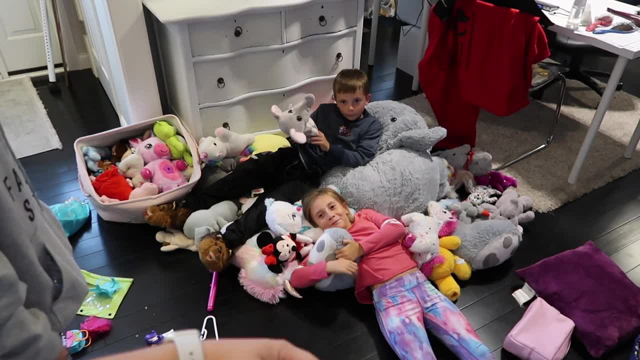 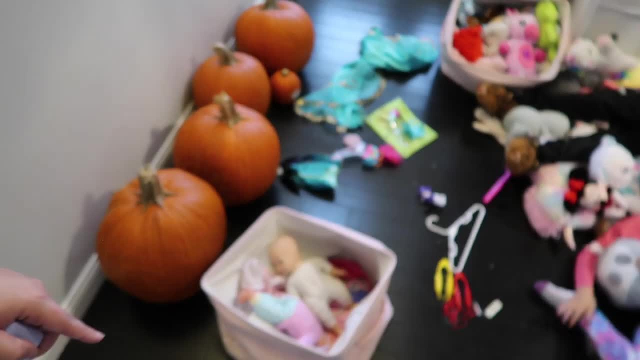 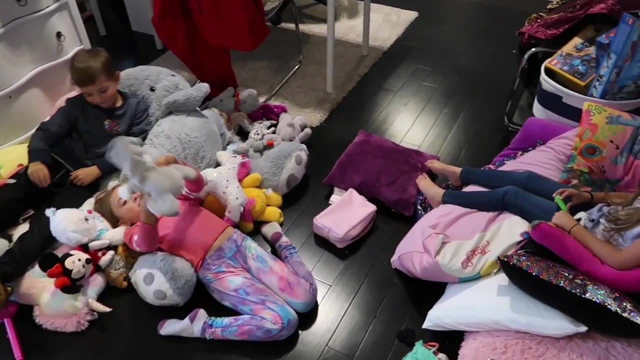 until brooklyn, right here. and then kenzie that almost six or just turned six year old, um, and then we have some baby doll and barbie doll stuff here that we're going to consolidate with the stuff upstairs. so we are going to start probably at the pillows and get rid of some of this stuff. 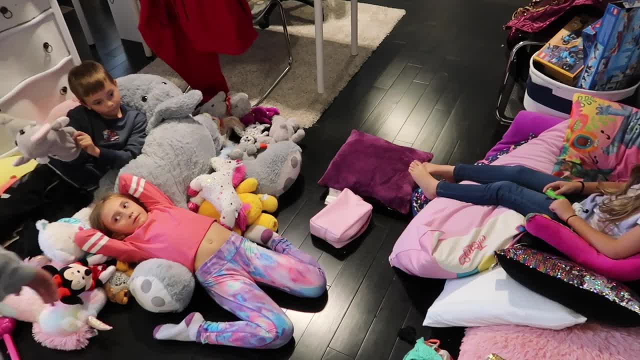 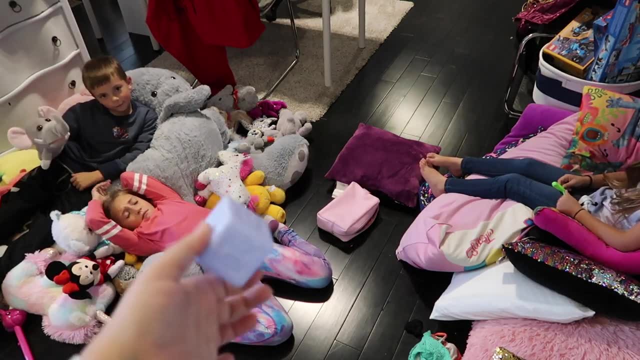 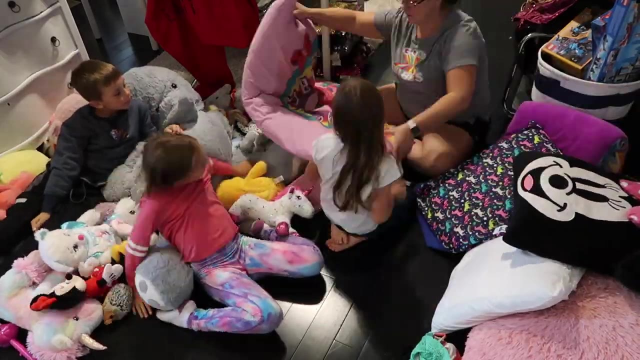 because they can't even lay in their beds, because between the pillows and the stuffed animals it's just too much all the time. all right, we're getting rid of this, because their baby dolls don't play with a block. so i can't let you go, baby. i just want to tell you that. 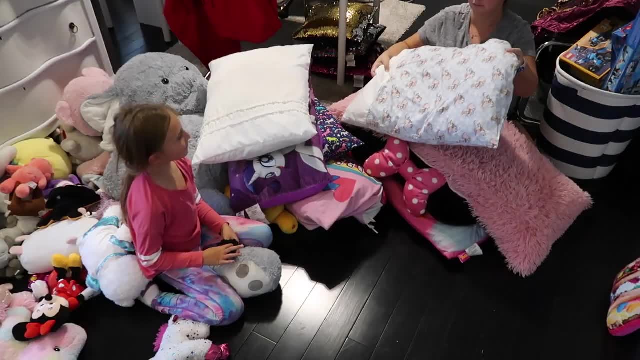 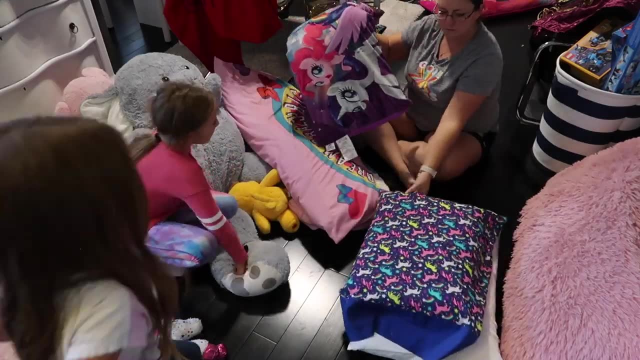 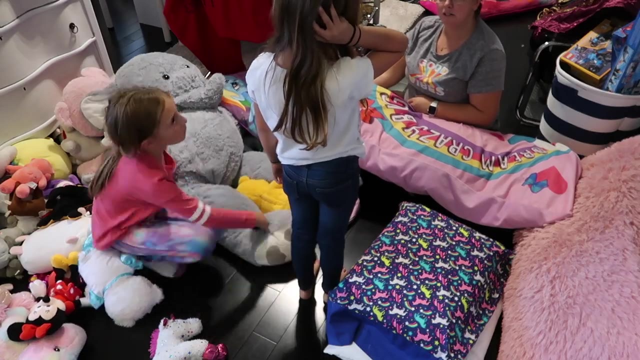 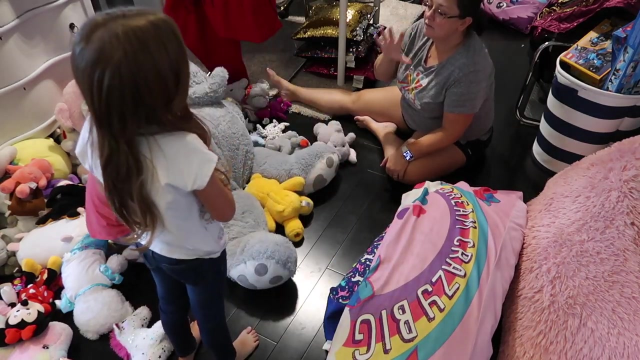 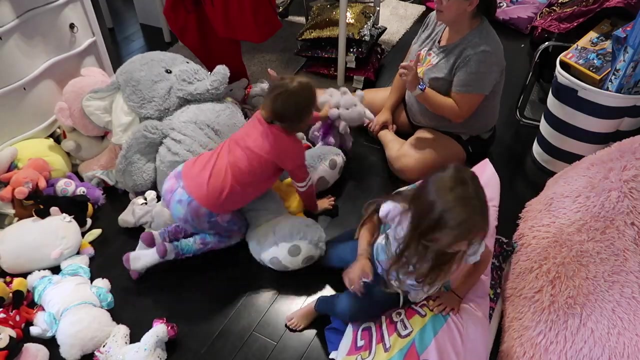 no, no, no. all of my friends say: girl, you better take care because that man is trouble. you best beware and hold it down. i know i might be headed for teardrops now that you got me started. i just can't stop. no, because i love you, baby. i can't let you go, baby. 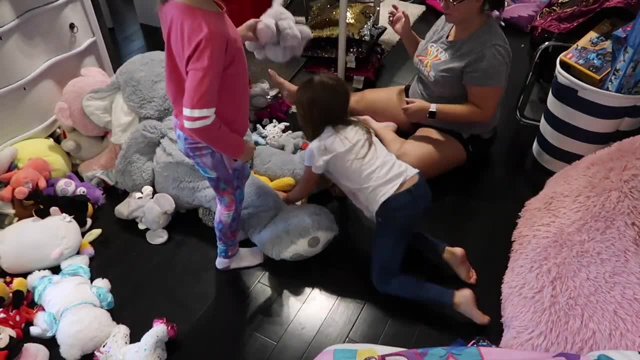 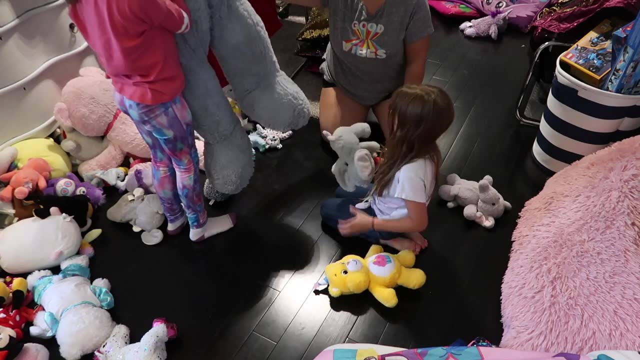 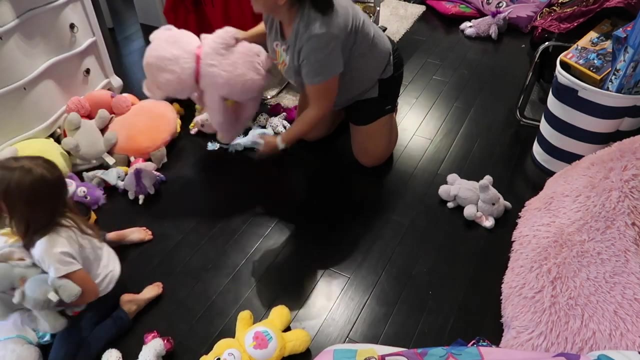 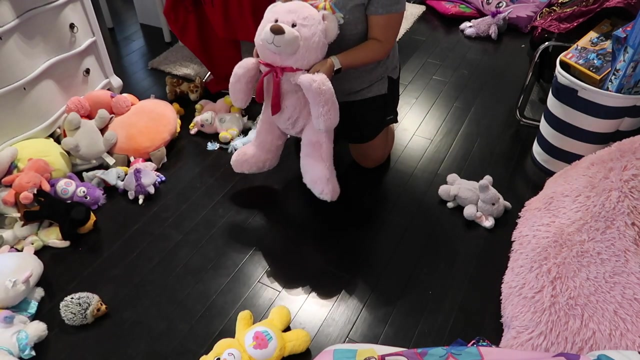 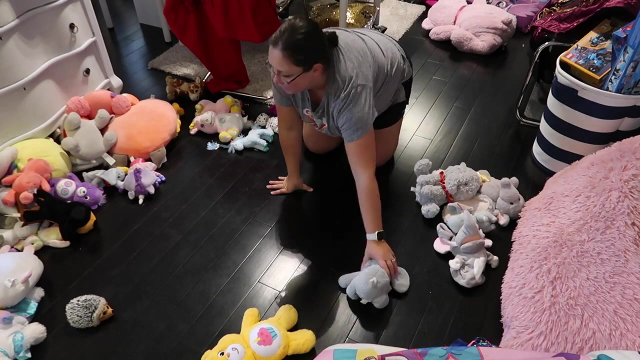 i gotta tell you, let's one up all the dumb blows. okay, all right, this one has an obvious key. if you could put it over on the stairs down and down, along came you- though you might be alive, i'm pretty sure. this dead guy. i can't let you go baby. i can't let you go baby because i love you, i love you, i love you. 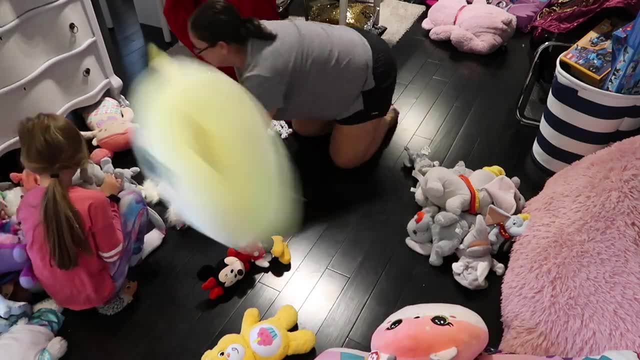 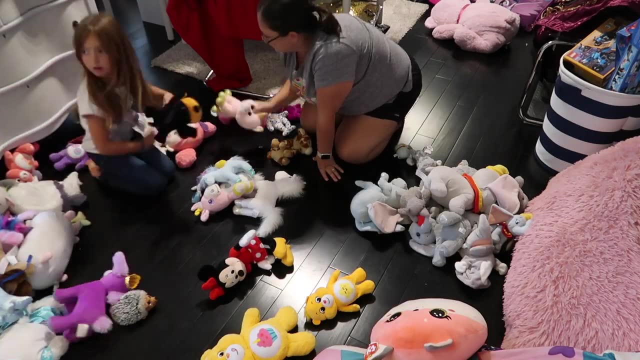 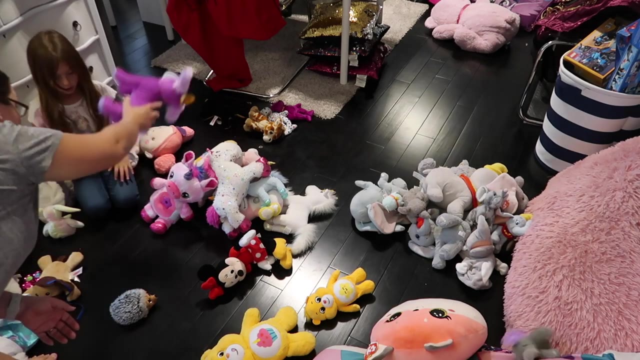 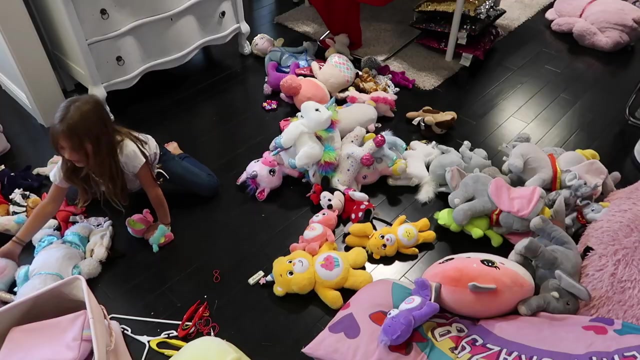 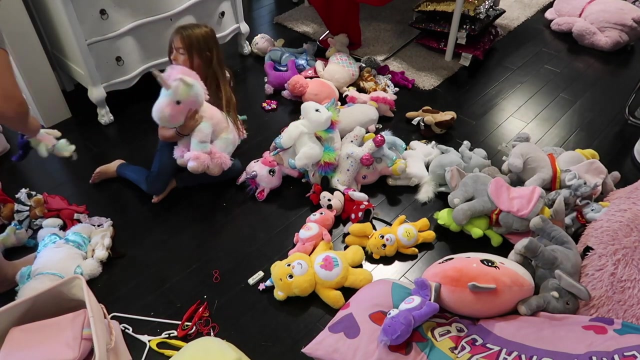 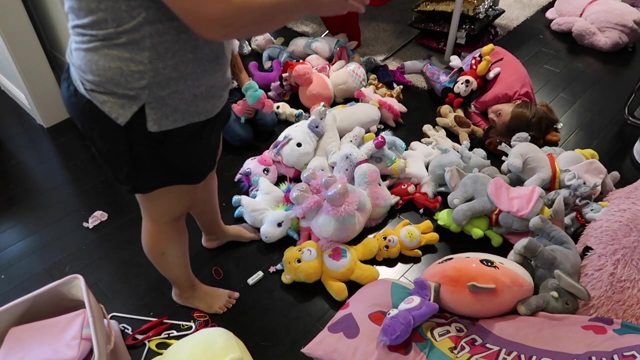 we may have a dumbo issue. all right, it's almost eat time, so let's finish getting them off 13. nine, what are we having? can you eat this hat i have put in to donate like five times. they need to stay and donate, all right. so this is kind of humorous and this is exactly why you. 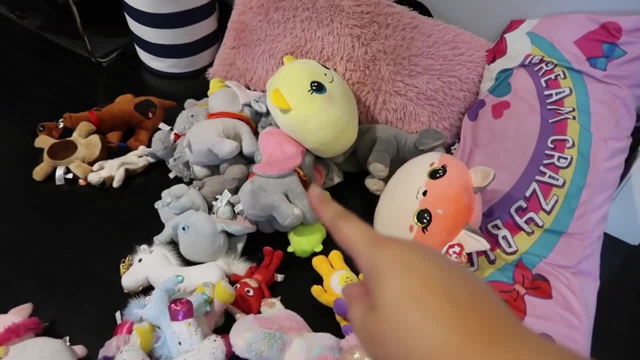 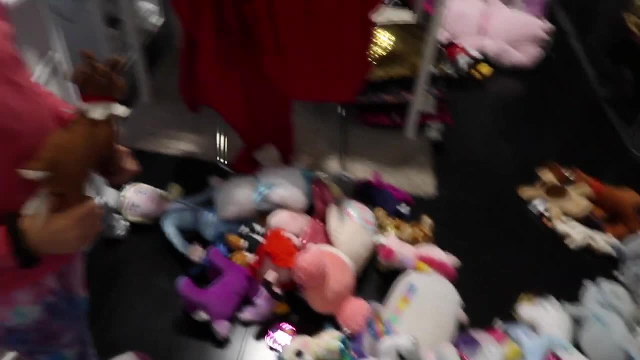 make piles like this. so this is our dumbo pile. those squishmallows will be keep. they're kind of like pillows. we've got a few care bears here and here. i thought this one was the one who absolutely loved stuffed animals, but i think it's my success. i think it's my success. i think it's my success. 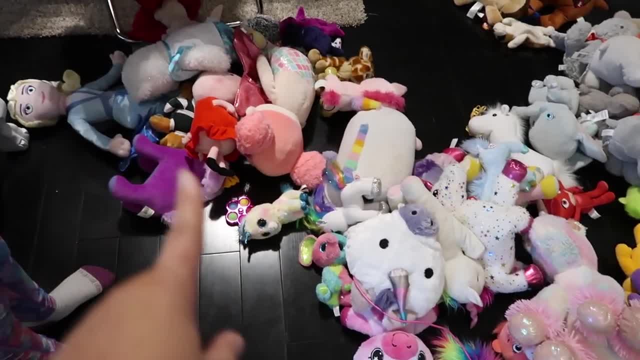 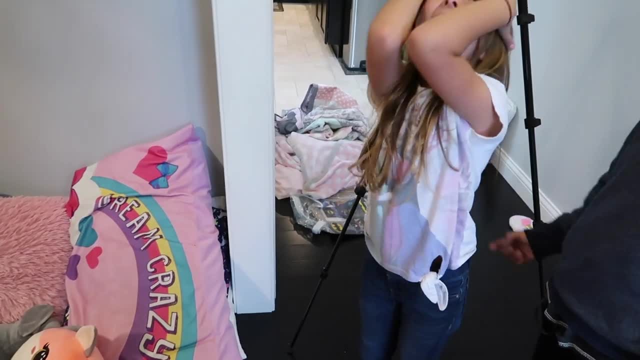 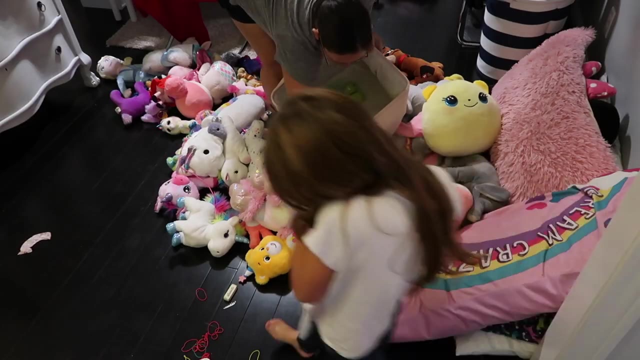 year old. look at all these unicorns and then all these extras. so i'm pretty sure she's gonna be having a few hard decisions to be made. yeah, you have to get rid of all. right, we need to go switch laundry and eat supper and then we'll come back to you. can't tell me to let go, baby, cause i love you. 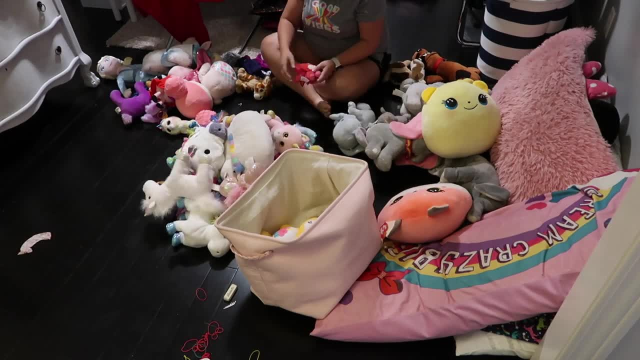 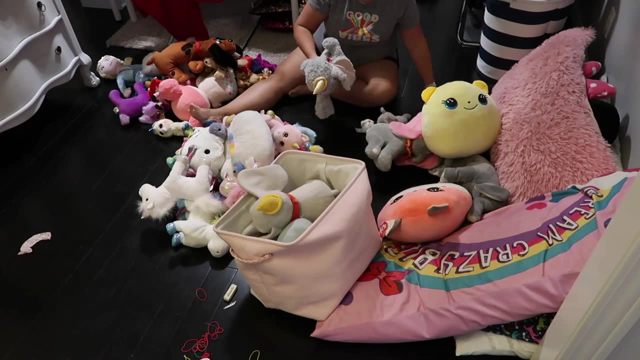 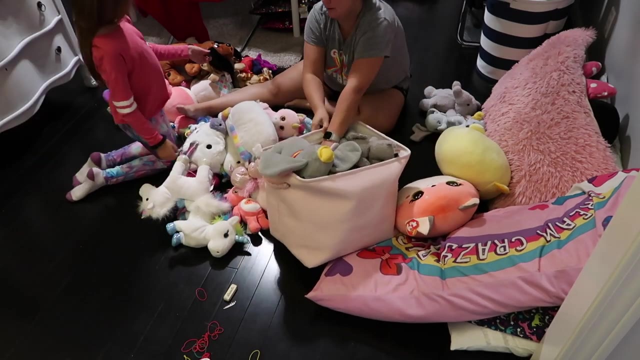 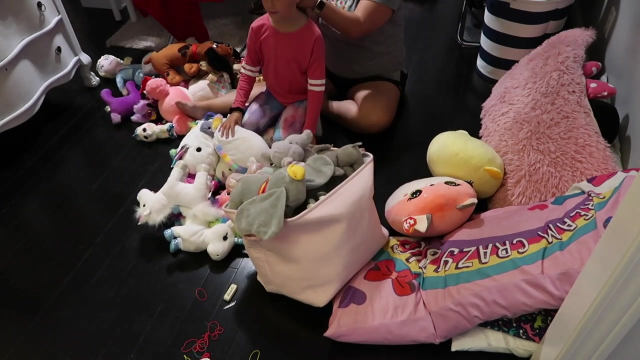 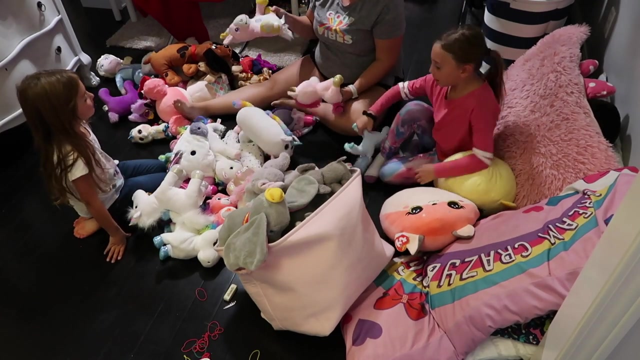 i love you. yeah, cause i love you. yeah, i don't wanna be the girl, but i kind of need a word. well, i'm into you and all i know. it's been a long time. i was on the sideline waiting for you. we could go to california or any way you wanna. as long as i'm with you, i'm all right and we don't need the drama. 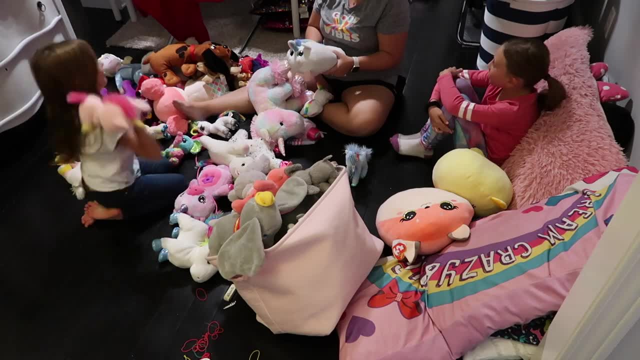 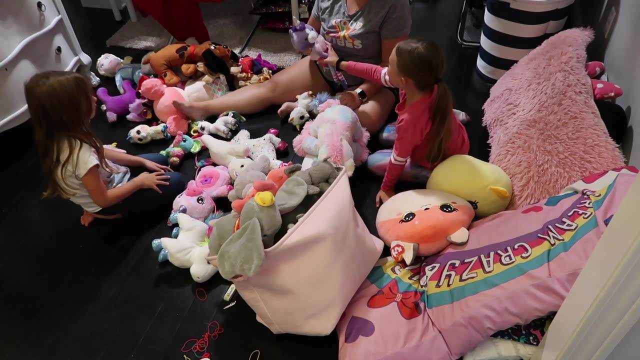 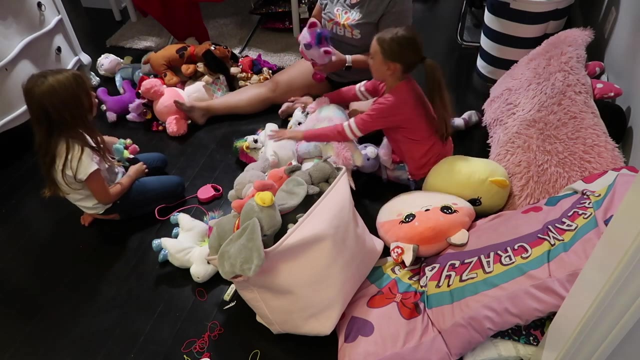 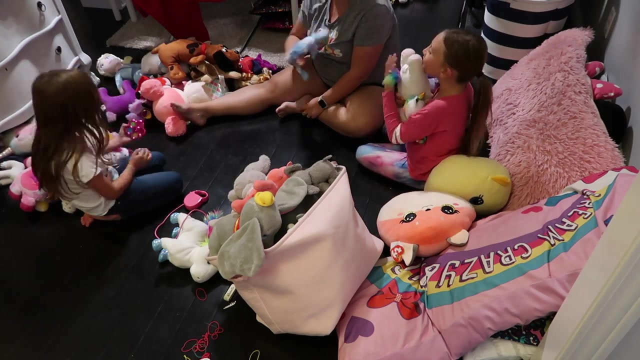 we'll find our own nirvana. so run away with me tonight, cause it feels like i'm dreaming when i'm waking up next to you and my world's heart is beating because it's beating next to you. all right, we didn't make much progress here. this is still an excessive amount of stuffed animals. 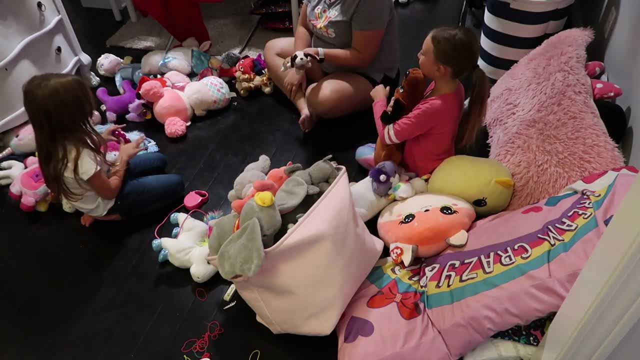 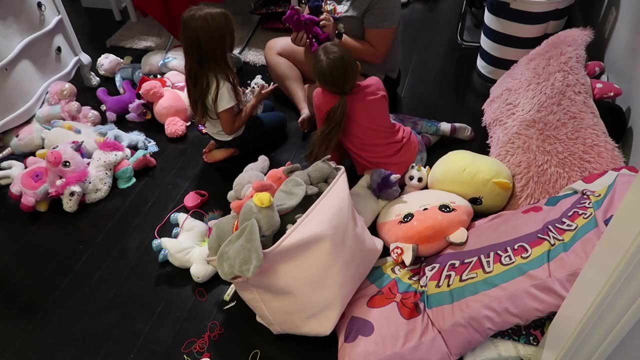 we are going to try to put them decoratively, like around their bookcase and stuff like that, and see how we can get it to fit. they're only allowed five in their bed and then we'll kind of go from there. it is my fault, like all the dumbos i just said. 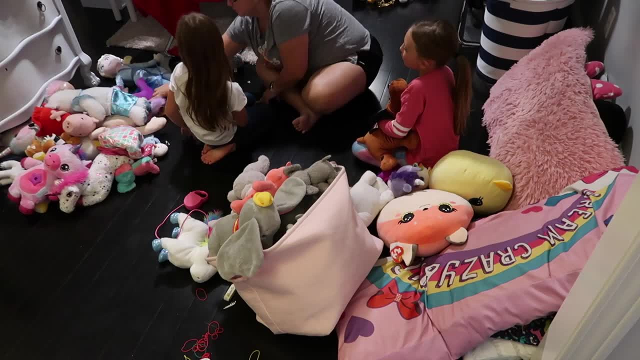 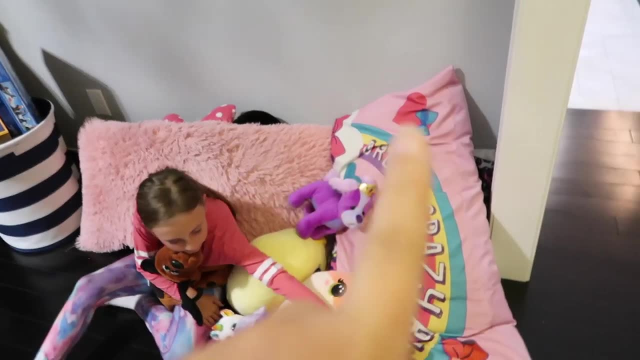 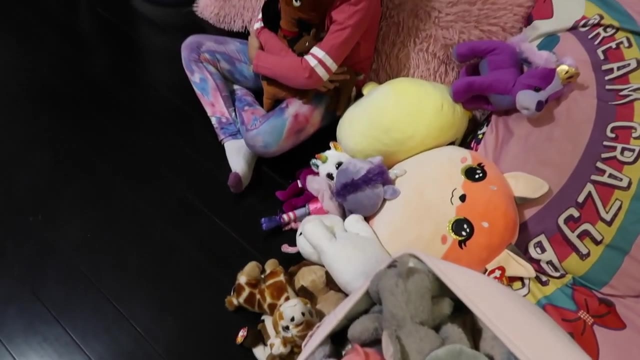 all we're keeping and stuff like that. but um, yeah, let's, let's see how we can get the room finished. all right, so all these are pillows. this pile is kenzie's, that pile is brooklyn's. this is mostly dumbos and some care bears. this is brooklyn's little pile. 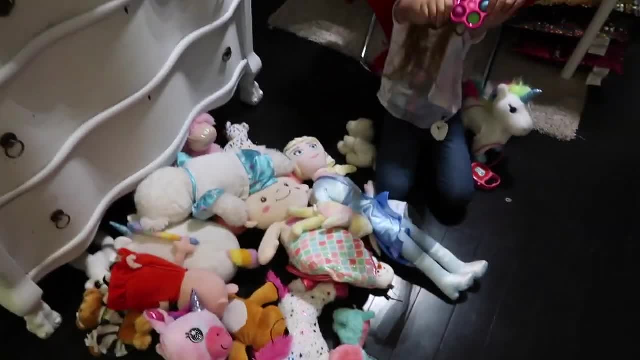 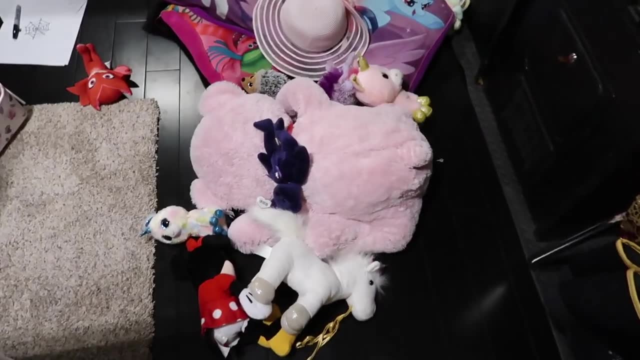 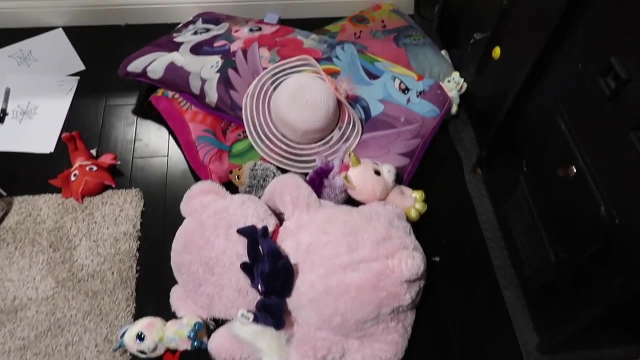 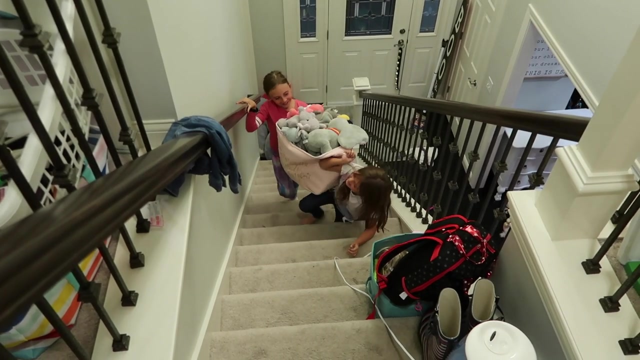 of um, stuffed animals- and this is kenzie's, so kenzie has a crap load. and then over here, i mean we got rid of a decent amount. it's not too bad by any means. um, that's like a whole entire trash bag full right there. so, all right, we're gonna get some stuff taken upstairs. 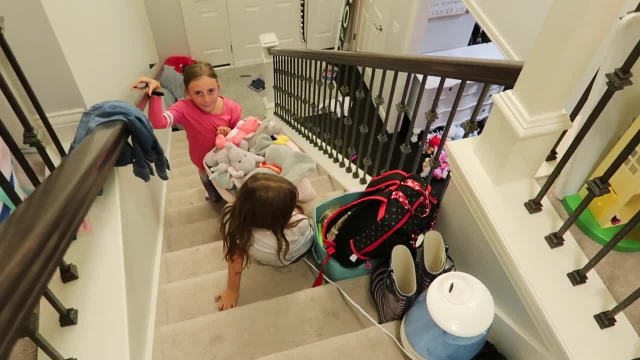 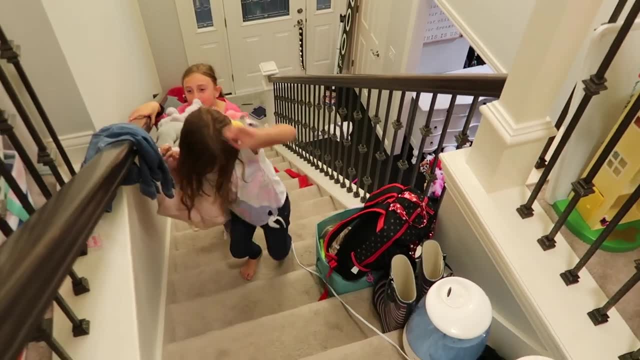 I just found right next to where Kenzie just sat. I'm pretty sure that's a whole entire bin of Barbies, but I do think we have enough room in the storage bin for it, so we'll keep going. All right, full thing of Barbies. 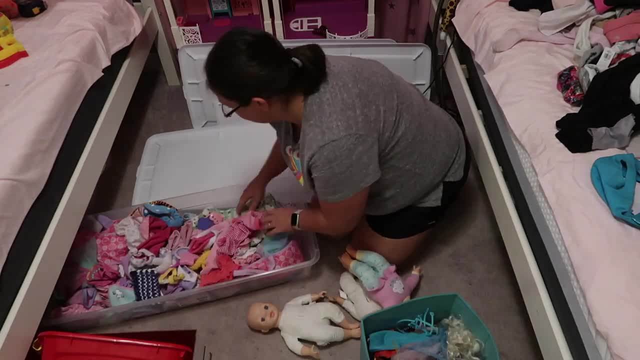 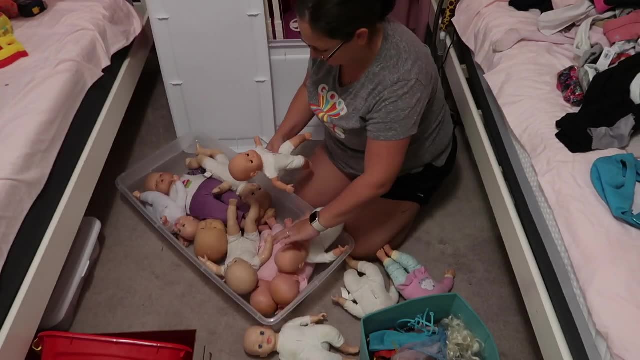 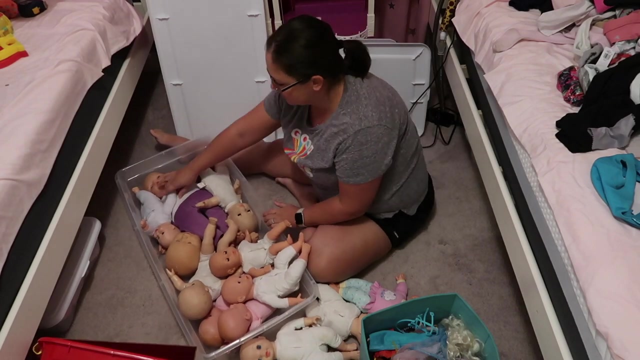 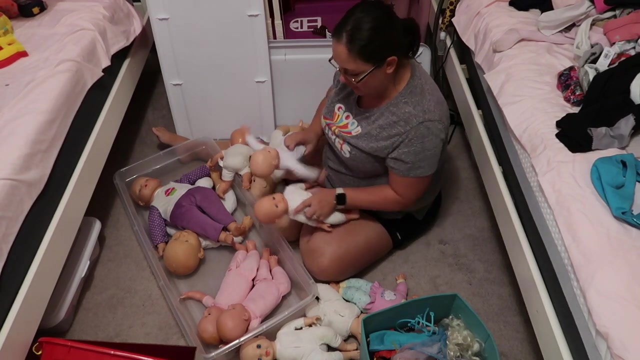 Most of these are looking the same at this point, so let's get rid of a few of them. All right, they like these two big ones, They like these twin ones, and then I feel like Queen, Queen. Okay, Those two are not the twins. 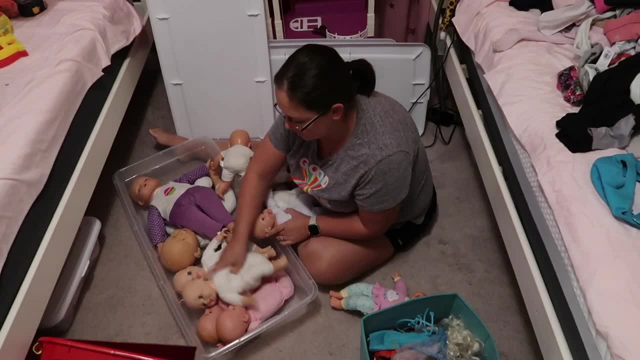 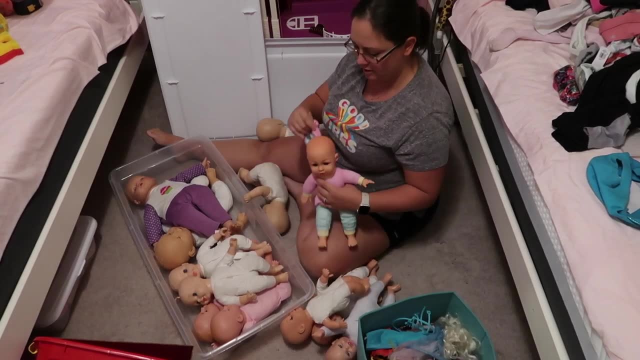 These two are more twins, so they like twin babies. None of these are matching, Don't we have a matching one to this? Yeah, a purple one, Where is it? All right then. these two are bigger ones, but they need their faces washed. 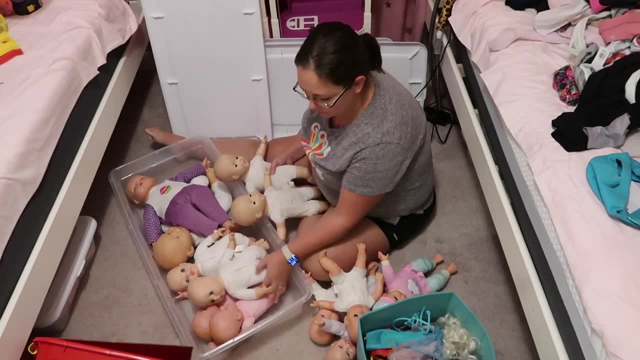 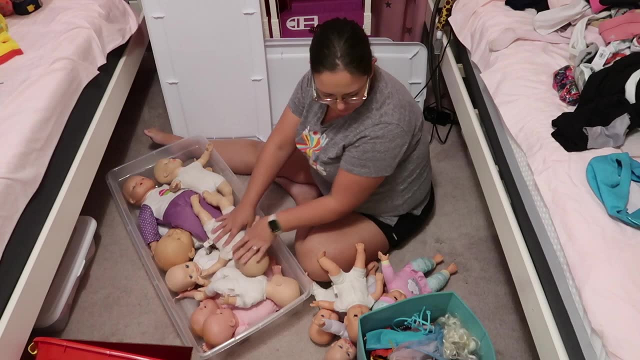 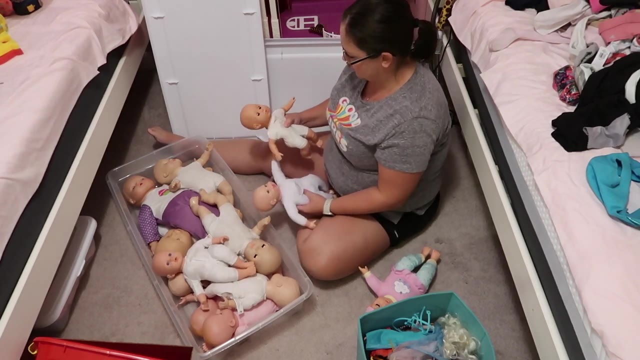 but they do like the size, whereas I feel like these ones are the same size. so keep Two of these Two bigger ones, and then I feel like we can get rid of those two and keep this one. Like I said when my kids play dolls. 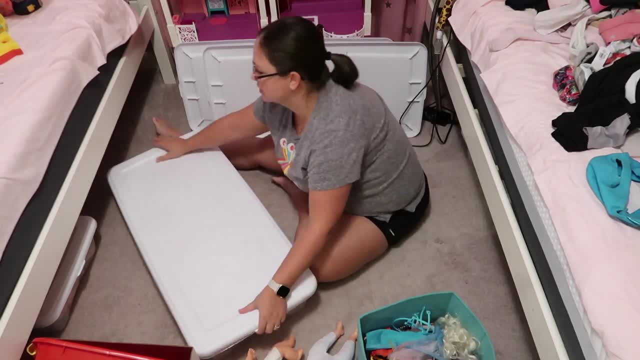 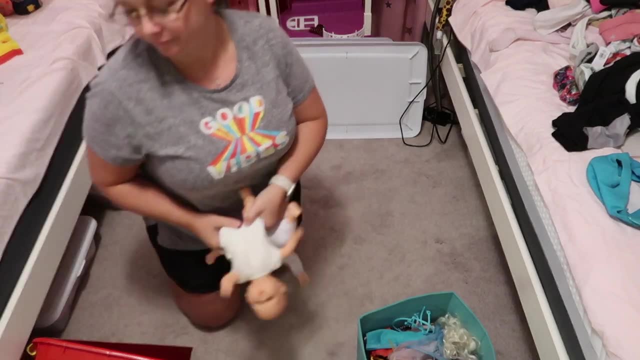 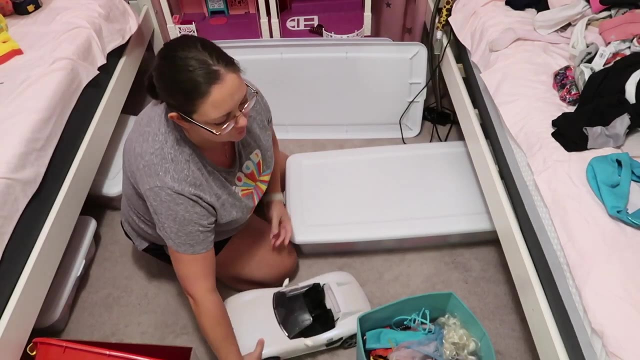 all four of them play together, so they do use a lot of dolls. They like to play daycare and stuff like that. So these two are going All right. now we have Barbie dolls and LOL And Rainbow High, So we might have to take this car out. 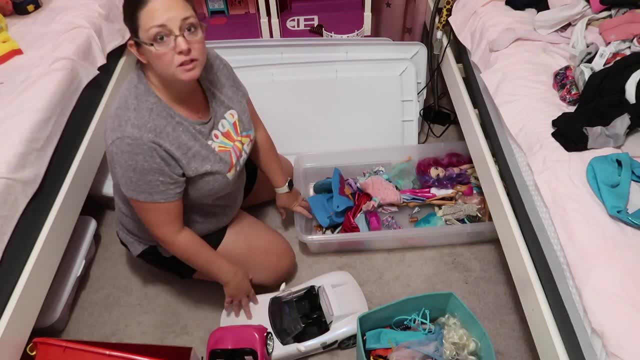 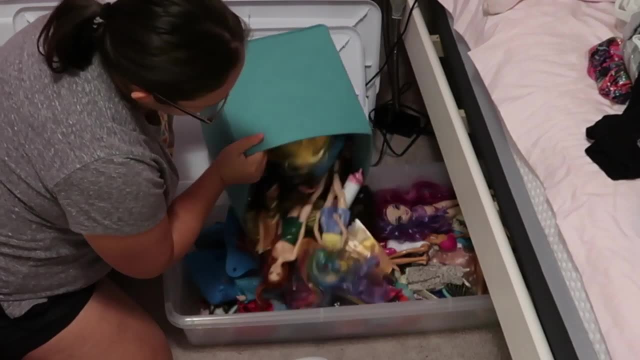 I'm going to let them have both cars, because this is a Barbie car and this one's a Rainbow High car and this one lights up, so it's really cool. All this is already sorted. Okay, Okay, Okay, Okay. 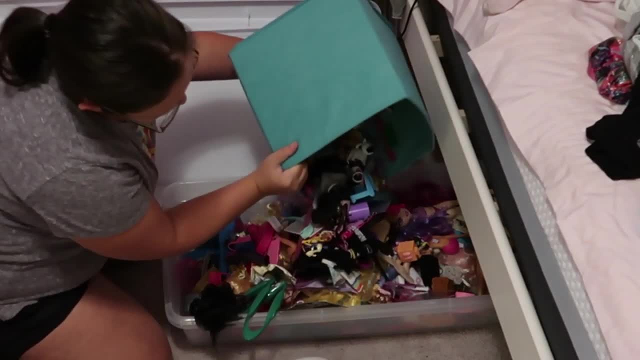 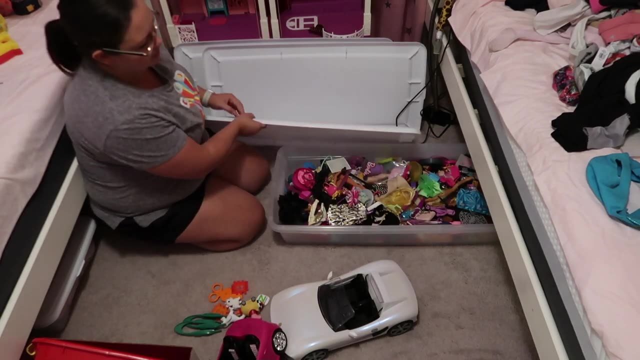 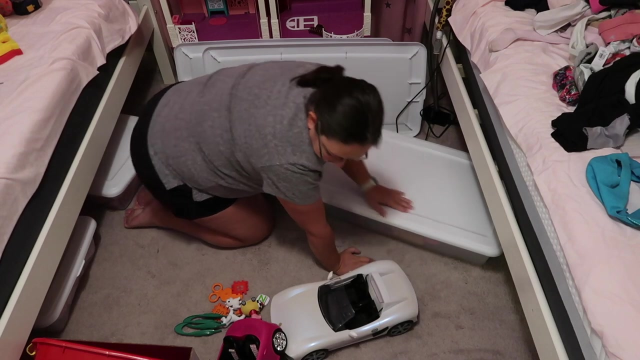 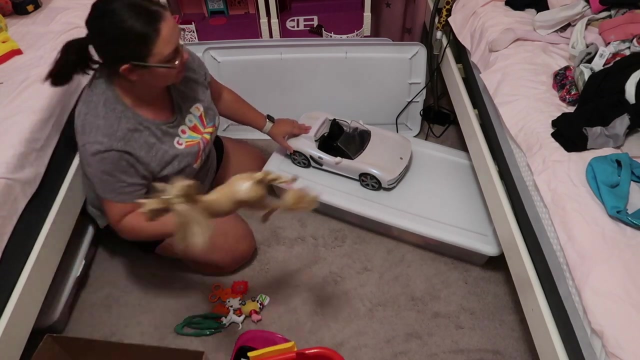 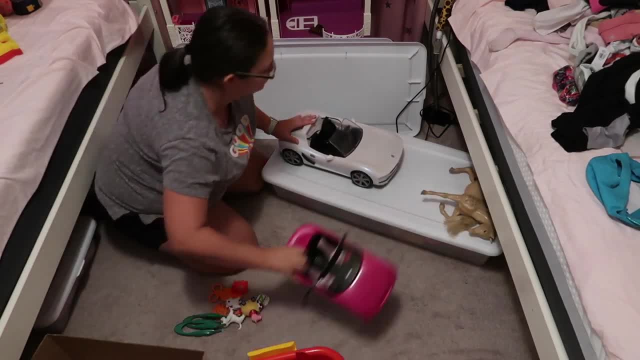 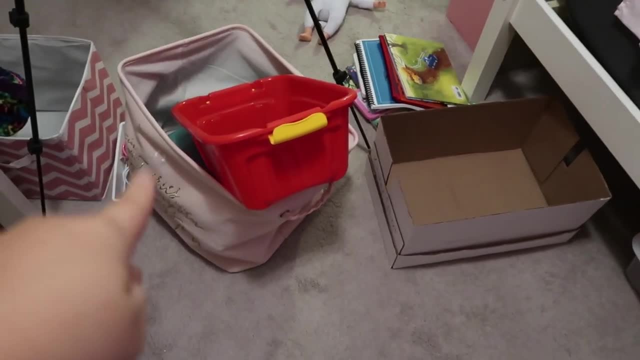 I feel fine about that amount. It all fits in here and it'll go underneath the bed. And then they have this Barbie horse that won't fit in there, and this, Alright, back under. If I turn you guys around, we just emptied quite a few bins. 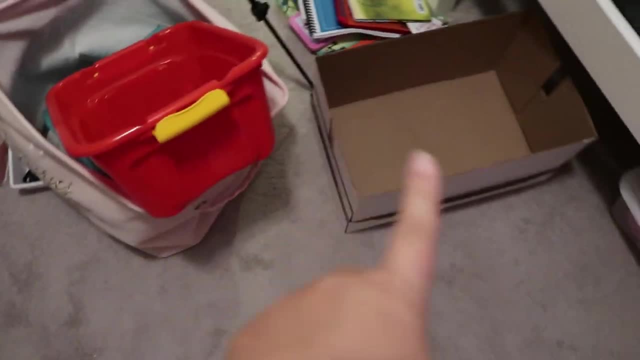 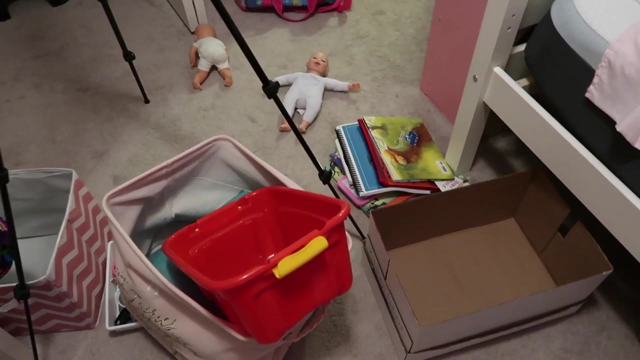 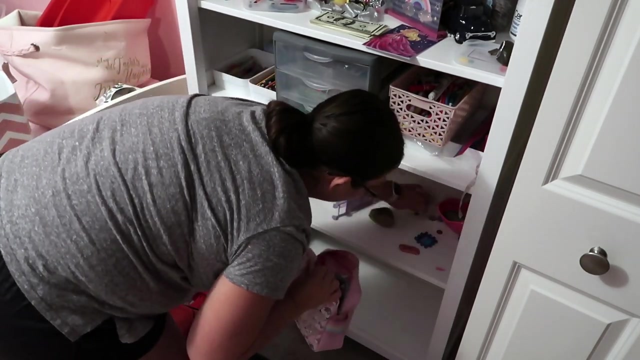 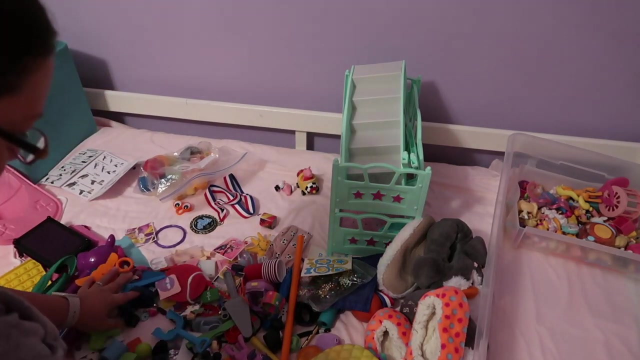 There's a bin inside here, inside here, there, and then this one, so quite a few bins done. gotta put those two dolls out in donation. love is like a roller coaster, but i'm trying to hold on. i don't want it to stop. even though we fight sometimes and it feels like a war zone, i still care about us. how do you move? 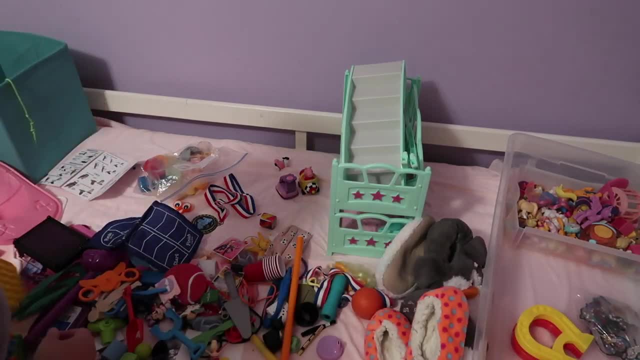 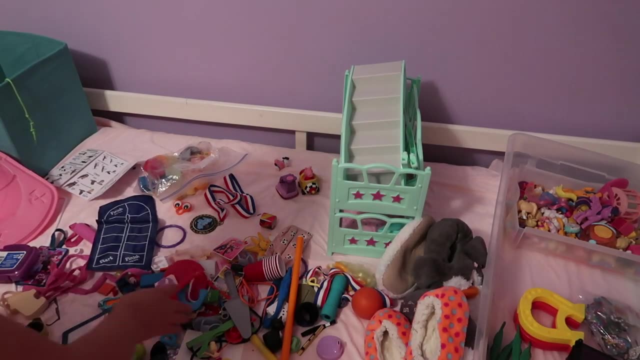 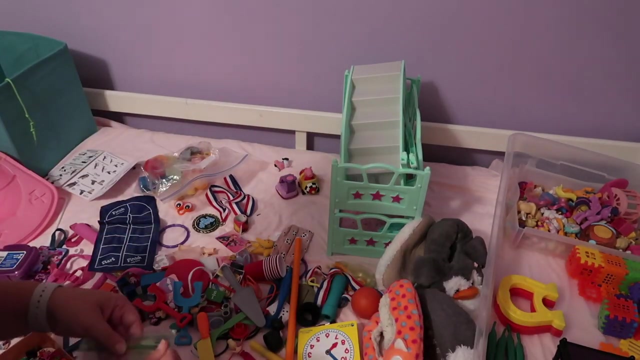 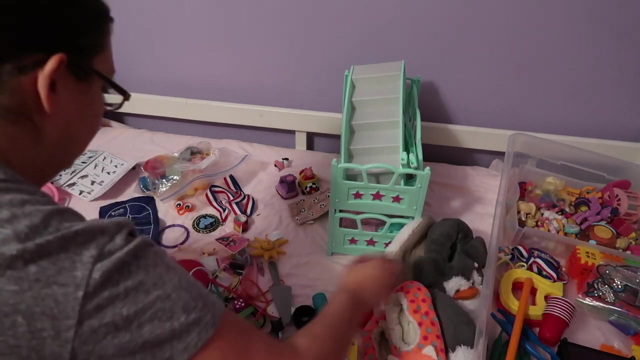 on when everything goes wrong. i'm trying to find a way to get you out my head. don't know how to cope with being so broken girl. i can't forget about what we said. i just wanna love you a little bit more. don't just walk away from me and close the door. baby, pull me closer now, before it's over. 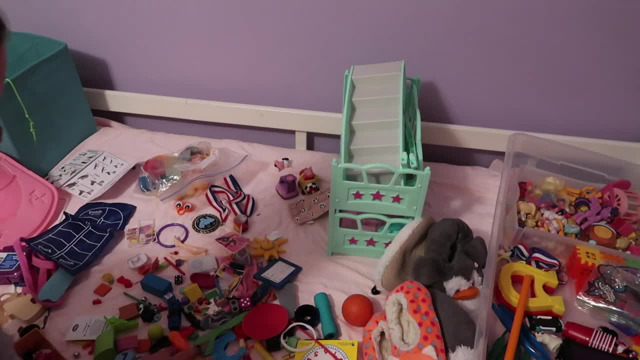 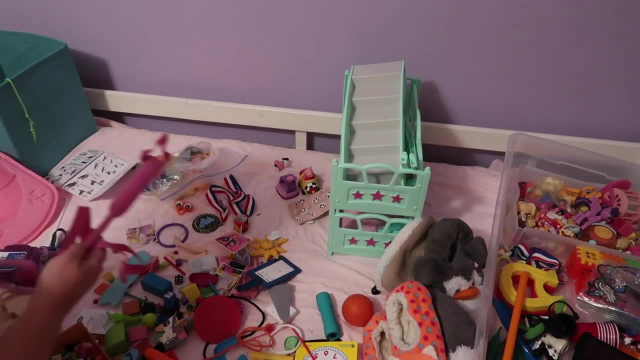 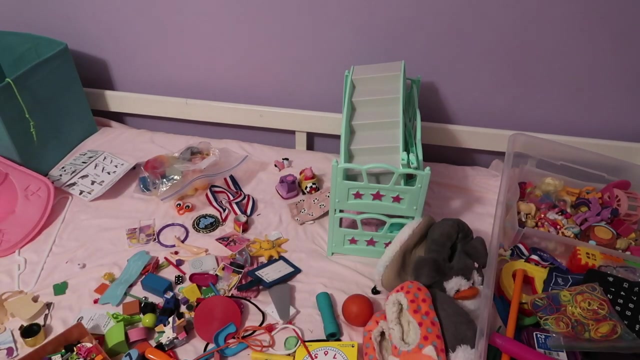 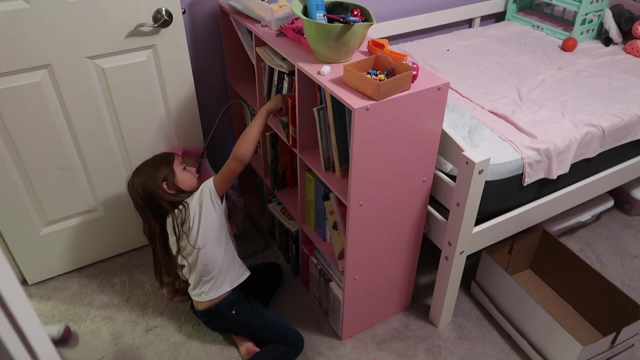 i just i wanna love you a little bit more. i know that it's difficult dealing with emotions, but i want you to know that you'll always be on my mind, even in the hard times. i care about you. how do you move on when everything goes wrong? i'm trying to find a way to get you out my head. 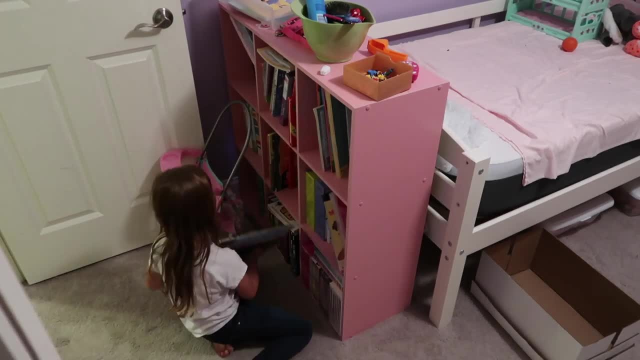 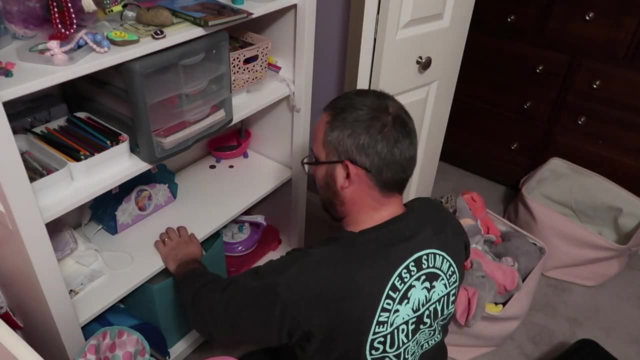 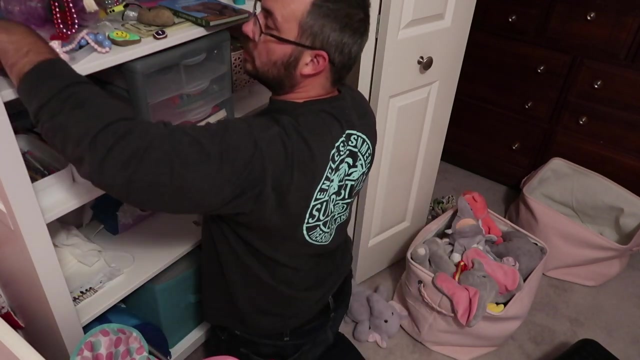 don't. I don't know how to cope with being so broken Girl. I can't forget about what we said. I just wanna love you a little bit more. Don't just walk away from me and close the door, Baby, pull me closer now, before it's over. 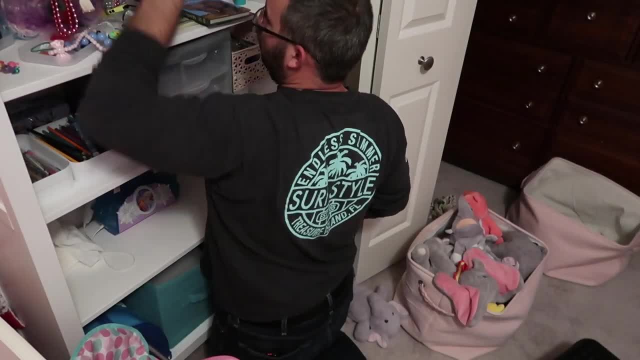 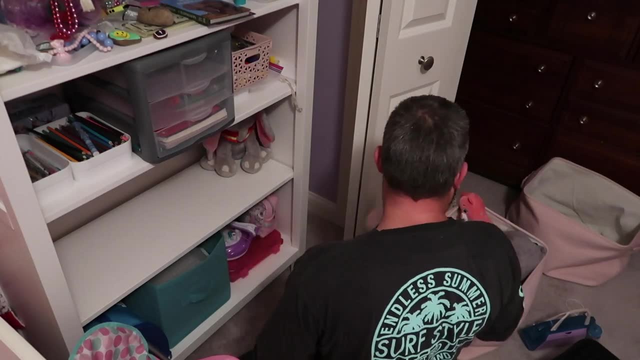 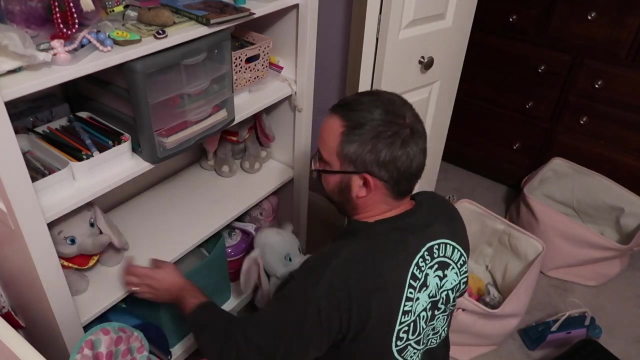 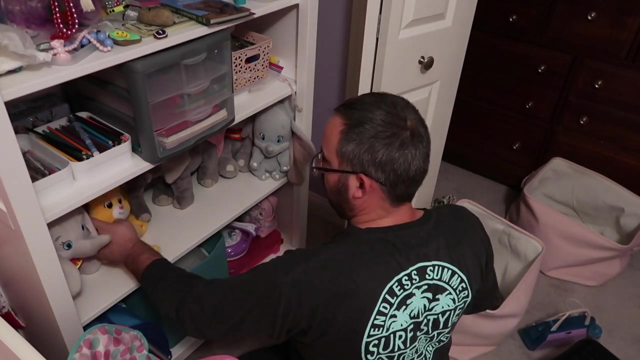 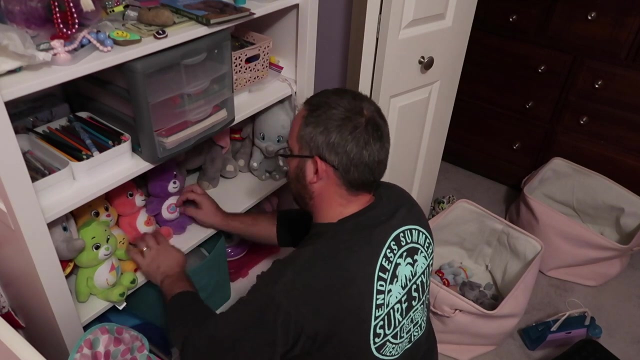 I just wanna love you a little bit more. Love you a little bit more. How do you move on when everything is wrong? I'm trying to find a way to get you out my head. Don't know how to cope with being so broken Girl. I can't forget about what you said. 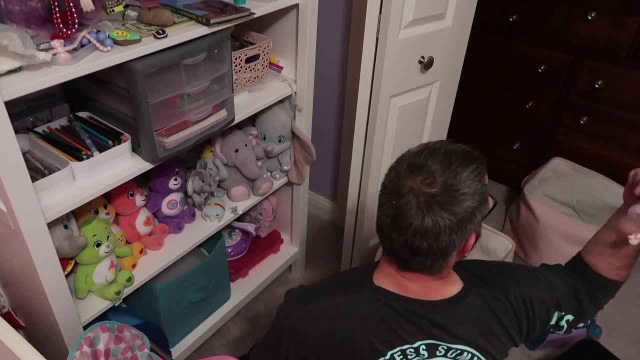 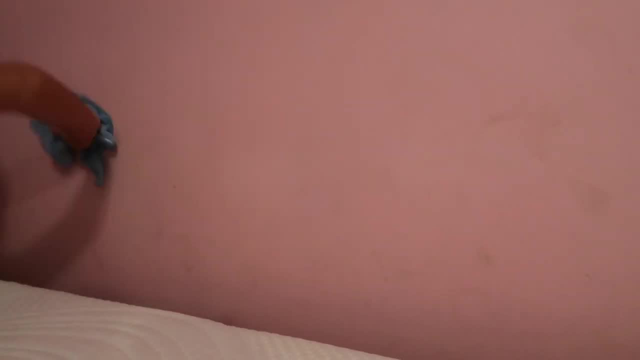 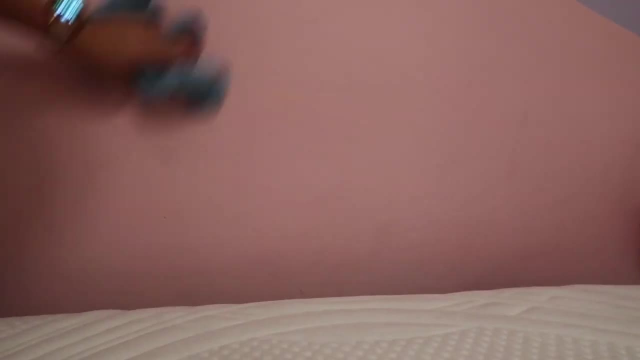 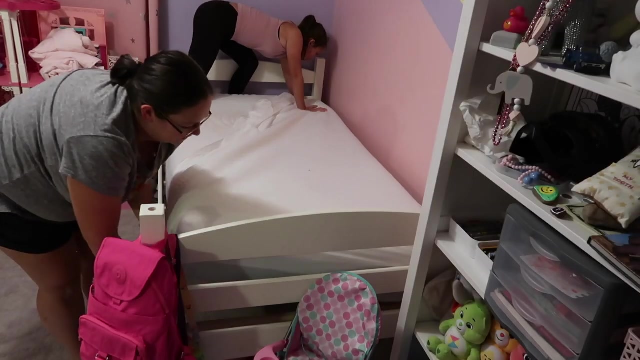 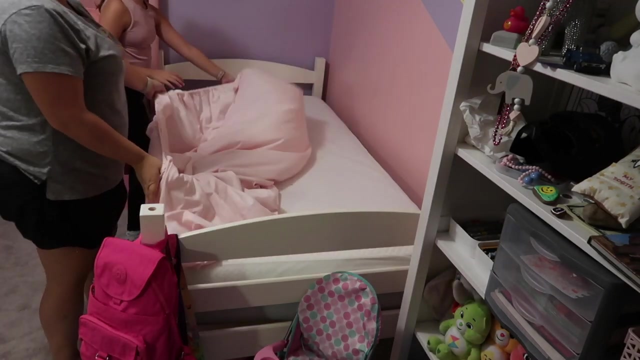 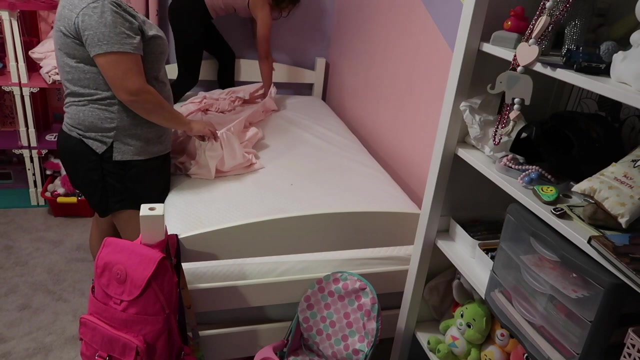 Love you a little bit more, Just a little bit more. Love you a little bit more, Just a little bit more, Just a little bit more. Tonight we're running on the right track. I know we never gonna look back. Oh, I just wanna have a good time. 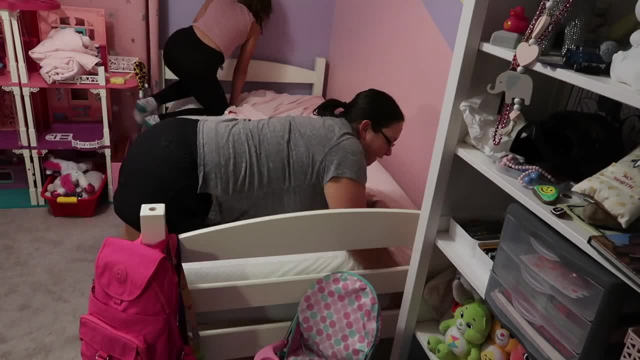 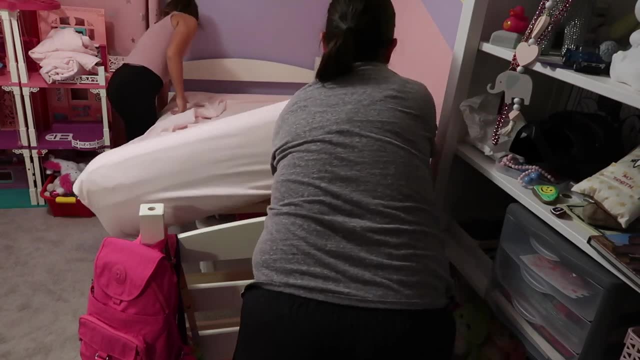 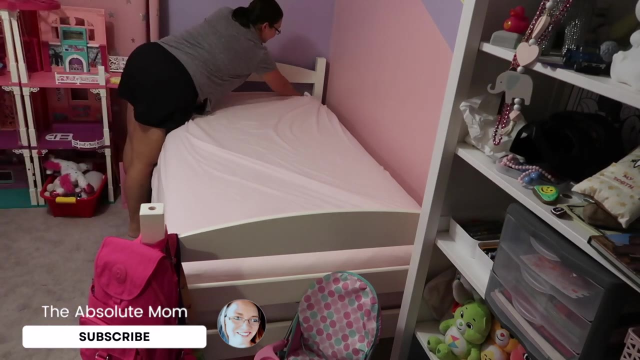 Call me whatever Cause I'm up for anything like that. Oh no, We're gonna have a good time. We don't wanna do no more, So tonight we'll just let go To the beat in the streets. Yeah, we'll freak out Singin' like, Singin' like. 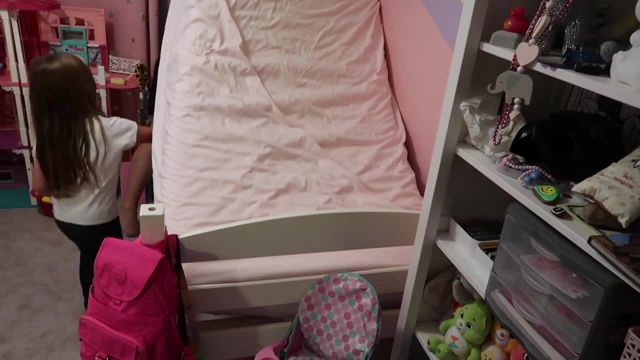 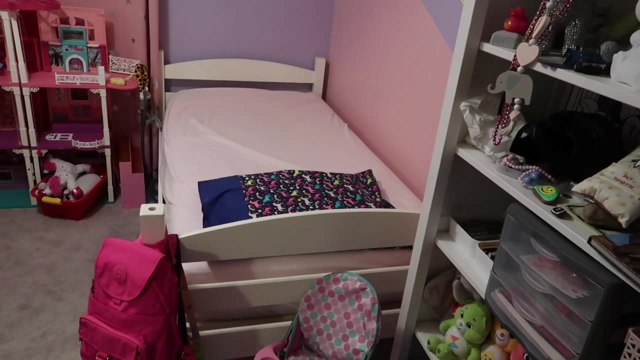 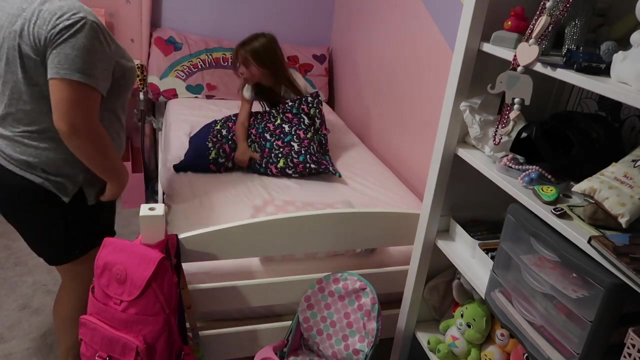 Party like Freakin' out To the beat- Yeah, we'll freak out Singin' like. Singin' like Party like Freakin' out To the beat- Yeah, we'll freak out. Singin' like Freakin' out In doing what you're told. 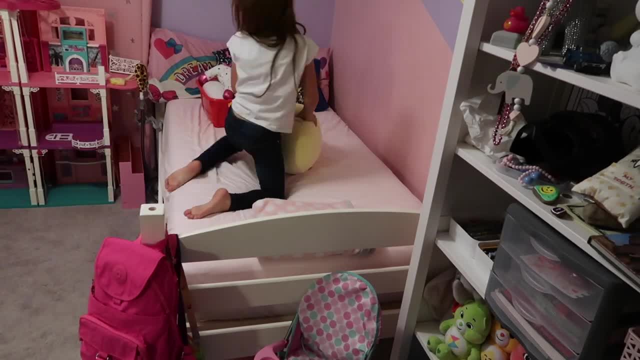 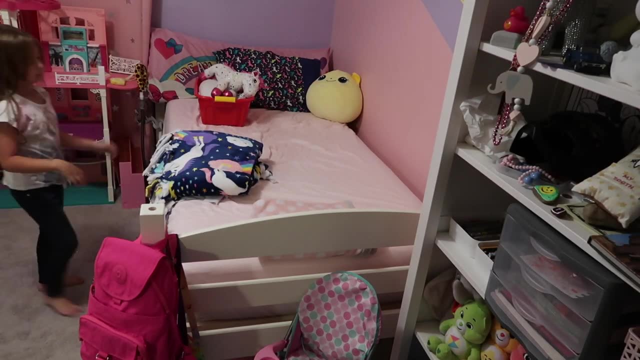 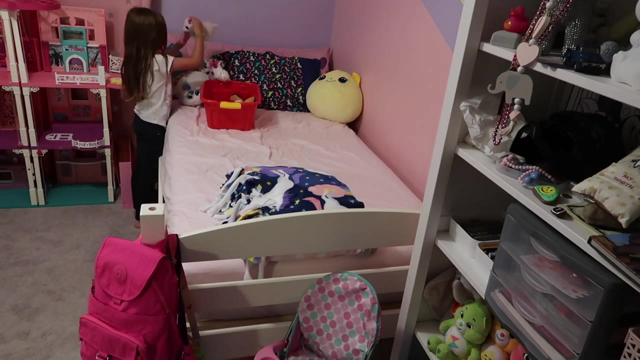 And I don't mind, even though I lose control. Oh, I just wanna have a good time, So call me whenever, Cause tonight, like this, it never gets old. Oh no, We don't wanna do no more, So tonight we just let go To the beat in the streets. 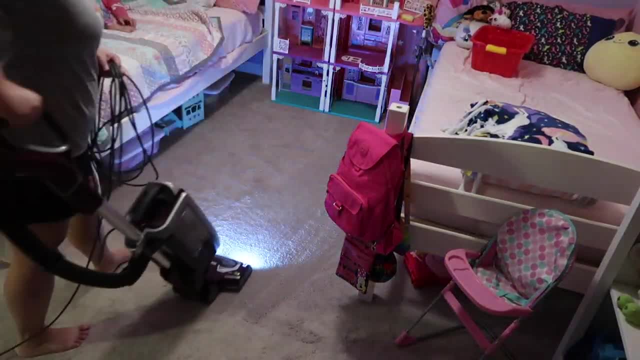 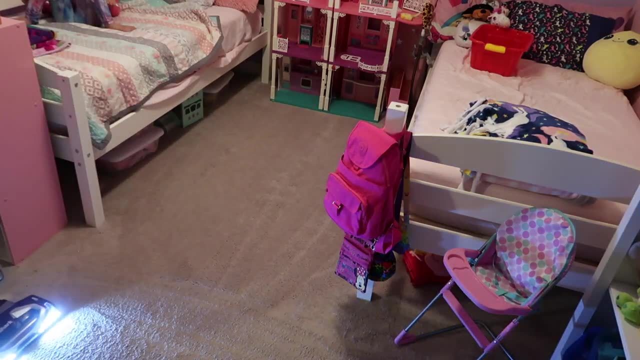 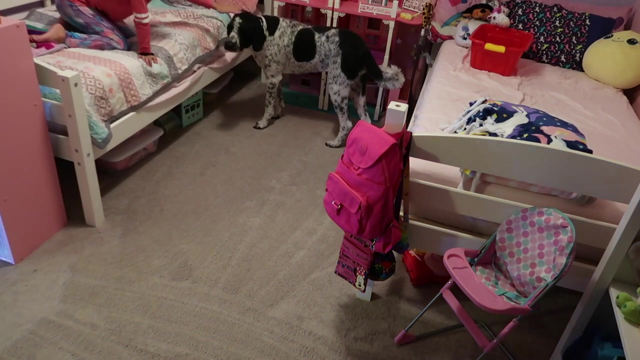 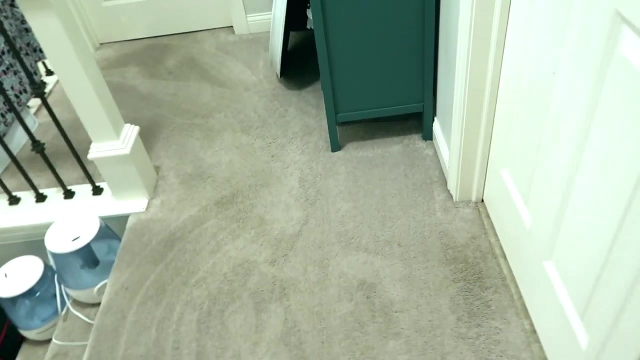 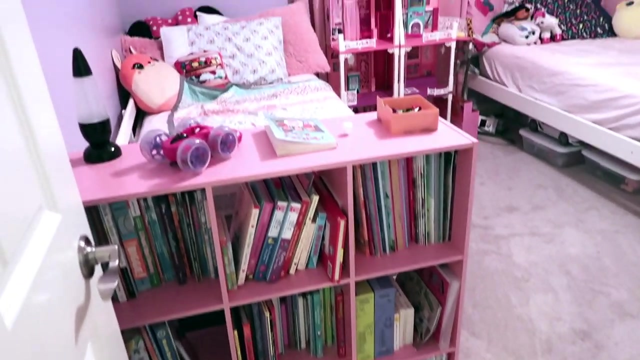 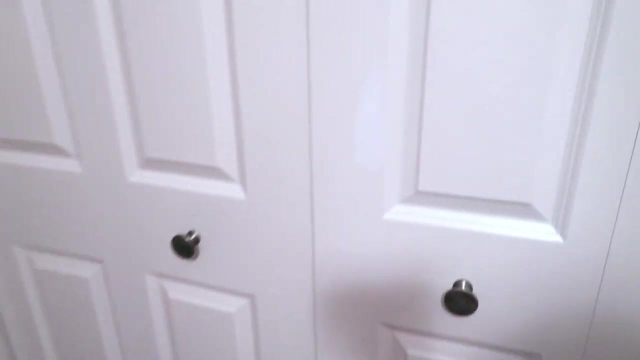 Of this street. I'll sing like Freakin' out. all right, we have a completely clean landing out here, so the stairs are cleaned off. also, all right, the girls room got done. beckett's room is not complete, um, but that's okay. we knew this would take a few days, so closet is cleaned out and organized. we just have some random stuffed.